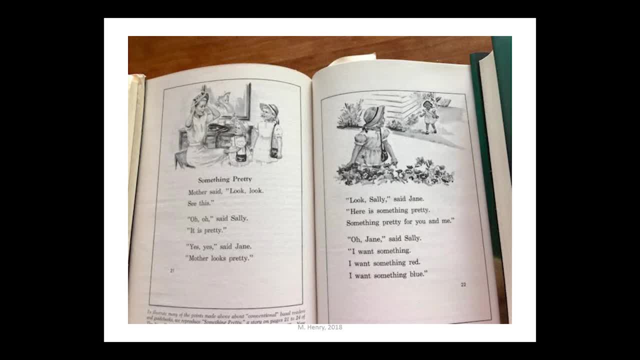 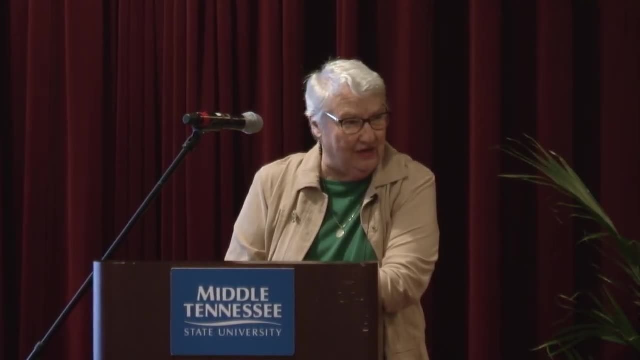 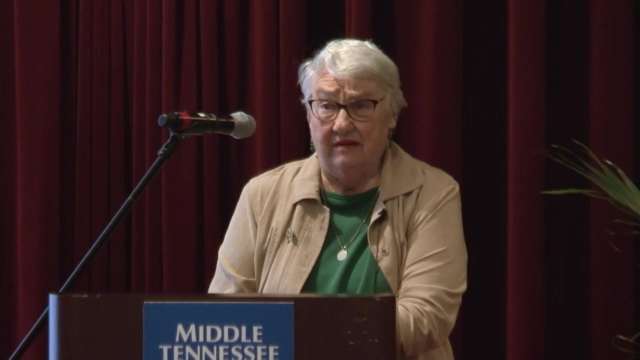 And that's how I learned to read And, fortunately for me, I had wonderful teachers and I was a good memorizer. I mean, I only had to look at a word two or three times and I knew it. I didn't know about a silent E at the end. 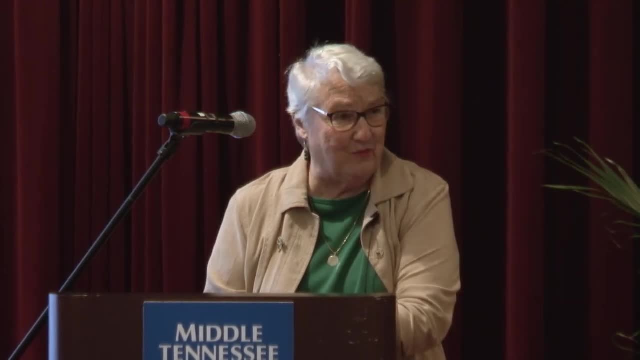 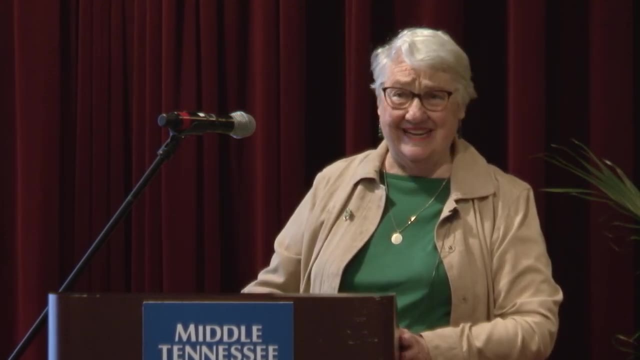 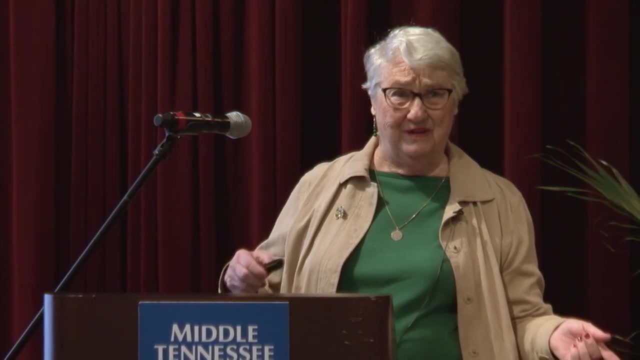 making that A and Jane long and it never had been taught. And then, four and a half years later, my brother came along and he's severely dyslexic And my parents couldn't understand why Peter couldn't read. he wrote his name R-E-T-E-P. 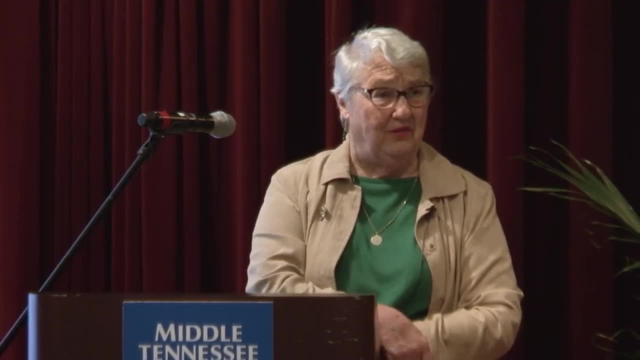 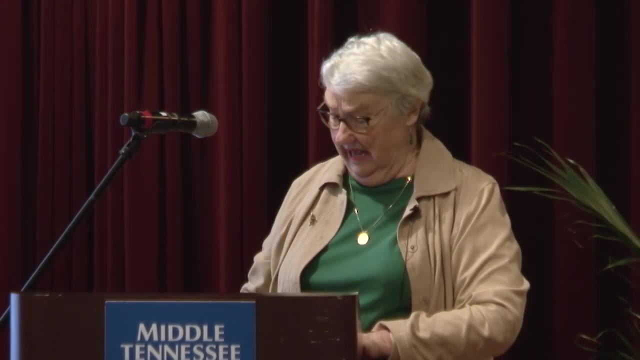 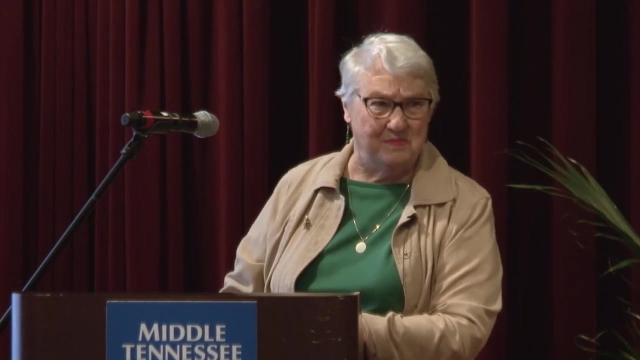 total mirror image until he was in about middle, second grade, And he couldn't memorize any of these. And my parents, the teachers, said: well, Peter's unmotivated, he's lazy, He's not as smart as his sister. 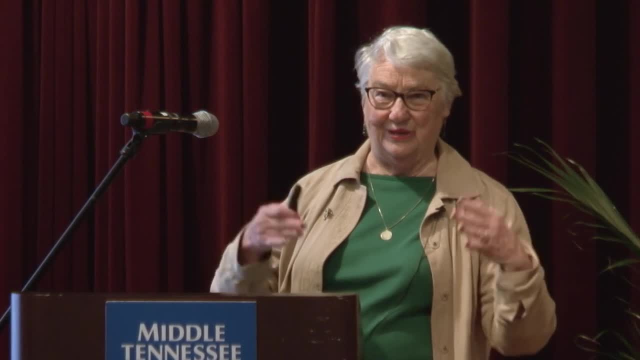 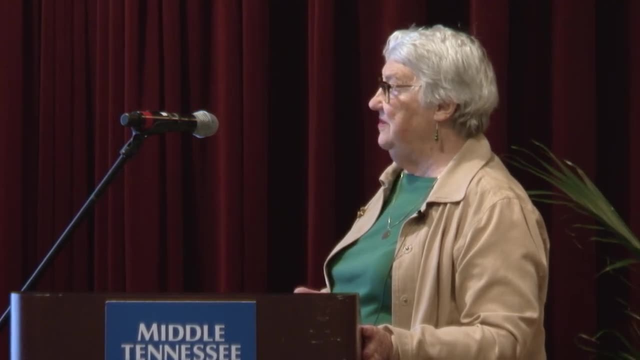 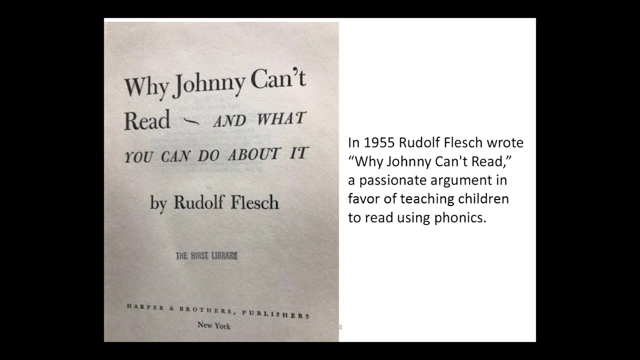 Girls are better in language- All the old myths that we heard. Well, what happened was in 1955, Rudolf Flesch wrote: Why Johnny Can't Read. Some of you probably weren't even born then, But I remember it well. 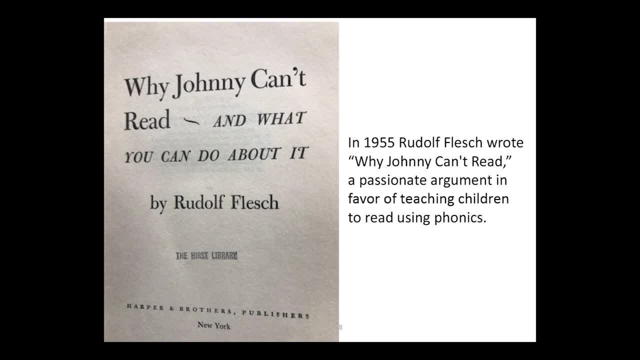 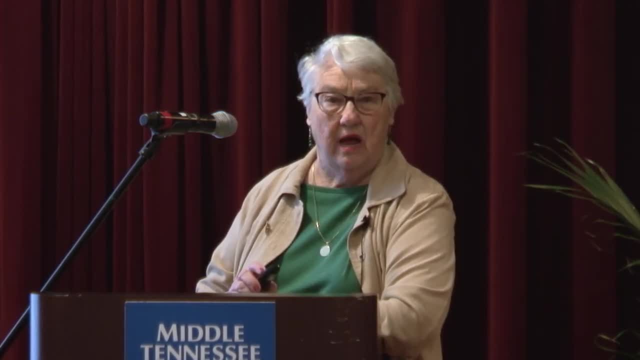 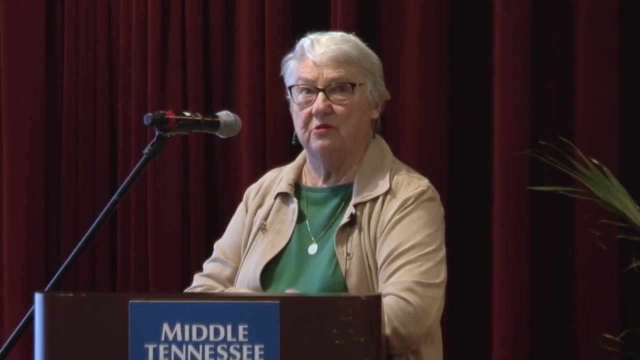 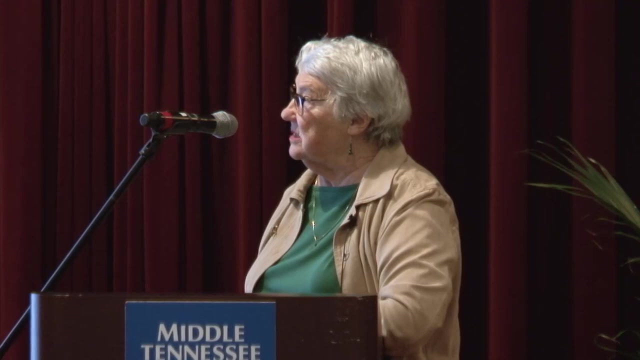 I was in college. I was in college at that time And he wrote this book primarily for parents and teachers, And he gave a very persuasive argument in favor of teaching children to read using phonics. Now Gene Choll in 1967, about 12 years later. 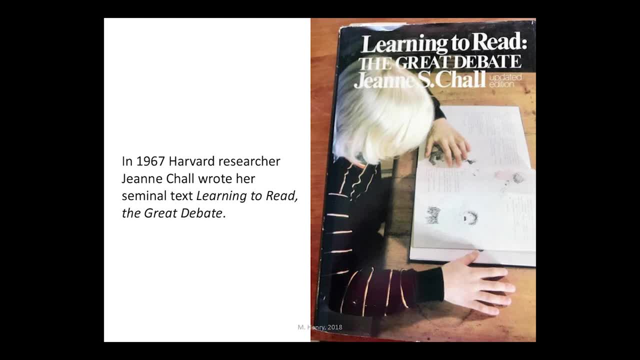 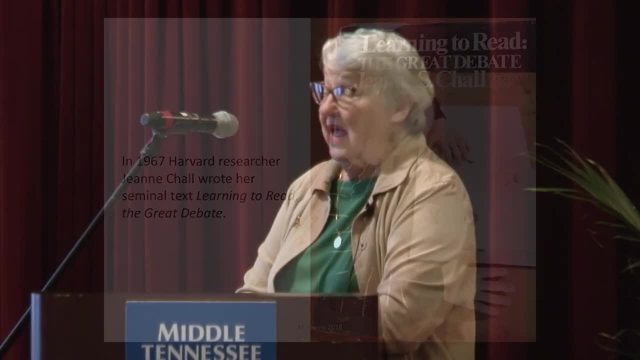 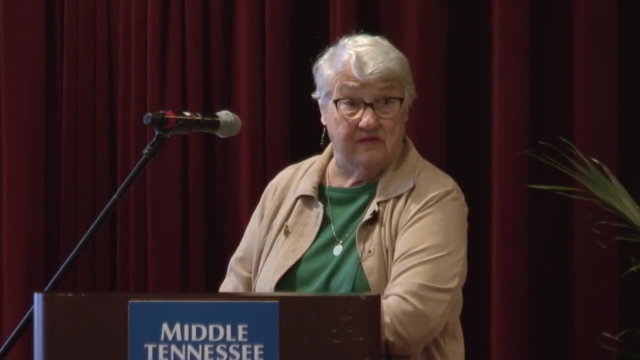 wrote her text Learning to Read The Great Debate- And many of you have probably have that or have seen that- And she again supported phonics Because Dick and Jane was very big at this time And we then went from that whole word learning 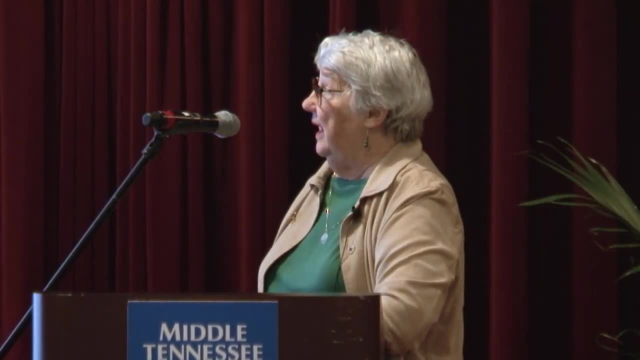 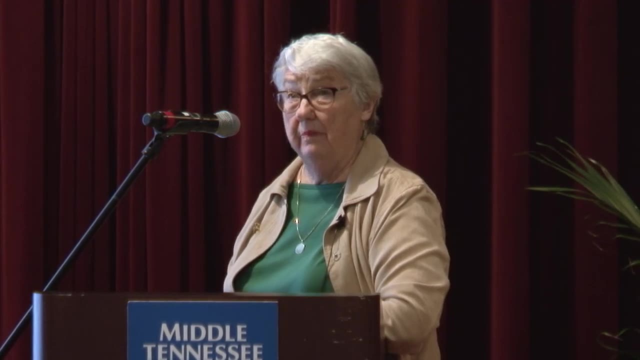 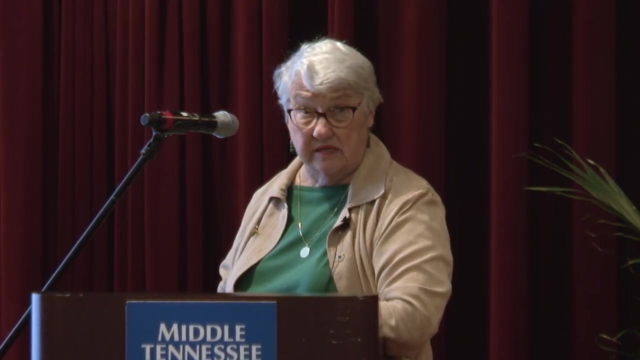 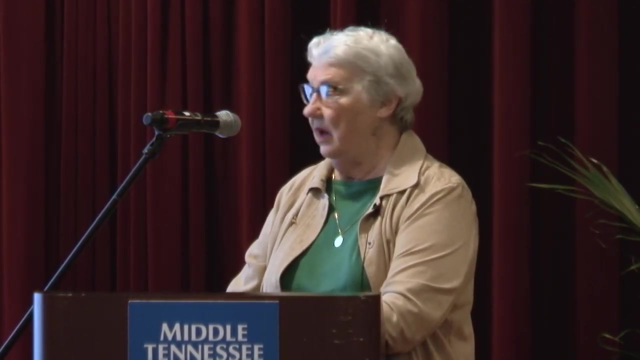 to whole language learning And early research started on reading. The big funding really started in the 1980s, late 70s and 80s And much of this funding came from the National Institutes of Health and Human Services, Children's Health and Human. 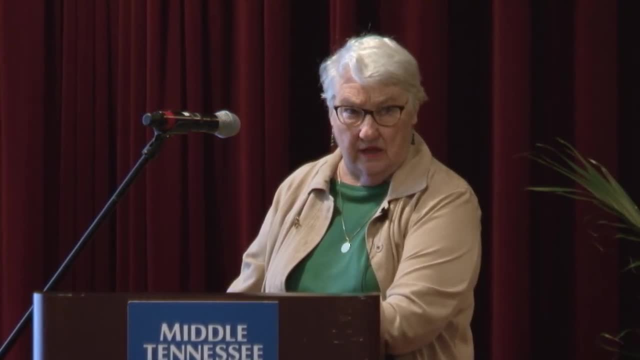 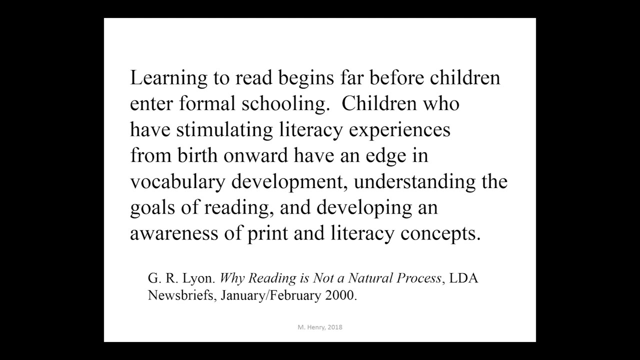 Services. Reed Lyon was the chief psychologist and he said learning to read begins far before children enter formal schooling. Children who have stimulating literacy experiences from birth onward have an edge in vocabulary development, understanding the goals of reading and developing an awareness of print and 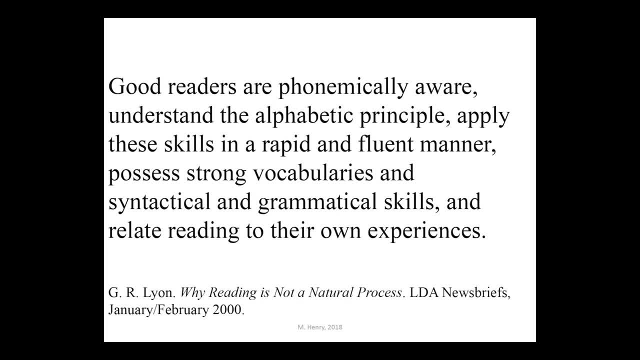 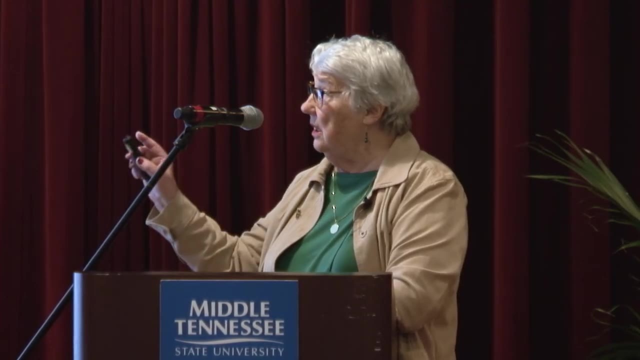 literacy concepts. He also said good readers are phonemically aware, understand the alphabetic principle, apply these skills in a rapid and fluent manner, possess strong vocabularies and syntactical and grammatical skills, and relate reading to their own experiences And his argument, his thoughts on this. 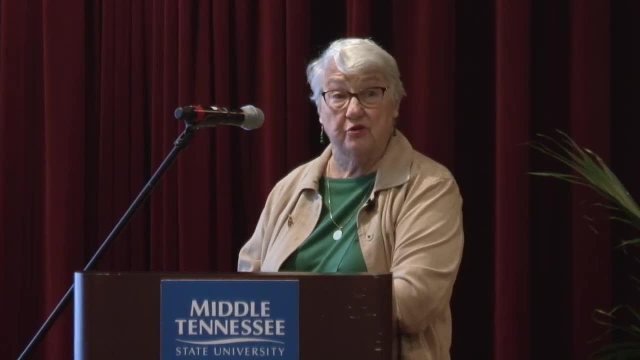 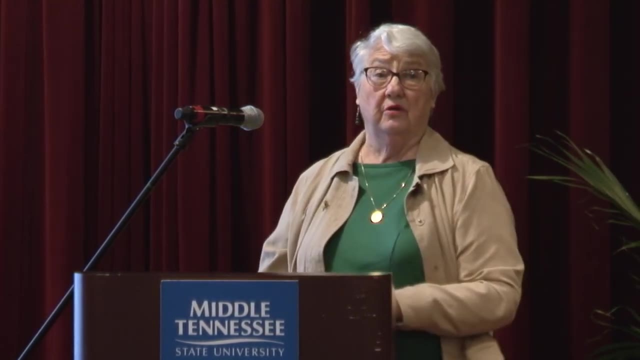 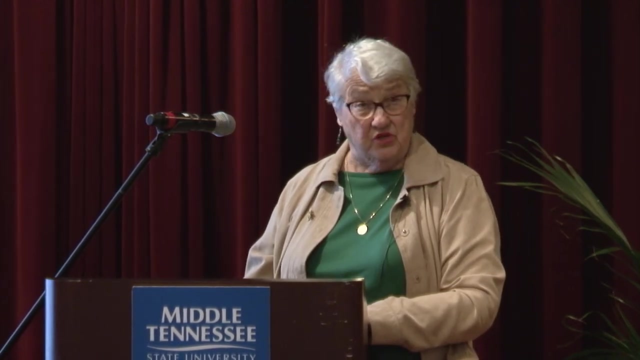 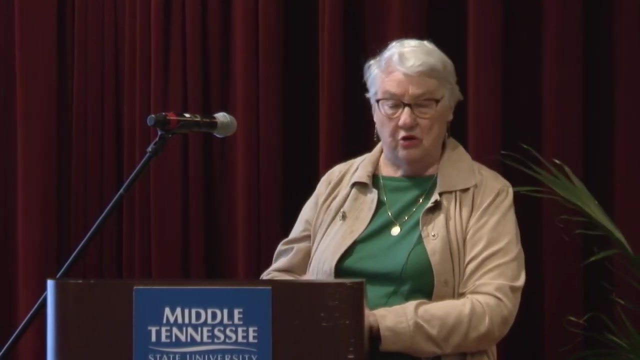 came because of the National Reading Panel that was formed, And this panel reviewed all of this research from NICHD, from the Office of Education, from Office of Special Education, all kind of showing that children needed to be taught to read and that reading does not develop naturally, which, of course, was the whole. 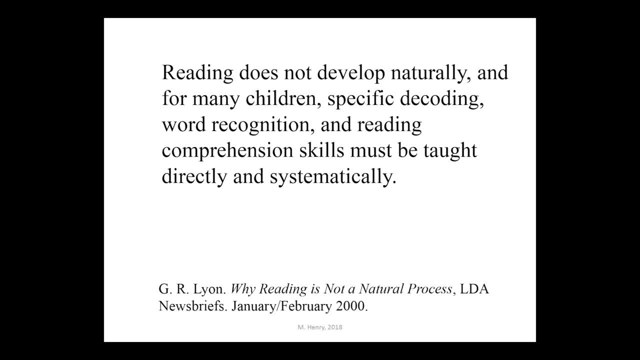 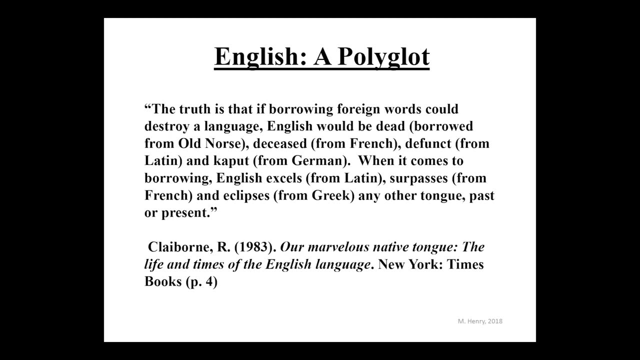 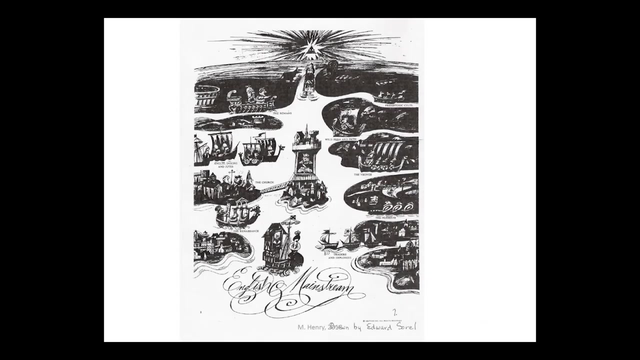 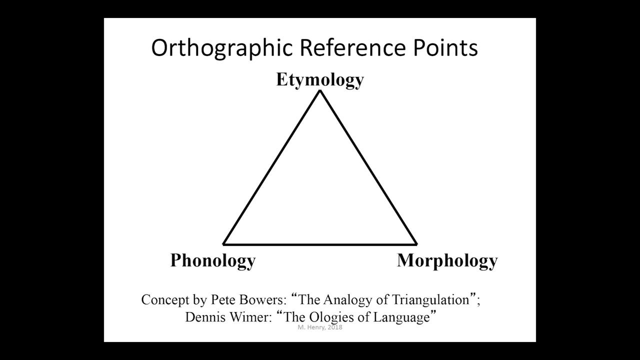 theory, And I would add spelling to this list. You've seen this about English being a polyglot- that favorite quote of mine- And you've seen this Now, this may be new. I was at an IDA meeting. oh, this had to be 20 years ago maybe, And two young men were speaking. 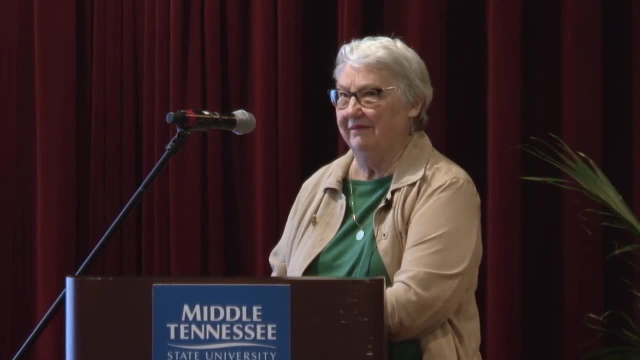 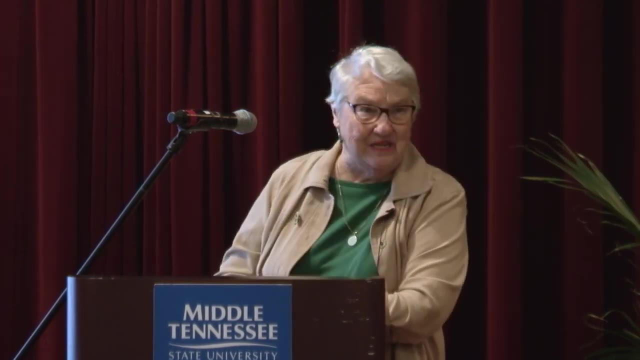 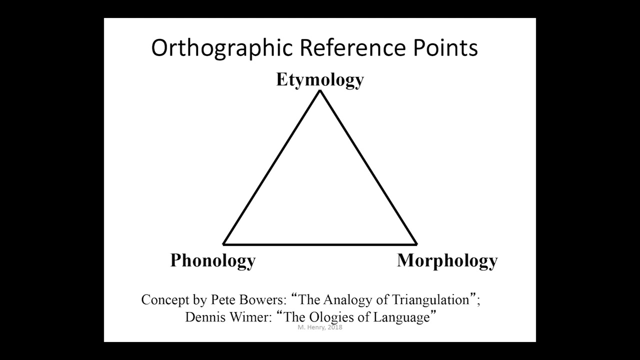 No, it was about. it was probably 2000 or 2001.. And there were two young men that gave very similar tauts. Pete Bower had a talk called the Analogy of Triangulation, And Denniscidos Wilmer Theologies of 좌c. 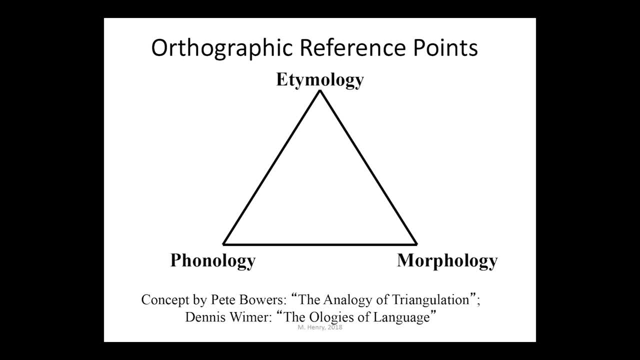 Unequivocally. he said I should have a PowerPoint birthday. So I actually showed up to meet Holda Wiley to talk about this Because I had read ridbles inơ language And what I loved this model. both of them had practically the same model And they. 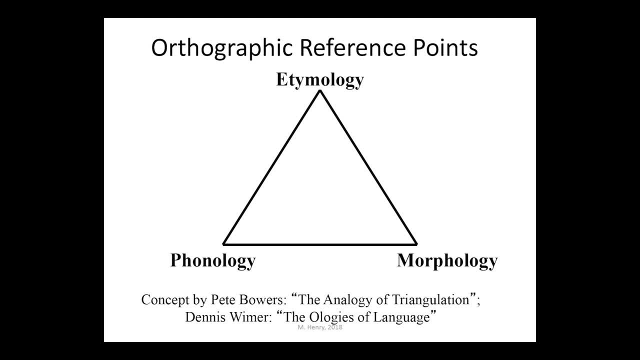 called it orthographic reference points, And what this meant was when we look at our writing system. orthography is any language's writing system And etymology is extremely important. That origin, the history of the word, kind of what we talked about earlier. 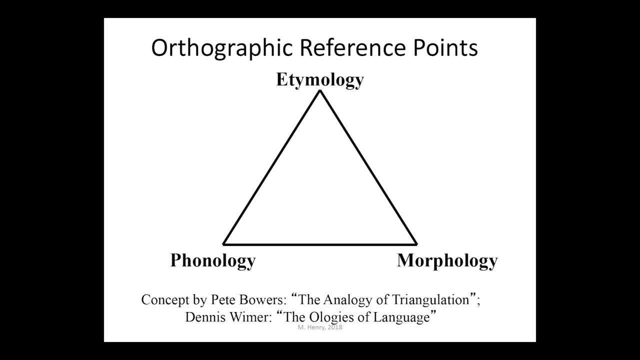 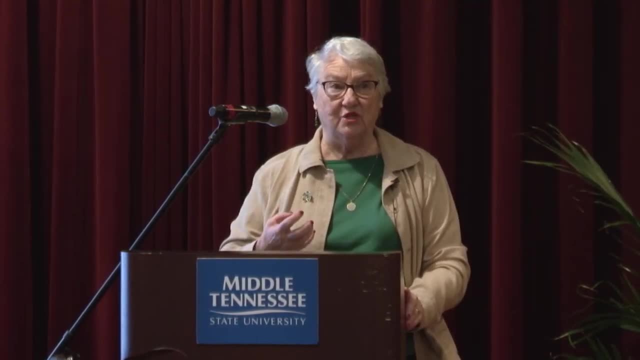 But also very important are phonology- the sound system of the language, and morphology. Morph means form or shape, And morphology is that study of the shape of words. It's the meaning units. A morpheme is a meaning unit within morphology. 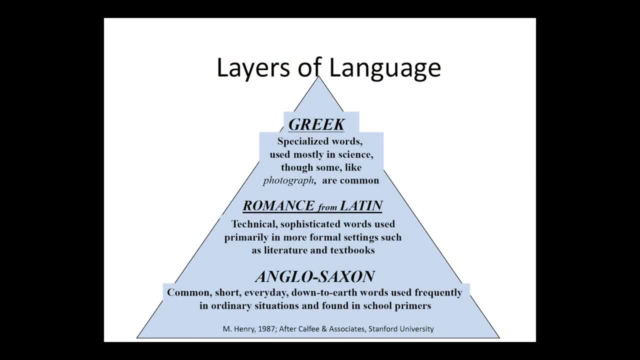 And morphology is a meaning unit within words. Now, you've seen this before. in terms of the etymology, Did it come from Anglo-Saxon, Was it from Old English Or was it from Middle English? Did it come at the time of the Norman conquest? It's a romance in Latin and the 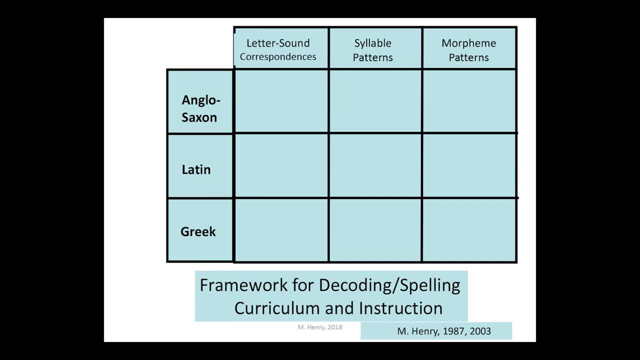 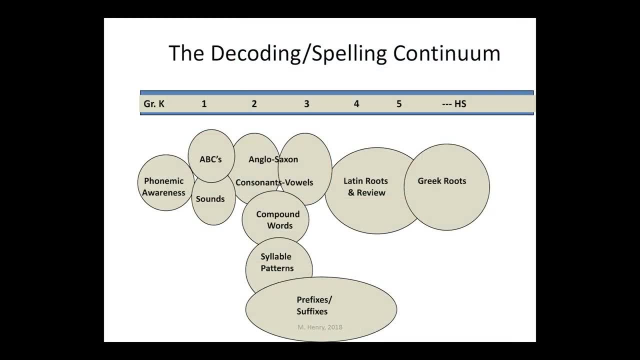 Greek. Now we're going to get much more into detail in this framework as we go through the morning. Here's a better picture. Here's how my thoughts have kind of changed on this. You'll notice that I have the compound words, syllable, patterns, prefixes, suffixes, going way down to second grade. So this 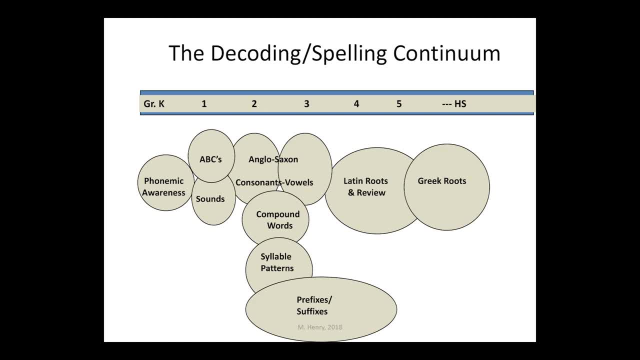 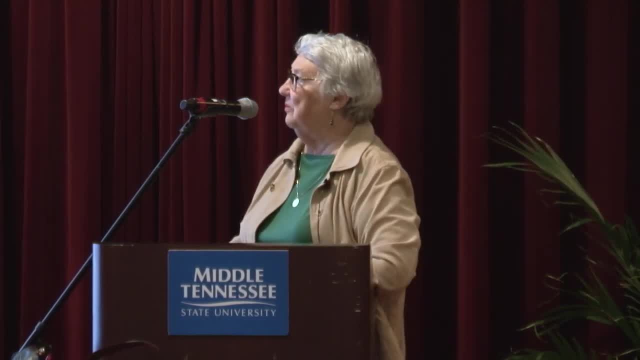 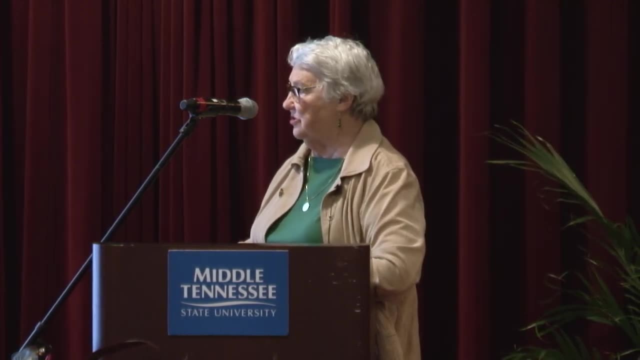 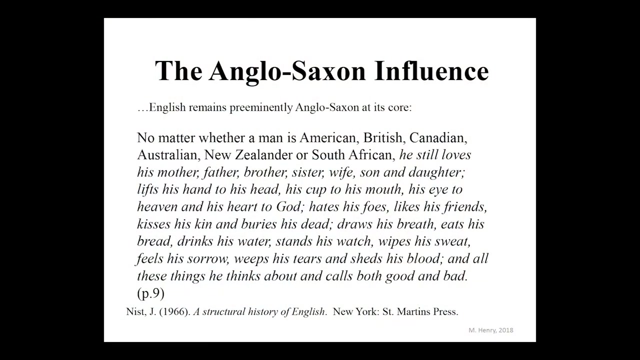 is more where my mindset is now in terms of that continuum. Now let me show you a wonderful. here's another terrific book called A Structural History of English by John Nist, And here's what he said about the Anglo-Saxon. English remains preeminently Anglo-Saxon at its core, No matter whether a man is. 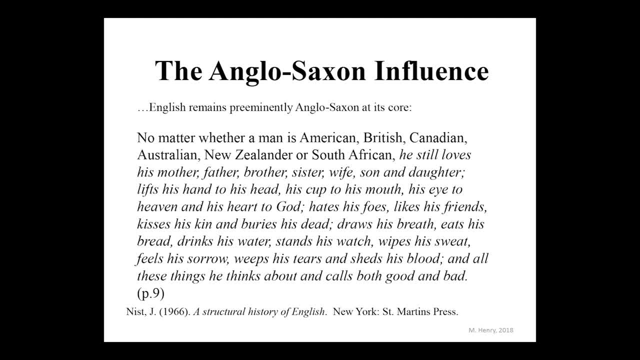 American, British, Canadian, Australian, New Zealander or South African. he still loves his mother, father, brother, sister, wife, son and daughter, lifts his hand to his head, his cup to his mouth, his eye to heaven and his heart to God, Hates his foes, likes his friends, kisses his 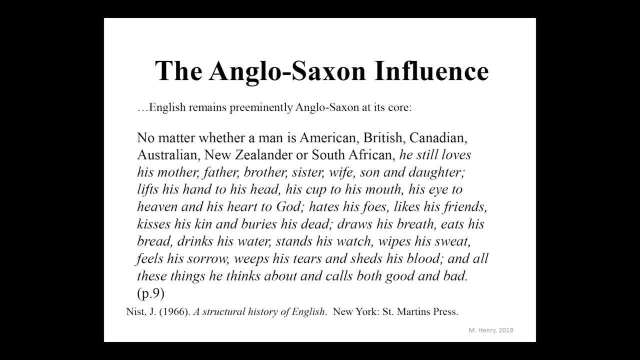 kin and buries his dead, Draws his breath, eats his bread, drinks his water, stands his watch, wipes his sweat, feels his sorrow, weeps his tears and sheds his blood, And all these things he thinks about and calls both good and bad. Now look at those words. Are they difficult? 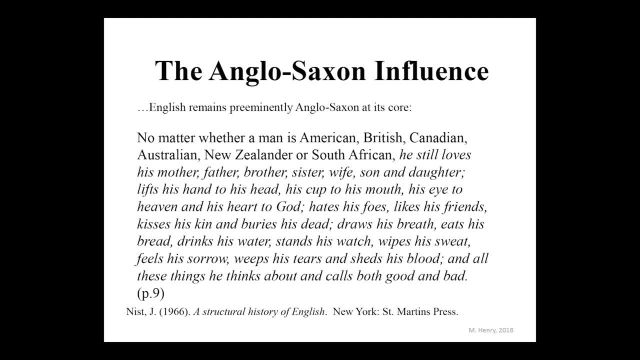 Are they sophisticated? No, they're the common everyday words we all use. But look at the nature of some of those words. Look at- I don't say he still loaves- his mother, father, brother, son and I don't know. 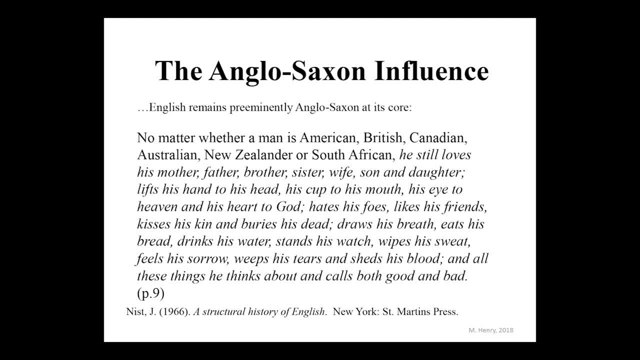 how we'd pronounce that. Look at heart, friends, berries, Watch, in a way, Blood, All irregular words. They don't fit exactly into what we think of as that phonetic scheme, the phonics that we know. So this is why I say this is sometimes the most. 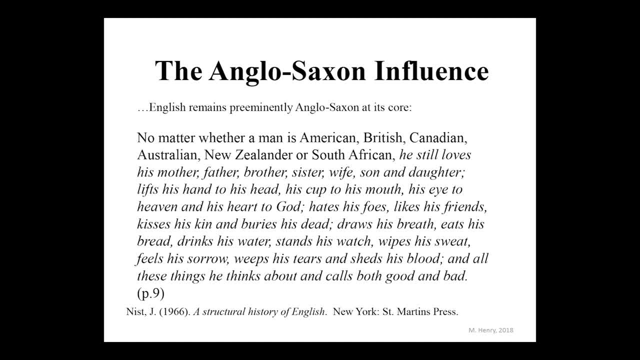 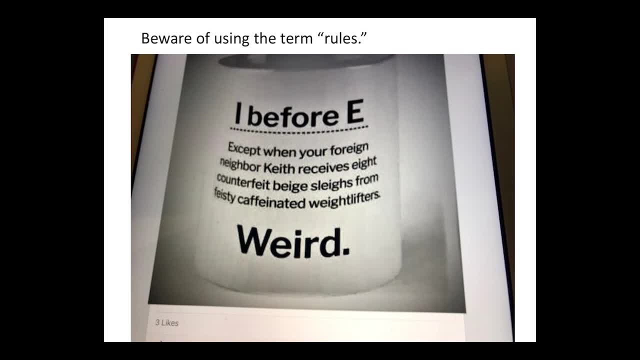 difficult layer for children to learn. I love this. This was on a coffee cup I saw the other day, So I'm very aware I've changed in my own teaching. I tutor occasionally but not on a regular basis. But I rarely anymore use the term. 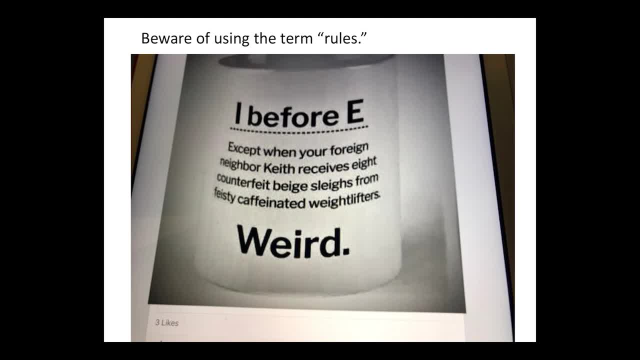 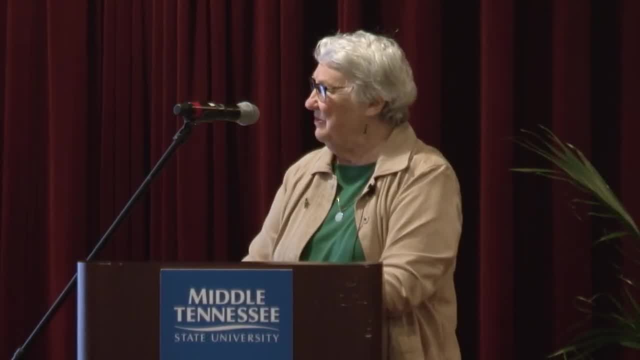 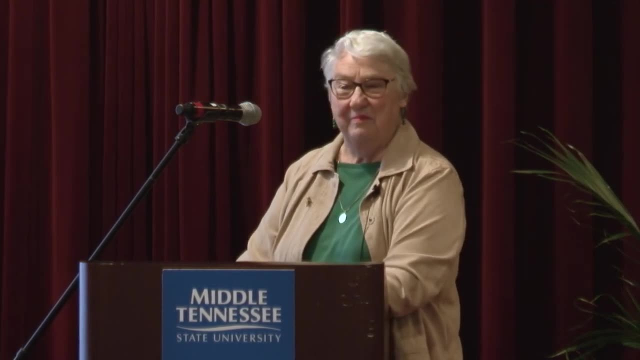 rule, Because to me a rule is something that really stands out, And I think that's a really difficult thing to understand most of the time. And when we think of this, there are all sorts of funny sentences like this. My brother, the severe dyslexic, remembers one from his ninth grade. 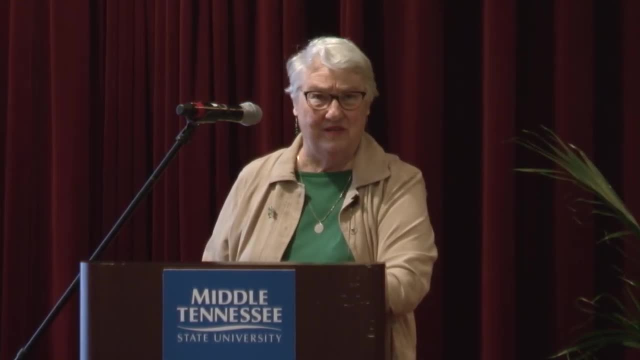 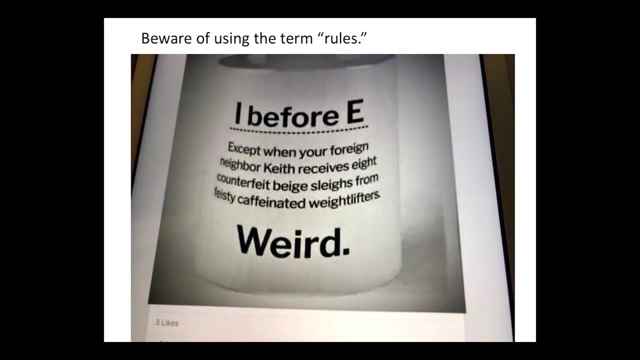 English teacher who got so upset with his spelling that she gave him this crazy sentence with a lot of exception words. He remembers it, He can just spot it. I don't remember it. So I always say kind of beware of the rules. Now, this is a nice little chart that. 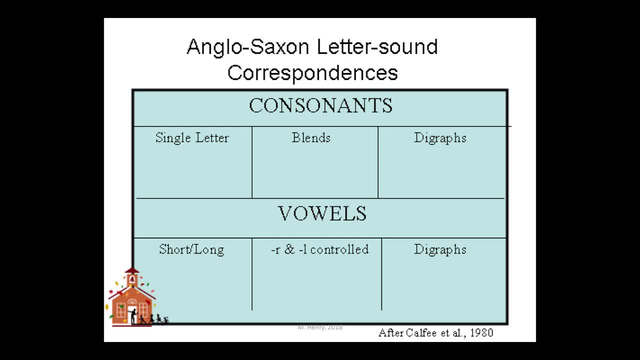 my primary advisor at Stanford, Bob Kelphy, had developed when he was working at the University of Wisconsin with Dick Vanesky, who's a linguist, who wasn't a linguist. What they did was kind of divide the core of the language, And I think that's what they did, And I think that's what they did. 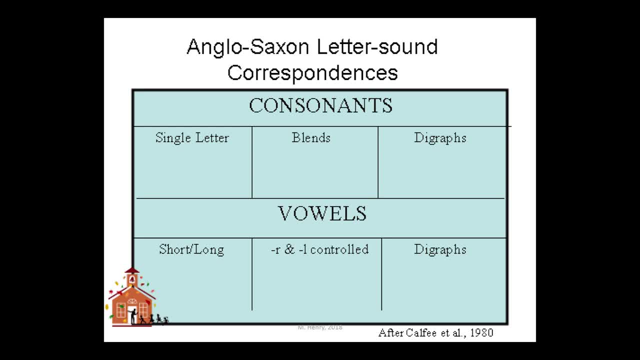 So I think you can see that we have letters into consonants and vowels. We have our single letter consonants, We have our consonant blends And we have our consonant digraphs, as well as those trigraphs, graphs like TCH, And then we have our short and long vowels, our R and L controlled. 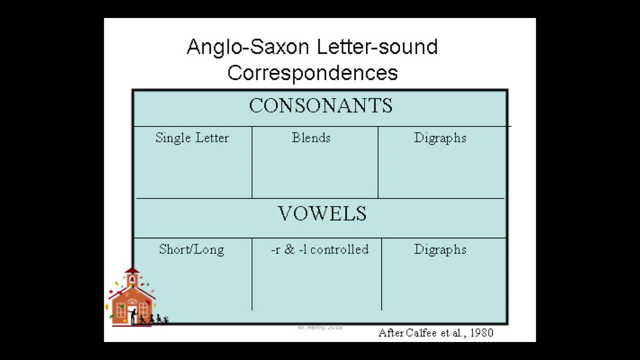 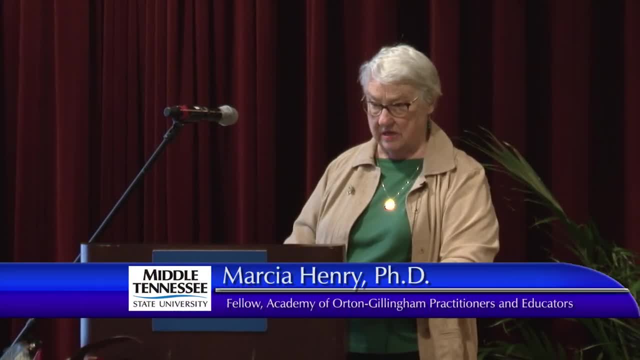 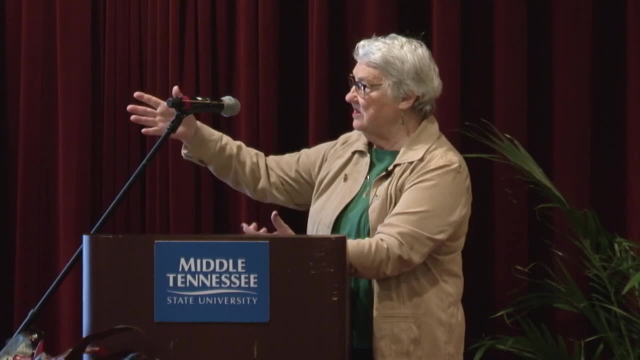 vowels and our vowel digraphs And almost all of those patterns that we want kids to know can go on this chart, And when I was teaching at San Jose State, I'd always recommend that they use a to my pre-service teachers that they have this kind of a chart in their room. 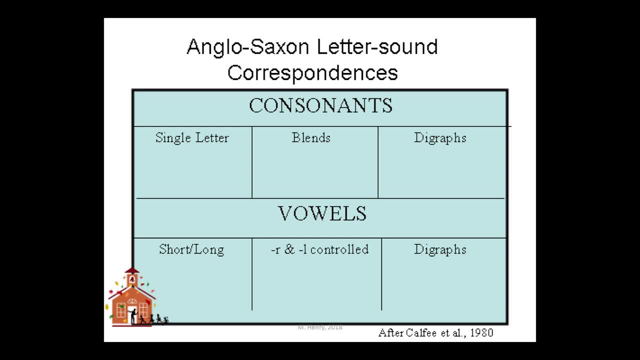 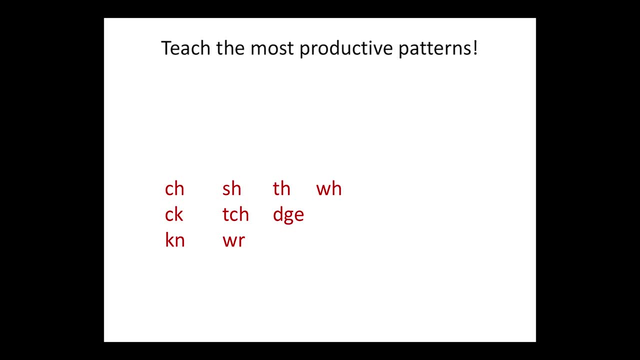 and as they presented the various patterns, they would place them here. Now, one of the things that I really emphasized with my teachers is teach the most productive patterns. So the vowel digraphs, some of those silent letters, obviously the main vowels- 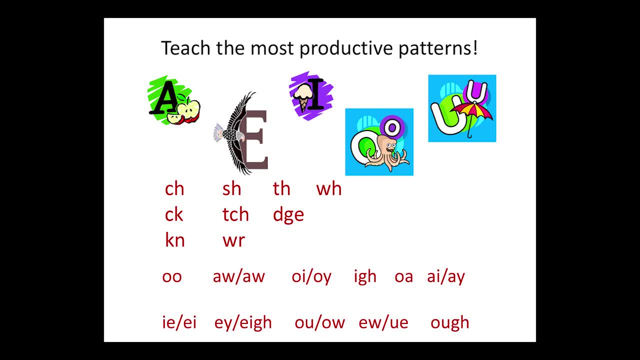 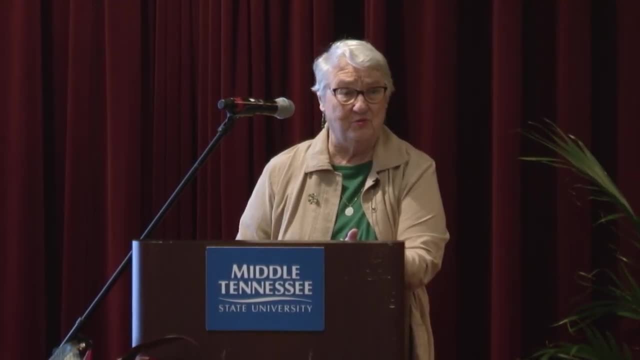 obviously the vowel digraphs and all the other consonants. I don't really I don't like to teach that there are eight ways to spell A, because over 96% of them of the words with A are spelled with an A. 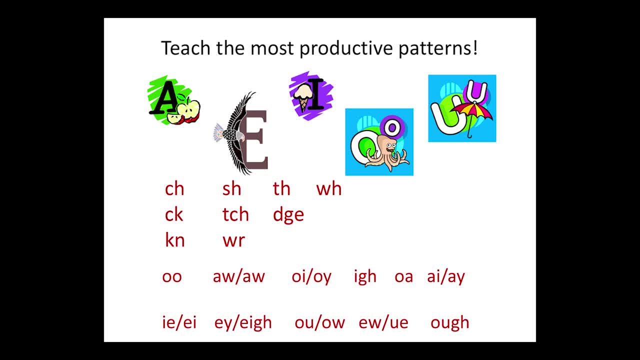 an open syllable, A, like in baby or vacation, an A consonant E, an AI or an AY, which usually is at the end. So those are real important to teach Now, whether you want to teach E-I-G-H. 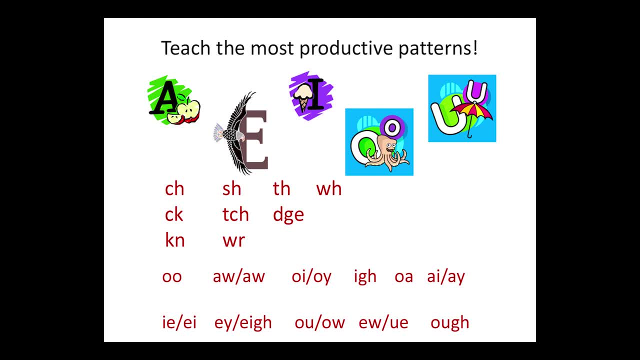 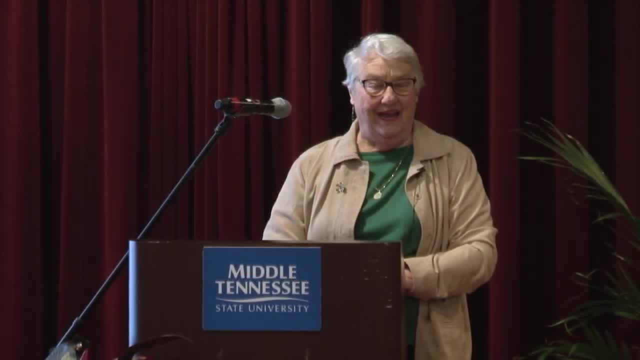 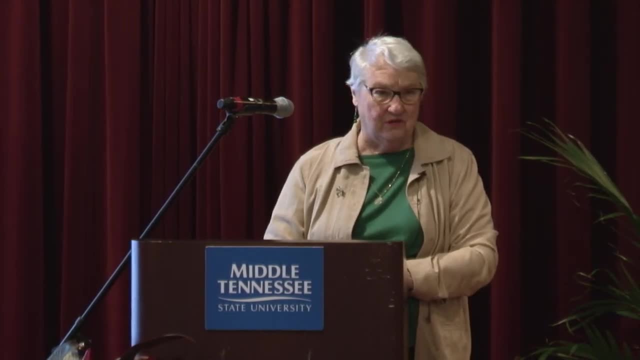 that's fine E-I, But some systems? I was saying this once at a meeting in New York and I said: don't teach E-A as being A. I said it happens in three words in the English language, three common words. 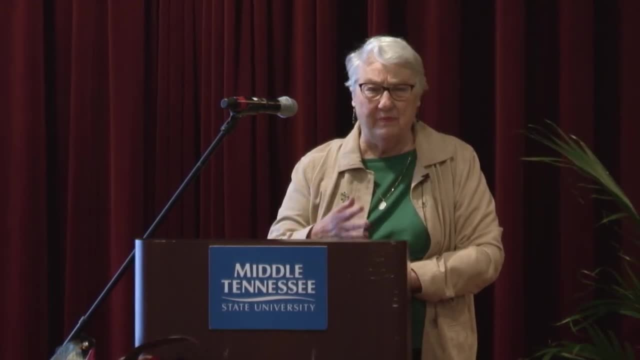 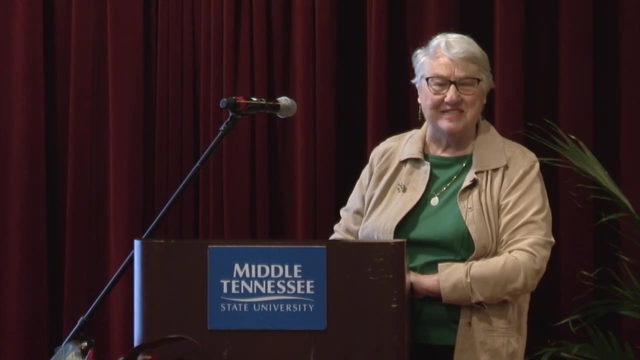 Great stake and break. You know, those are better learned as memory words. And one woman raised her hand and she said: well, what about Shea Stadium, which is S-H-E-A? And I said, well, proper names don't count. 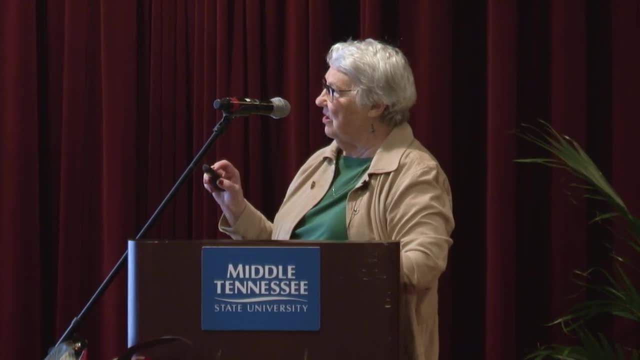 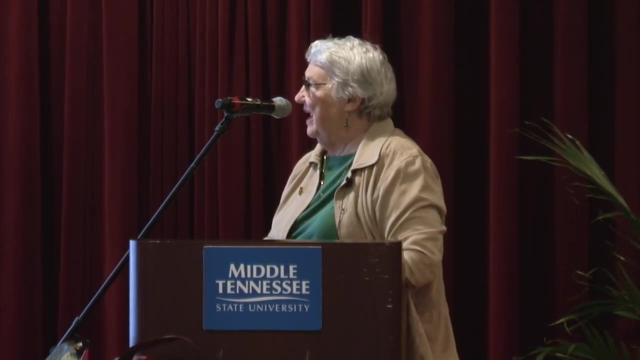 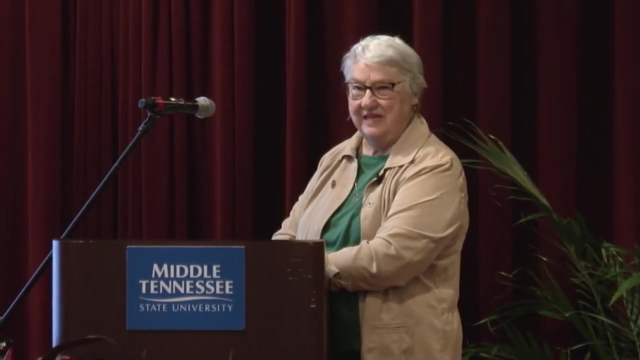 But so. so that's just one of my thoughts. You know, if you have a limited time, teach the very productive patterns. Now, this is a conference on spelling, And here's Dolly. Spelling would be easier if you could buy vowels. 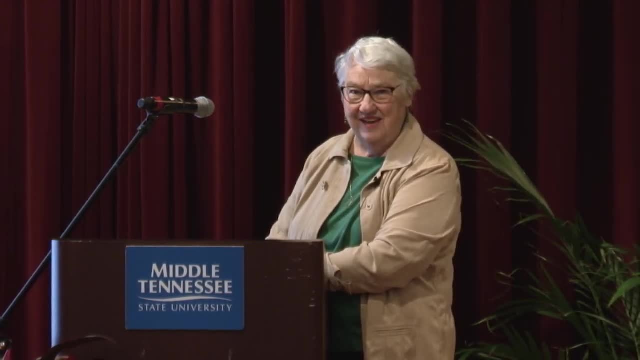 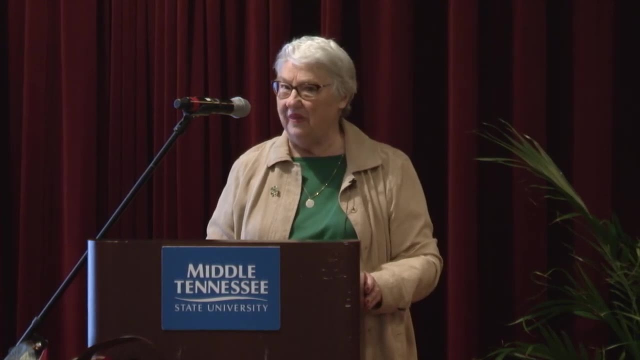 And isn't that the truth? This is the area. it's mainly the vowel sounds that our kids have trouble spelling. Most of them do pretty well with. you know the consonants, But the vowels are what are so difficult for our kids. 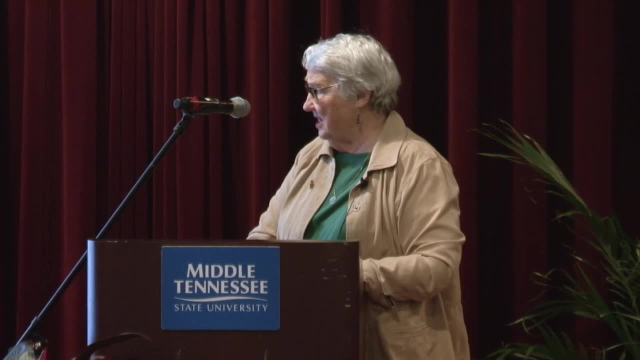 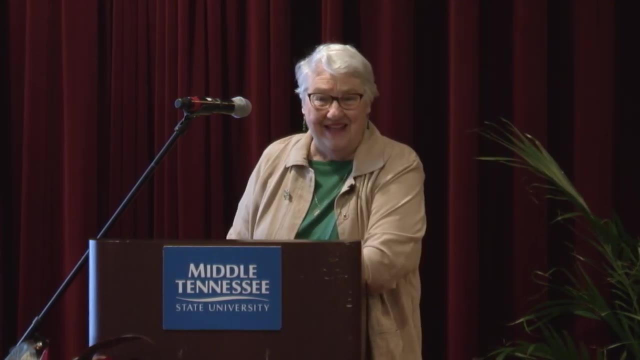 And Dennis? here's Dennis. They're spelling things around me and I haven't been able to break the code yet. And that's what our kids have to do, isn't it? They have to learn the code. The alphabetic code is: 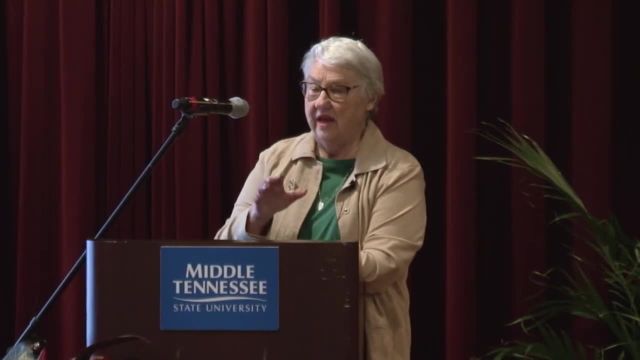 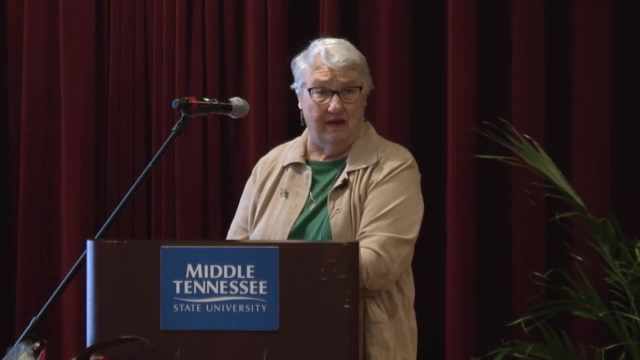 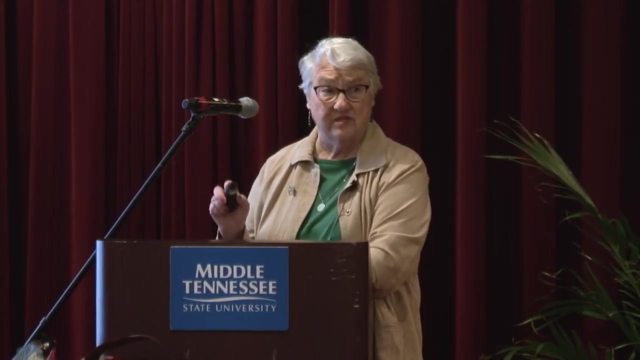 means that letters have corresponding sounds, And that's what I'm trying to do, And that's what we, when we're teaching phonics. that's what we mean: We're connecting those graphemes or letters with the phonemes. 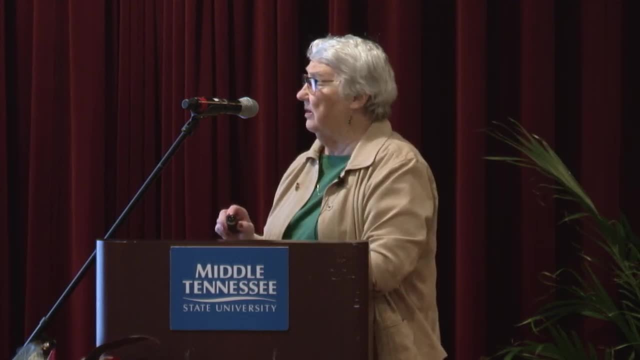 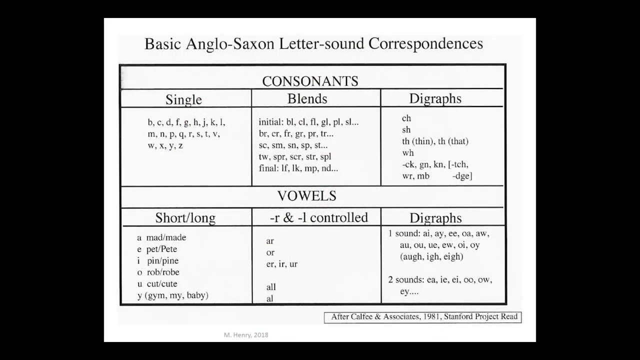 or sounds. So those are terms that that are important to to know. Now here's something just kind of filled out: this basic two-by-three matrix. Obviously it's alphabetically here, We don't teach alphabetically, And so 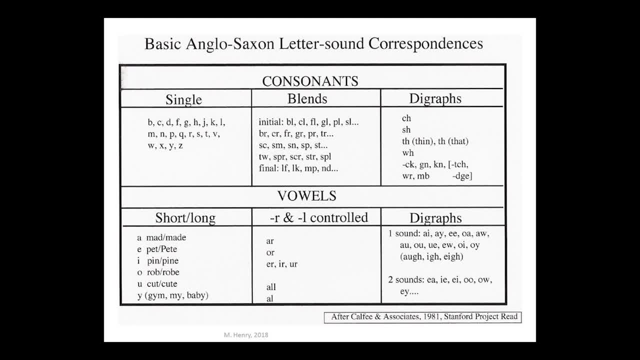 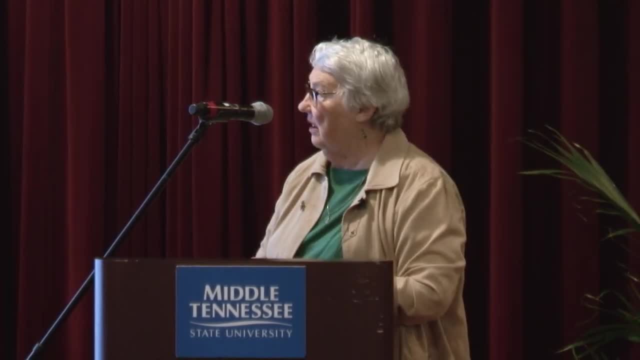 we don't teach B and D at the same time, because chances are many of our kids are going to reverse those. There are lots of books that give you, you know, an appropriate sequence and, for teaching these, One of the things you want to think about. 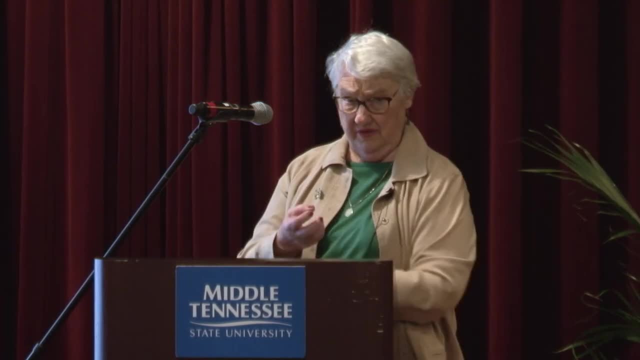 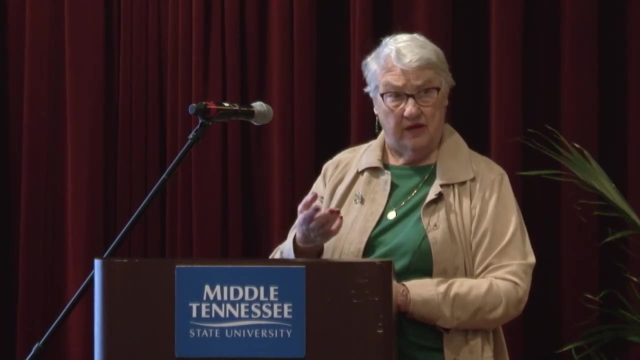 is that this is all cumulative. You start with a handful of of consonants and maybe one short vowel. Then add the other short vowels as you're adding more consonants. Then get into consonant blends to consonant digraphs. 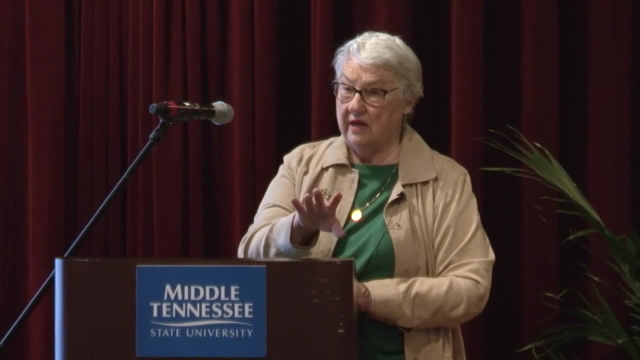 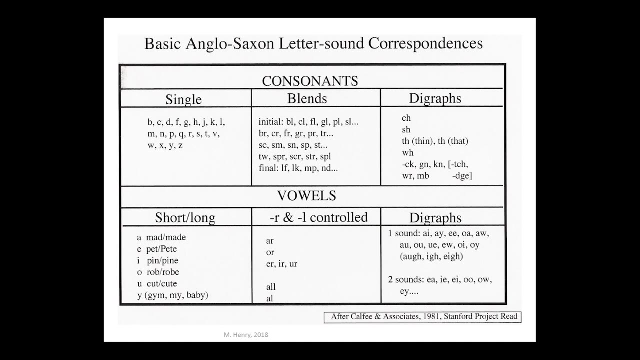 at the same time presenting some of the vowel digraphs, often called vowel teams, So, but these are the types of of patterns that we want kids to know automatically: As they see the letter, they know what the corresponding sound is. 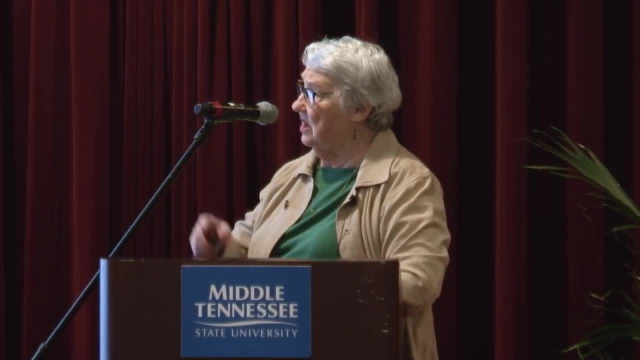 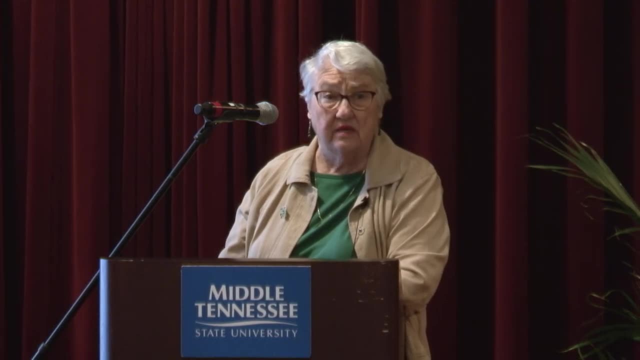 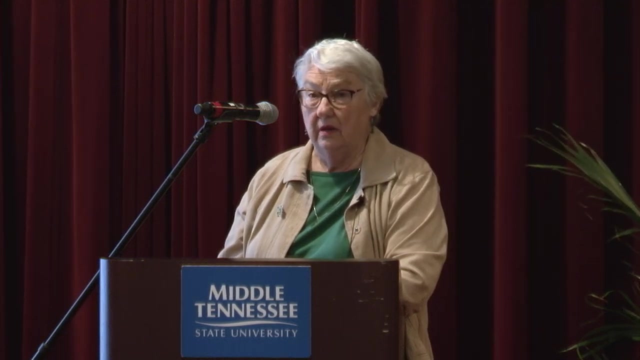 Most of the consonants, single letter consonants, have only one sound. A few have two, Like C being K or S, And the S sounds S, sometimes the- I should say the Z sound, the Z sound. 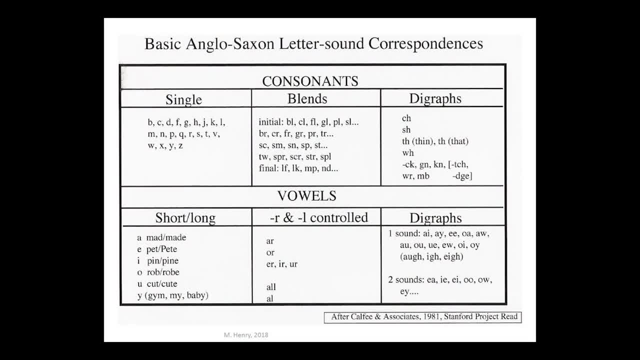 sometimes is spelled with an S, So some of these have more than one sound. So I want to take kids through these basic phonics and I'm not going to say much more about that. What I want to do kind of think of that. 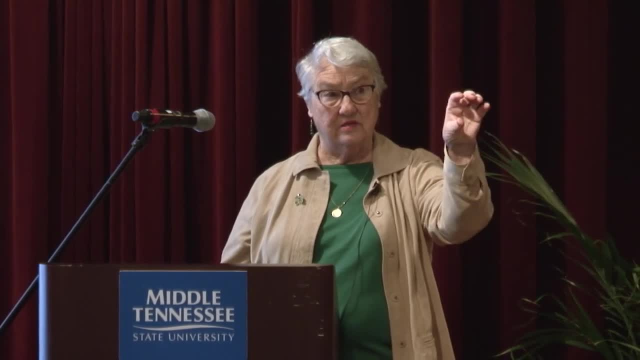 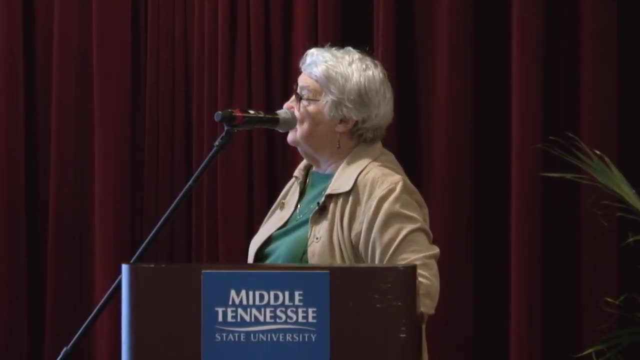 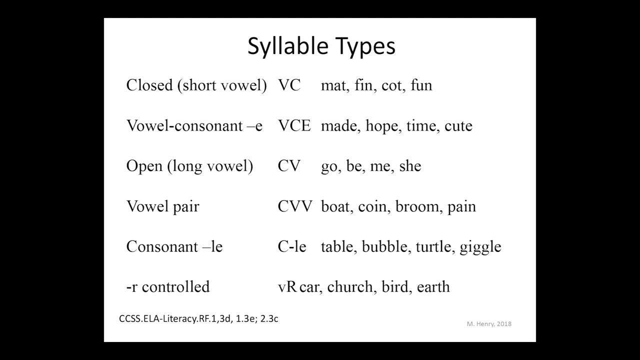 three by three, matrix with Anglo-Saxon letter, sound correspondences, syllable patterns and morpheme patterns. Now we'll talk a bit about syllables. We want kids to be aware of the six syllable types. We want kids to be aware. 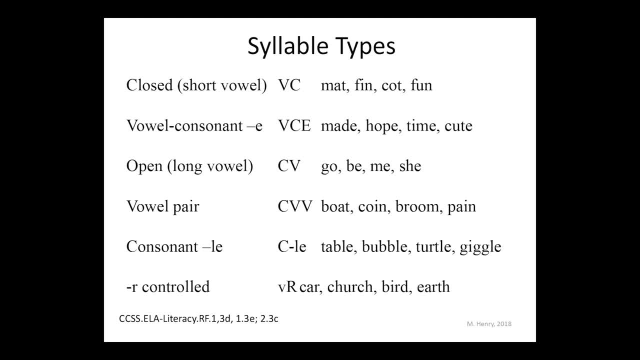 that when I have one vowel followed by a consonant or two consonants, I'm going to have a short vowel, A closed syllable it's called. The vowel is closed off by the consonant, We have our vowel-consonant. 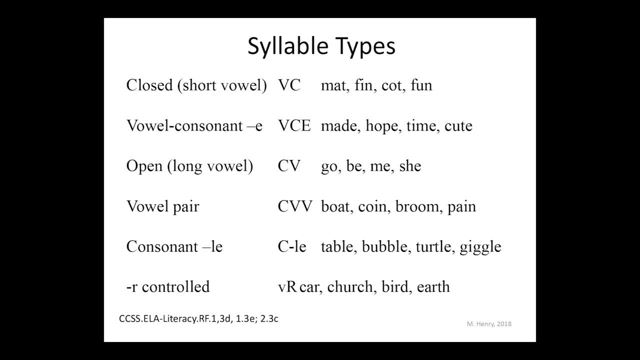 E syllables where the final E. if I just had M-A-D, it would be mad. I add the E and it's made. Hop. I add an E and it's hope An open syllable is where the vowel is at the end. 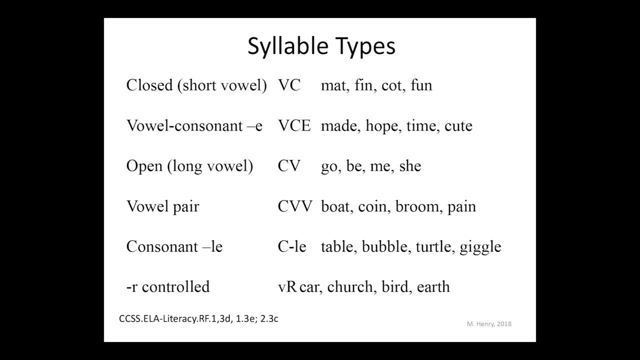 of the syllable: Go be me, she oboe, baby vacation. The vowel pair or vowel digraph: boat coin, broom pane. where I have a consonant, I mean a vowel digraph. 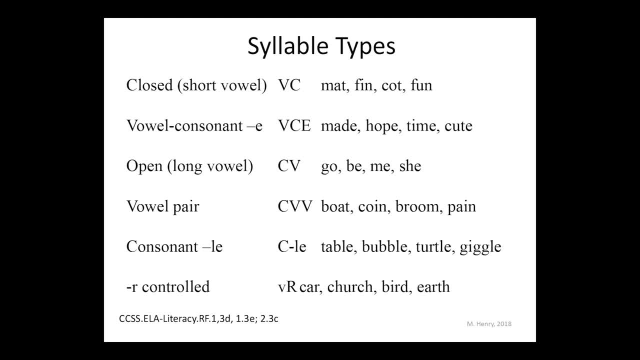 in the, usually in the middle, And then our consonant L-E: table bubble, turtle, giggle, sizzle and so on, And our R-controlled with the vowel followed by an R, as in car church. 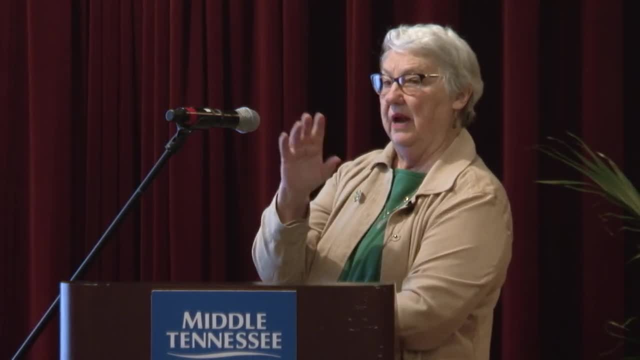 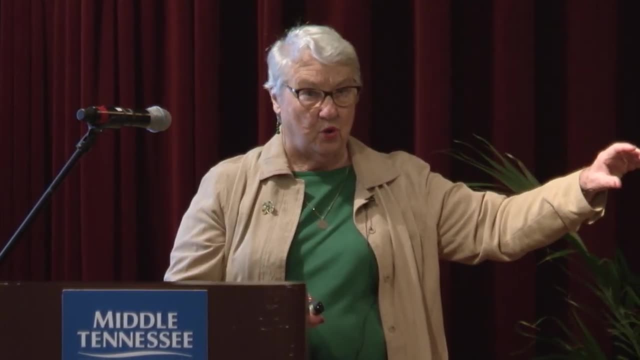 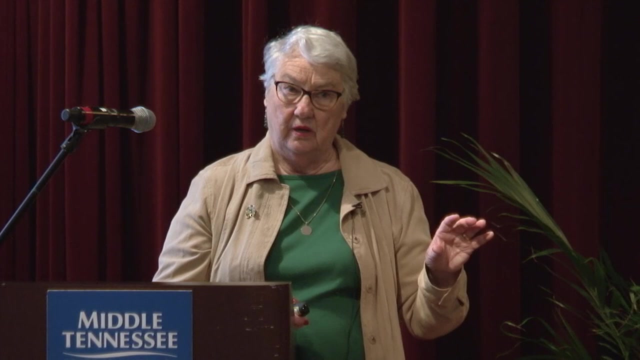 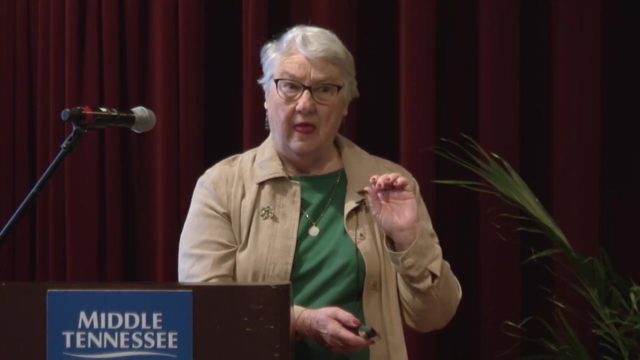 bird earth. Remember that I mentioned that when I showed you that three by three matrix, that what these different cells show are the strategies available for children to use. So I have a word that is a familiar word, They don't have to guess at it. 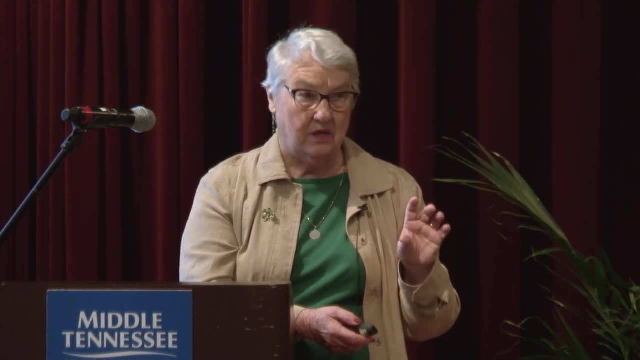 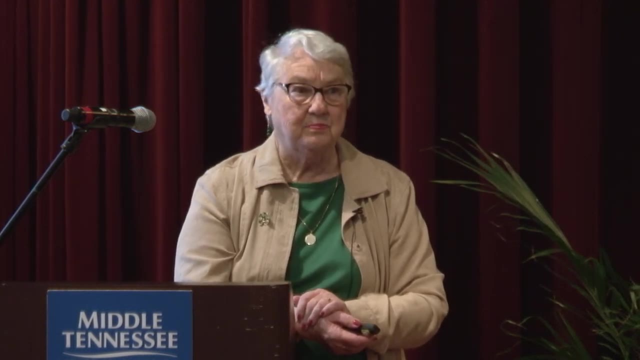 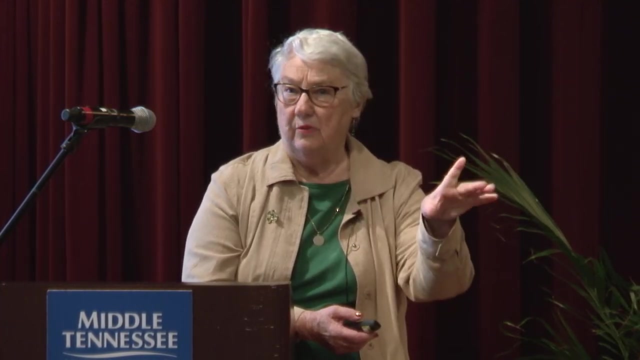 If it's a short word, a word of one syllable especially, they can usually sound it out letter by letter, sound by sound. So I have a word like grasp, Grasp. So I have to hear those five sounds. That is something. 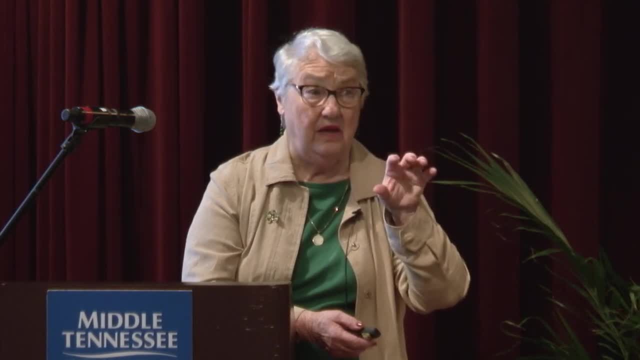 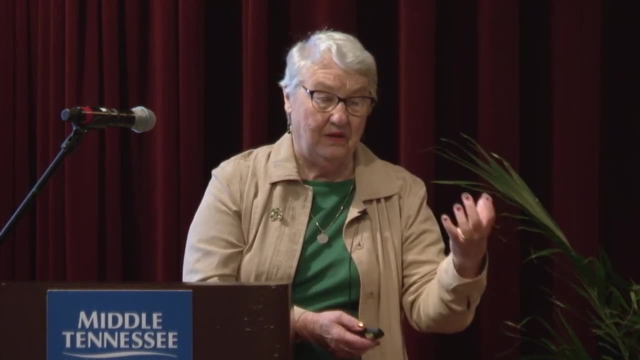 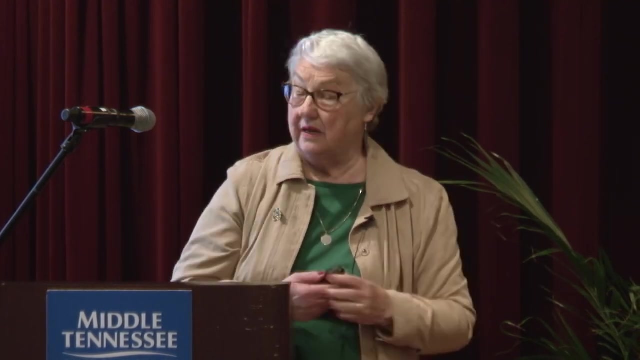 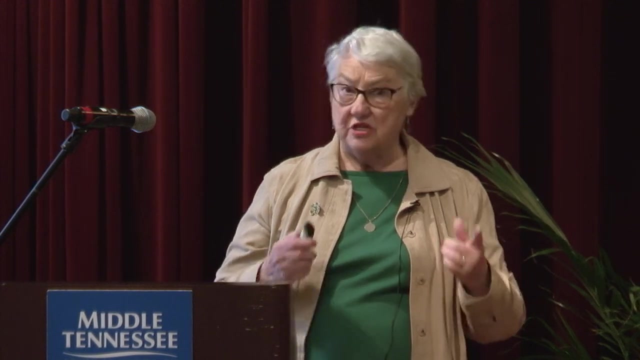 that is very necessary in order to get those five sounds. We have to be able to hear those And then, if we're spelling grasp, I go and I can write the corresponding letters. Syllables provide another strategy. Syllable division just. 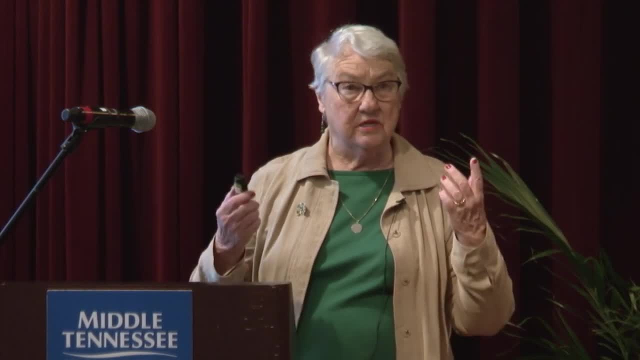 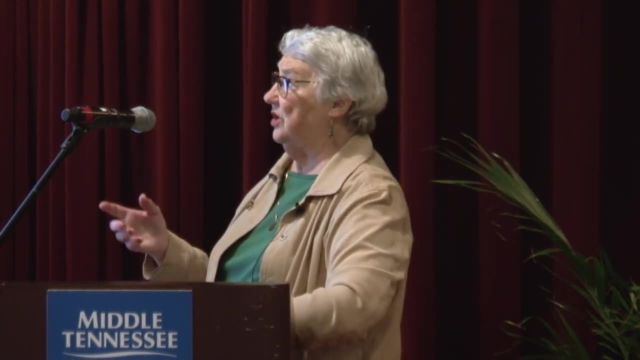 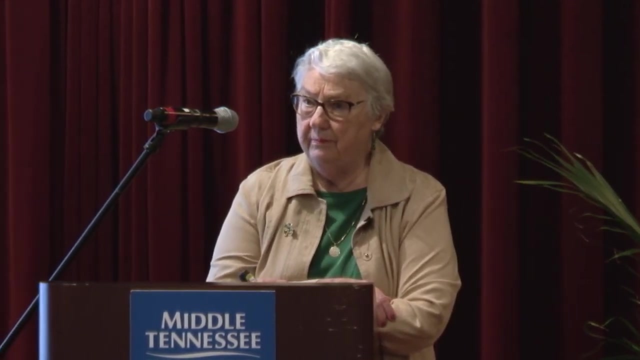 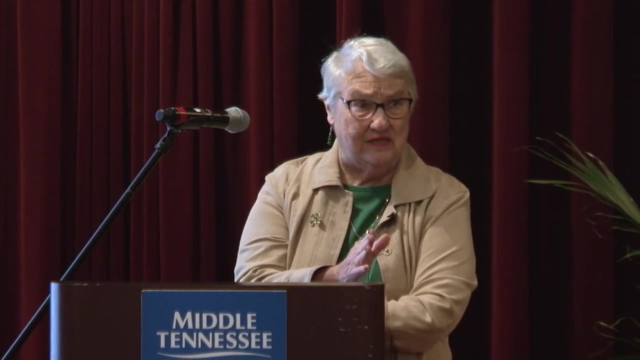 gives us another way to think about words And to a strategy for both decoding and spelling. Because if I have a word like campus, can I get campus by going? I can't. I have to do it one syllable at a time. So therefore, 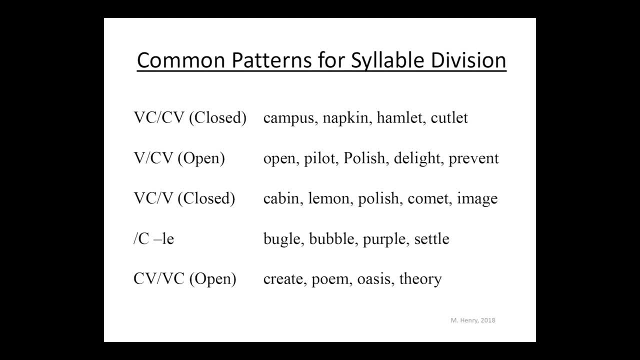 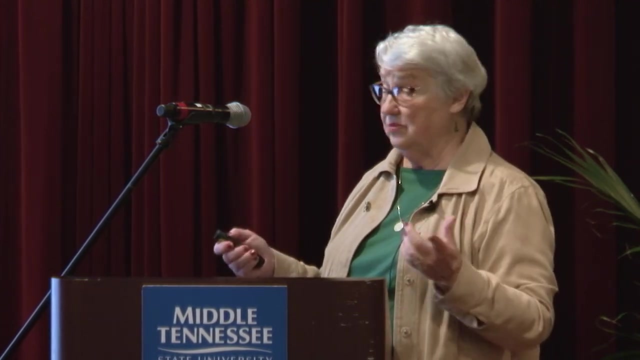 it's helpful to know that I'm going to divide into three parts And I can then sound out: campus, Campus, Napkin, Napkin And so on. When I have a vowel, consonant vowel pattern, I have two options And you always. 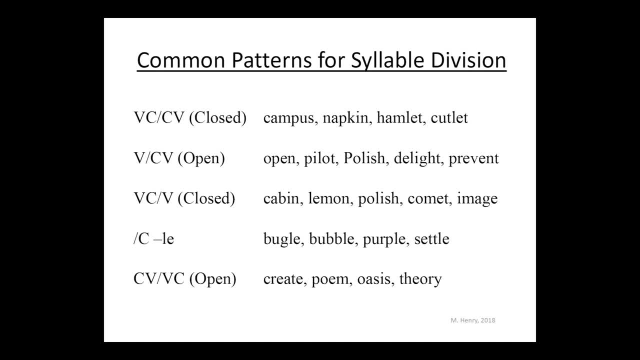 if you don't know the word. you always want your students to try the open syllable first, Open Prevent. But let's say they have cabin and they see that vowel- consonant vowel- and they go cabin. They know that doesn't sound right. 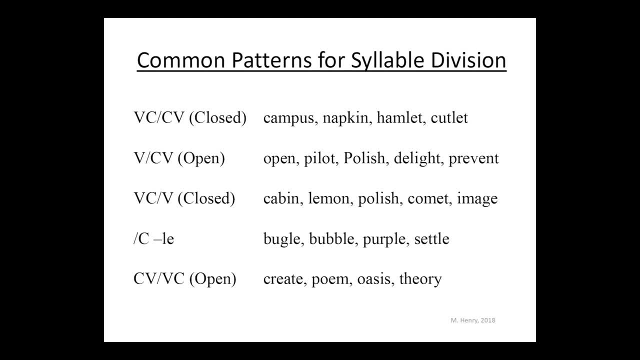 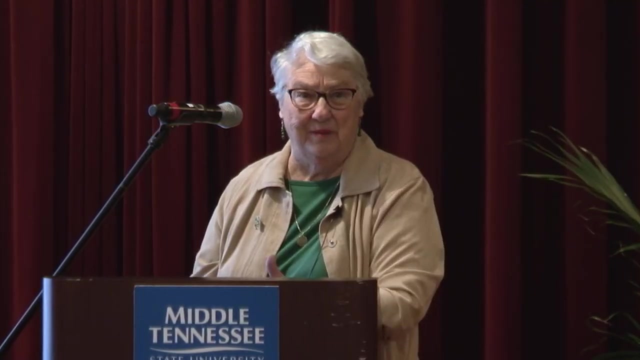 So they can try the alternative: Cabin Cabin Lemon. Polish Comet Image. Now look at the two that are spelled exactly the same. So how can I tell the difference? The capital letter doesn't matter, because I could say polish: the table. 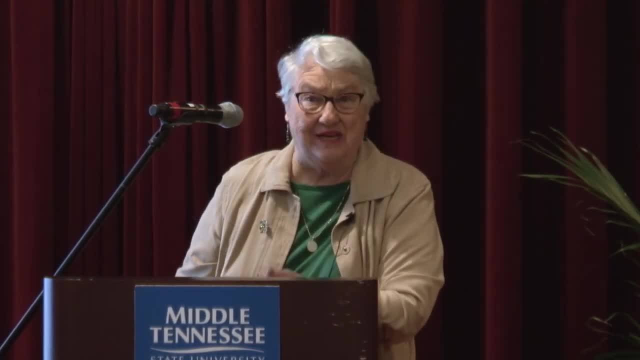 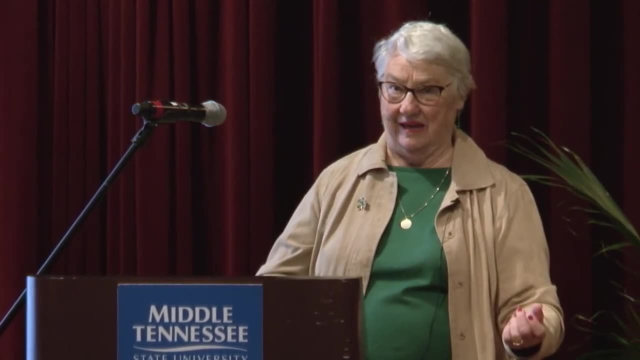 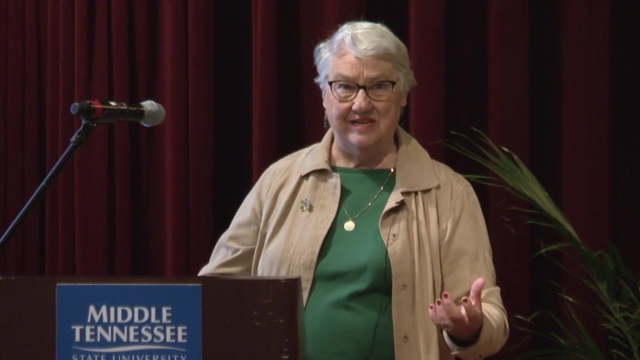 and it would come in. But I have to know the meaning, don't I? I have to know the context. Meaning is so important to spelling. Never emphasize that If I'm spelling the word read, I have to know: do I mean a read instrument? 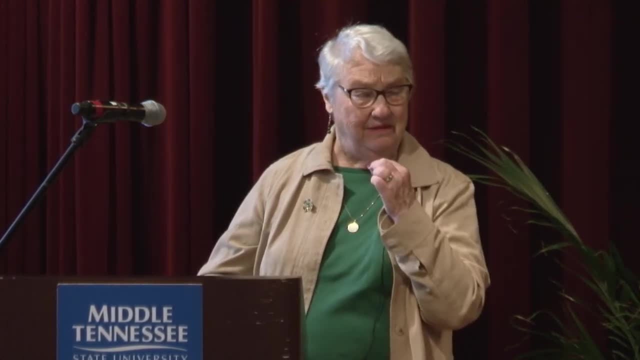 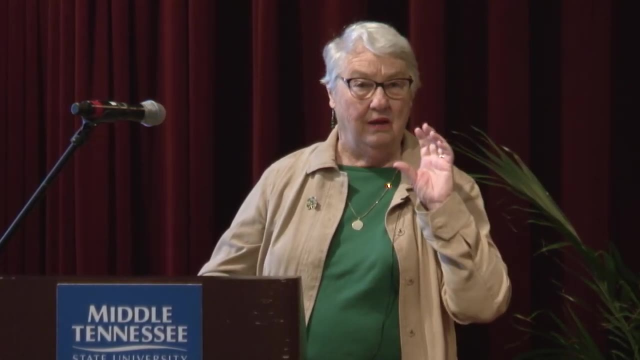 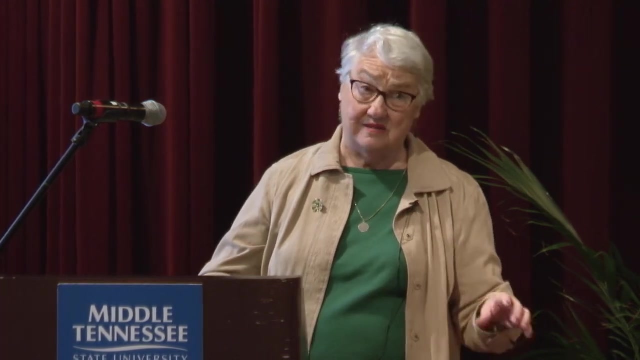 like a clarinet or an oboe that has a read: An R-E-E-D, Or am I reading a book R-E-A-D? So in a way the meaning is predominant to the sounds. Um, or at least you have to do it. 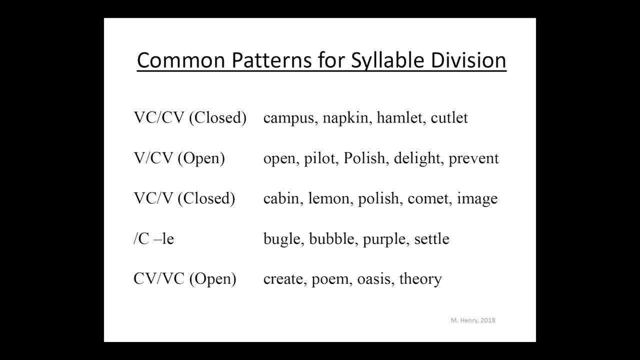 in combination. So we have Polish, meaning the nationality, and polish, And only in a context, in a sentence can I know which one is which. What happens with the consonant L-E words I have the consonant L-E, always stick together. 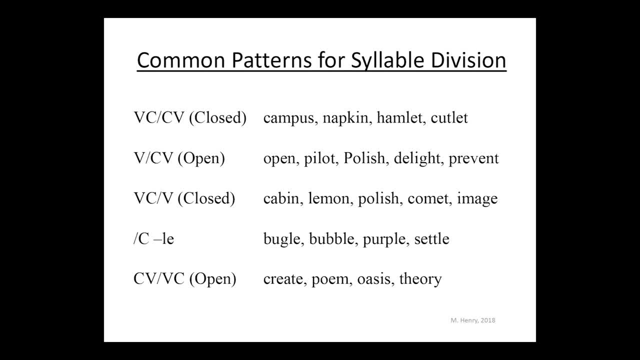 So that would be bugle, That you would be long If I spelled it with two G's. what would it say, Buggle Exactly. If I spelled bubble with one B, it would be buble, Exactly. The important thing to remember. 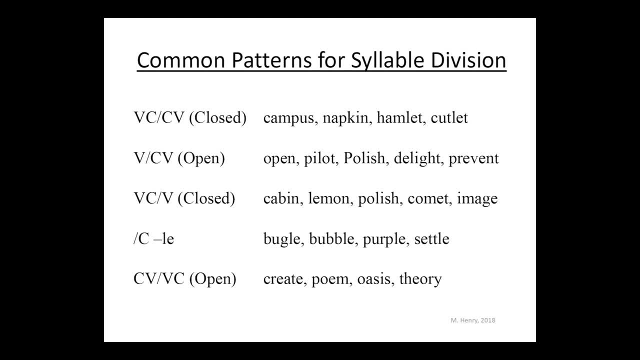 here is that you always keep that consonant L-E together And then you'll know if that's a long, an open syllable or a closed syllable. We have some words that have two vowels in the middle: Um Anna Gillingham. 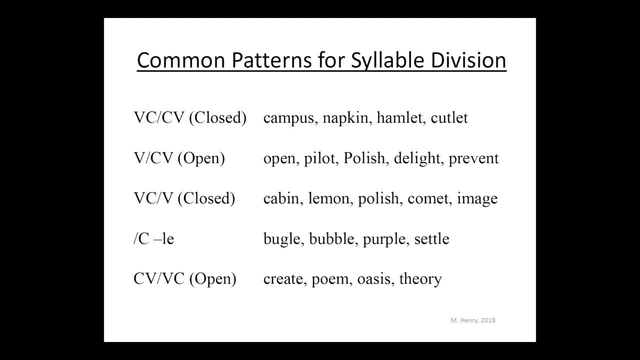 called these unstable diphthongs And um so we don't this word here. we don't say creet. That's not a vowel digraph. there is it. It's create. How many syllables in this word? It's. 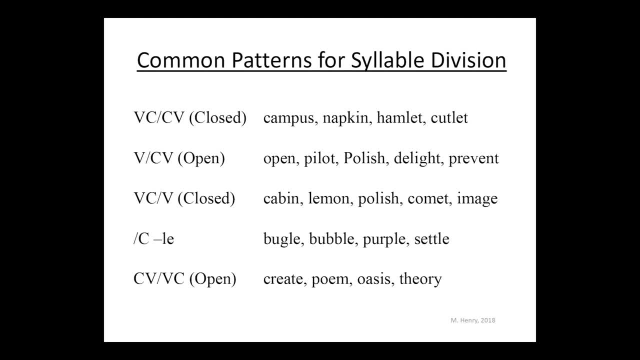 two, isn't it? It's not a poem. How many of you would say poem? Many of you might. A lot of people say it's a great poem, But it's a poem And when we hear the word poet, then you really hear the. 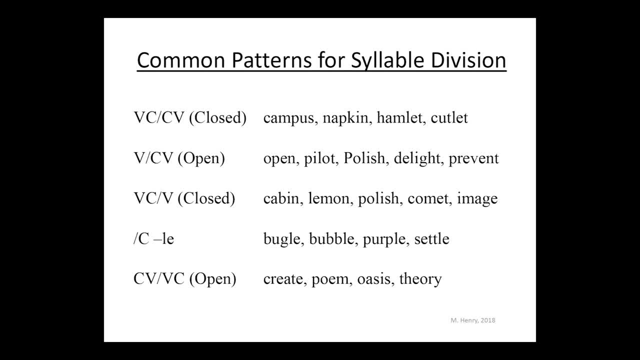 two sounds. But when you see that P-O-E, the O-E thing, oh, is it poem? No, it's poem. It's not osis, it's oasis. So I'm dividing: after the O, after the A, How many syllables? 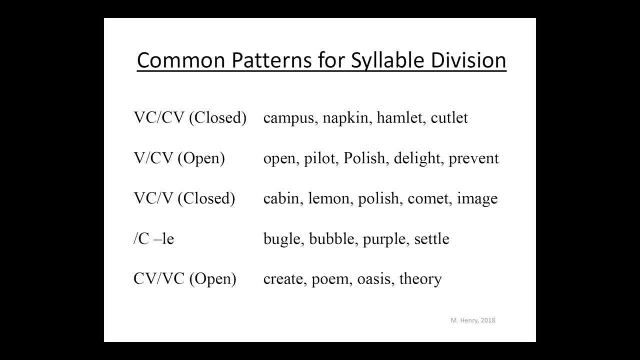 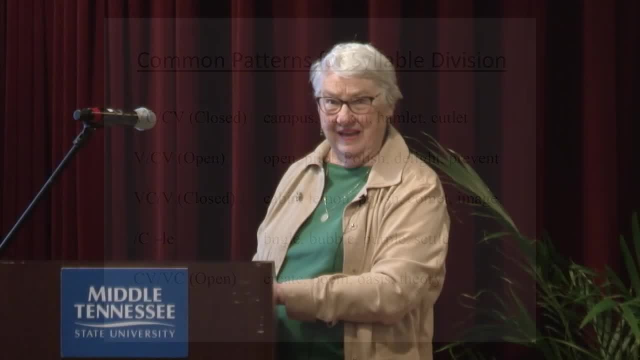 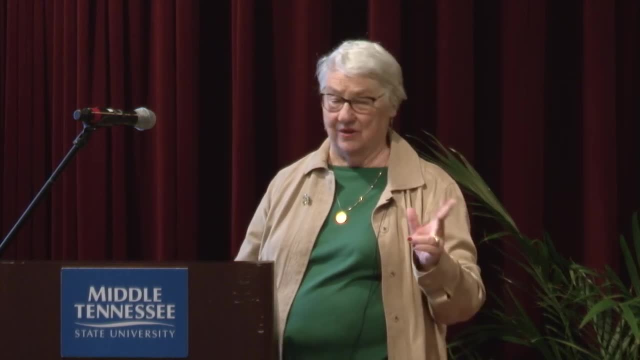 in this last word, It's three, isn't it? It's theory, It's not theory. And you hear it when I say theoretical The-o-re-ti-cal, Then you can hear it, But most people just say theory. But it's. 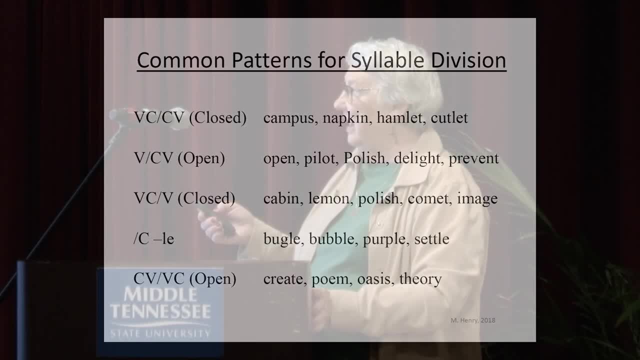 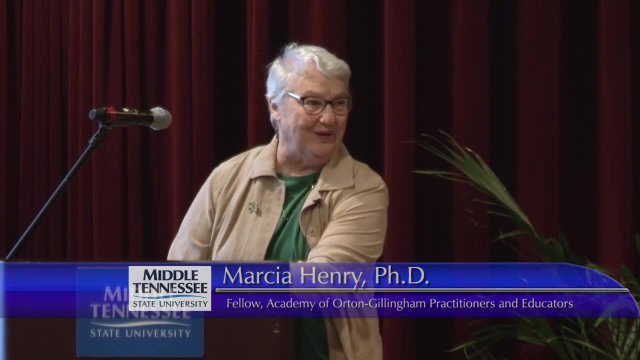 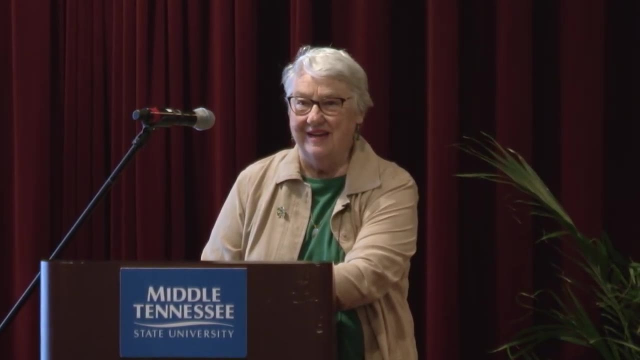 technically theory. Okay, I mentioned the work of Pete Bower and one of the participants here said that he had heard Pete and Gina Cook and I speak at an IDA conference five years ago, was it, or so? Yeah, And anyway. 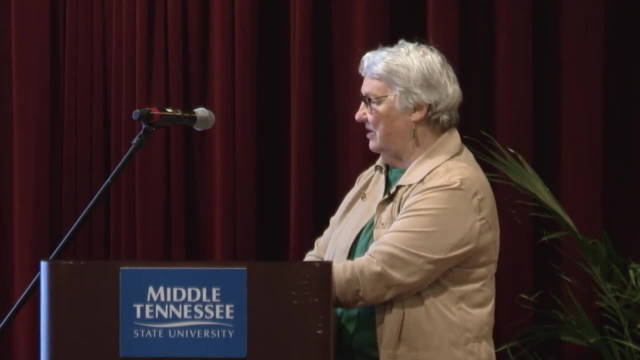 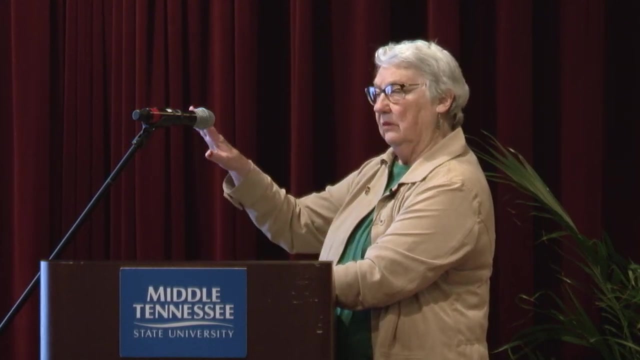 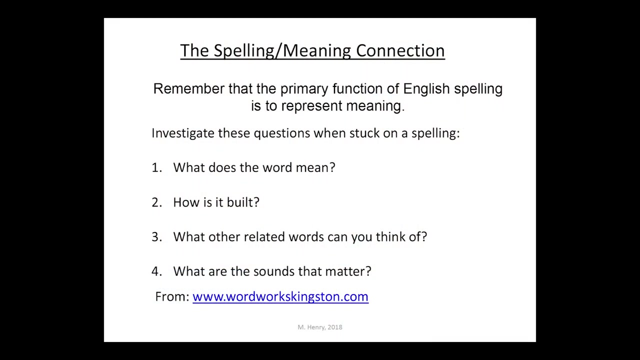 Pete just finished a doctorate at Queen's University in Kingston, Ontario, And he has a wonderful program called WordWorks in Kingston. And here's what he recommends: when you're stuck on a spelling, First of all figure out what does the word mean. 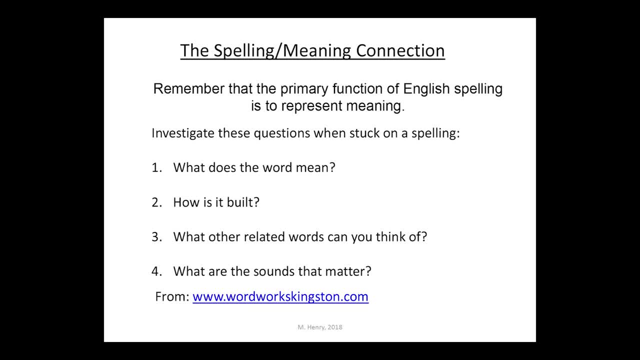 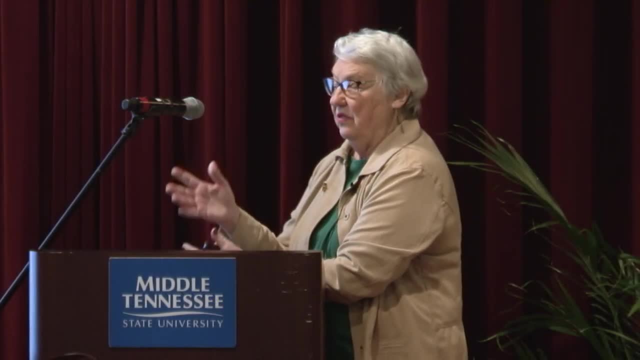 Does that help you out? How is it built? That means, what is the structure, Are there prefixes, Are there suffixes, etc. What other related words can you think of And those relationships could be? let's say the word is interruption and 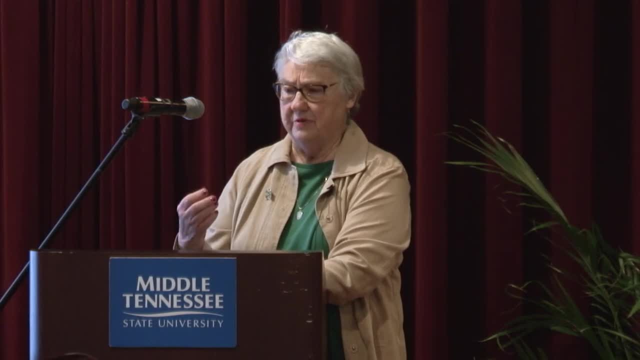 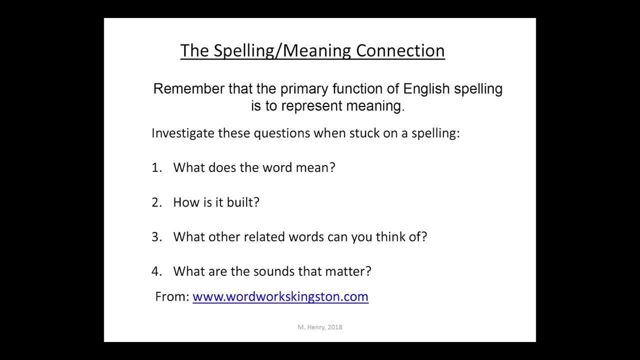 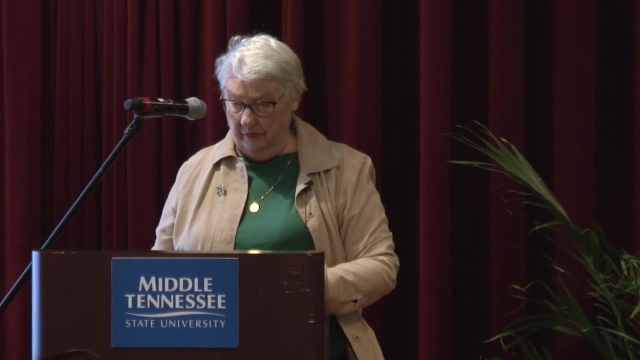 you see rupt, and then you think of abrupt and erupt and so on. Or they might be related semantically in terms of what other synonyms and so on. And what are the sounds that matter? Some people think that Pete and some of his colleagues 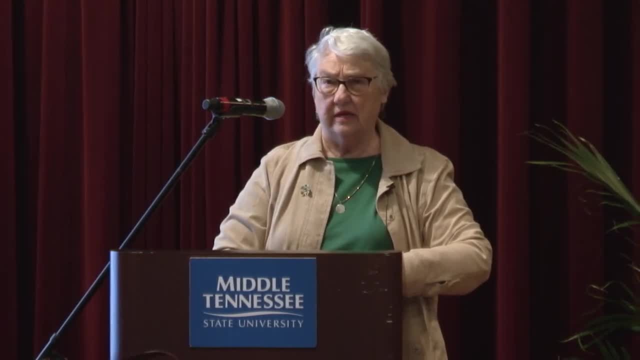 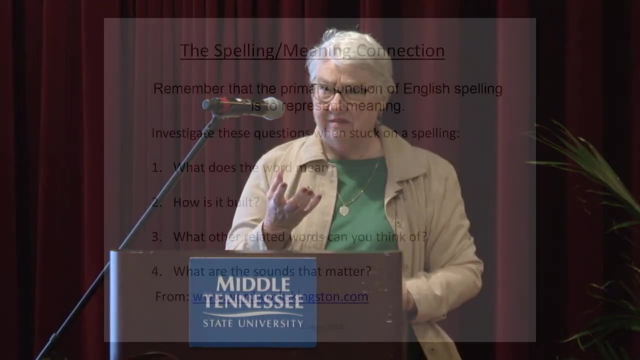 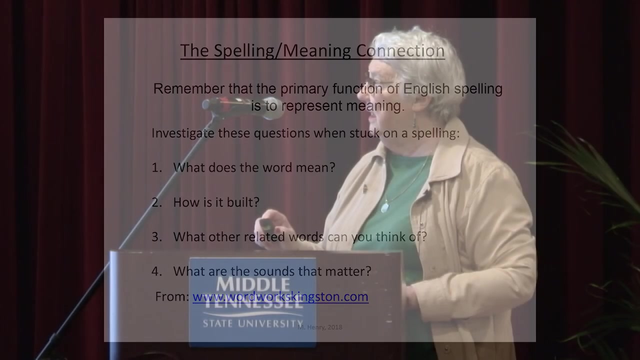 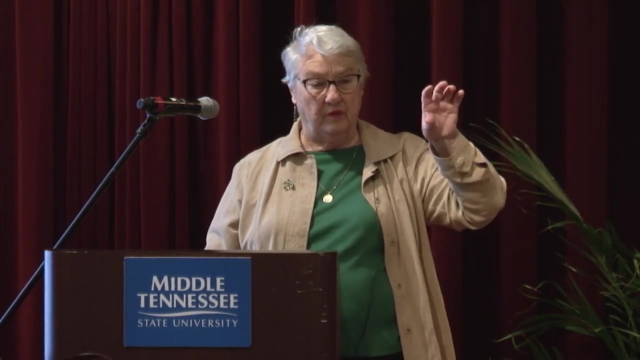 have gone overboard on morphology to neglect phonology. and they don't at all, But phonology kind of comes last. What are the sounds that matter? as you're spelling this word, Now, what happens? remember that matrix, and we have the letter sound correspondences. 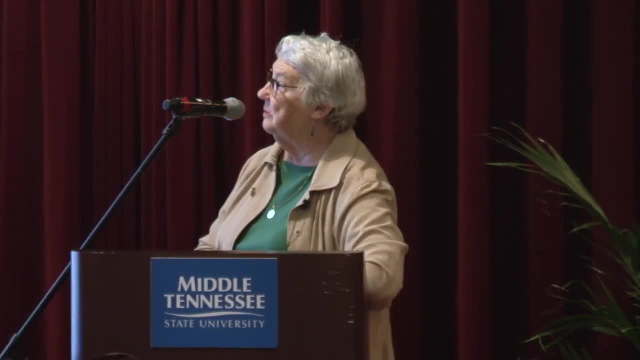 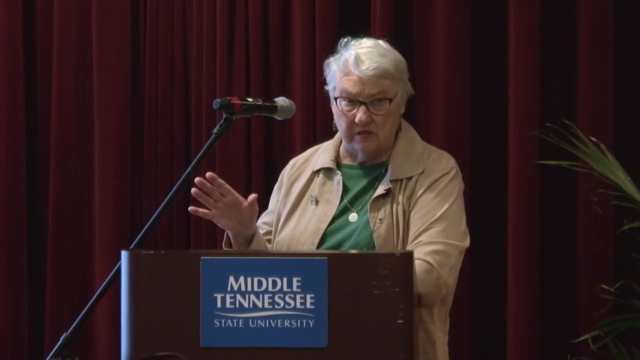 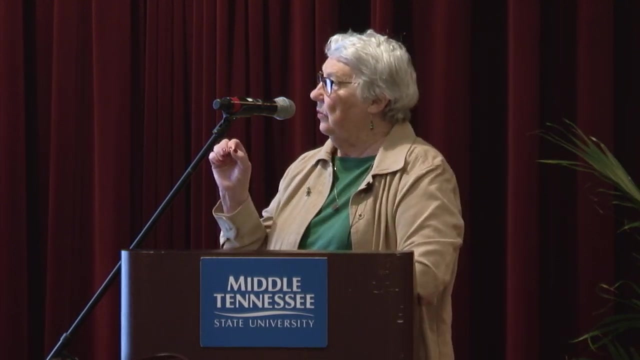 the syllable patterns and the morpheme patterns. What happens with the? remember? the morpheme patterns are meaning units, That is, they have specific meaning, And we're going to talk about the difference with semantic meaning and syntactic meaning in just a minute. 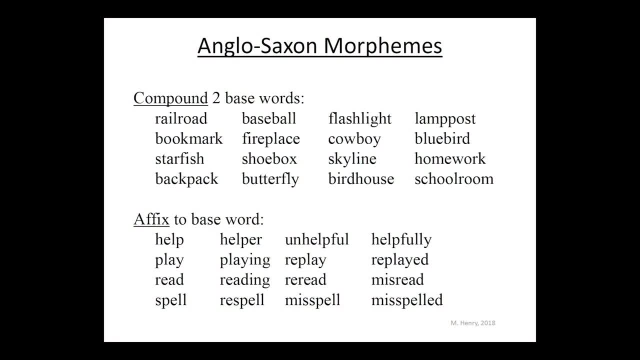 But what happens with the Anglo-Saxon morphemes? To expand words, to add morphemes, we do one of two things: We either compound or we affix. By compounding, we take two of those little Anglo-Saxon base words and we put them together. 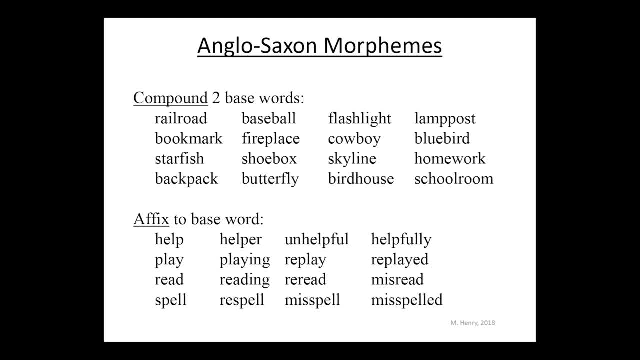 So I have railroad baseball, flashlight, lamp post, bookmark, fireplace cowboy, or we affix, we add prefixes or suffixes. So help, helper, unhelpful, helpfully play. playing replay replayed. 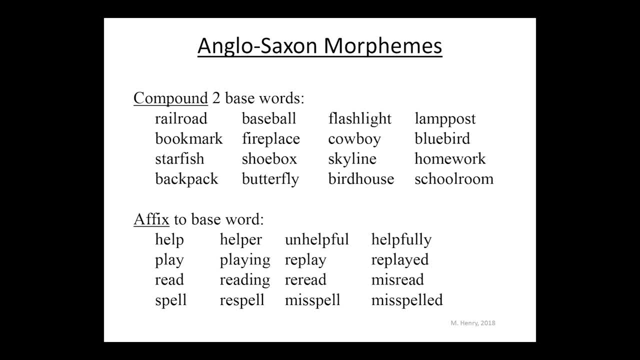 read, reading, reread, misread and so on. So these are little words. we've got basic words, but we've added suffixes or prefixes, So we can either compound or we can affix. Now think about: remember that the morpheme is the smallest meaningful unit of language. Count the meaning in these words. I mean count the morphemes. How many in dogs? Two, exactly, Dog, plus the plural s. How about railroad Right? How about? 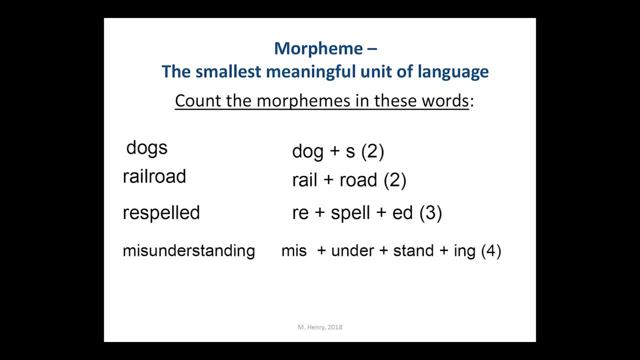 re-spelled Three. I have re-spell and the e-d. How about? how about this one? It's four. Mis-under-standing, Mis-under-standing. How many syllables in that word? Five, exactly Five syllables. 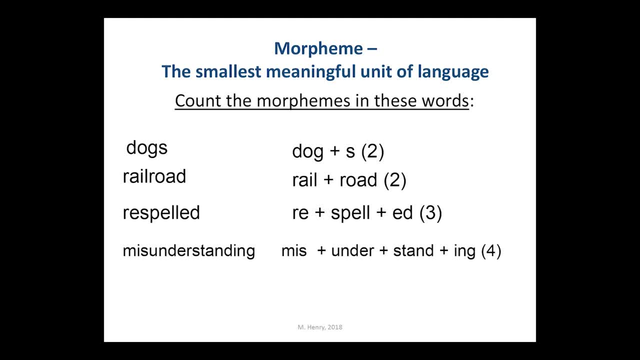 but for me morpheme- because under is a morpheme, Un- is also a morpheme, if I have it like unhappy, unlikely, but dur is not anything. I mean, it's not an affix and it's not a base. 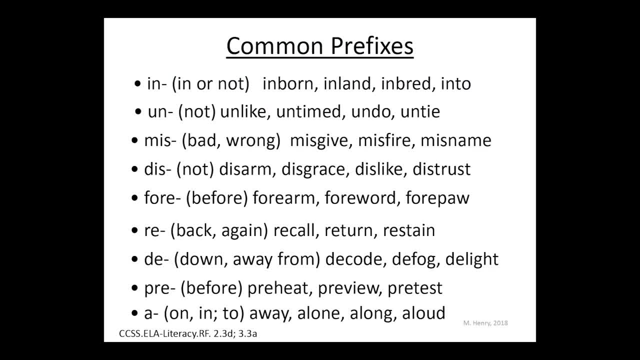 So I have four. Now what are the most common prefixes that we teach? first, We have in meaning, with two meanings: in or not. We have un- meaning not Mis-bad or wrong, Dis-. Now notice those first four. 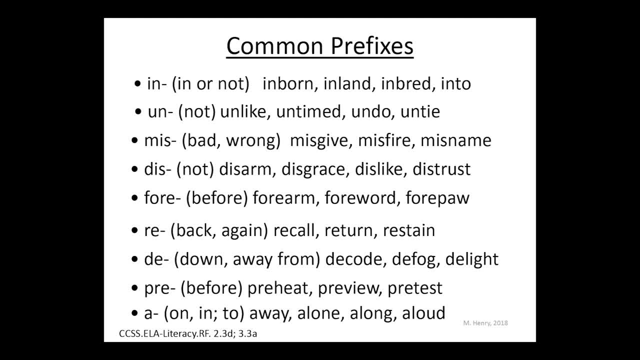 are all prefixes with short vowels, They're closed syllables. We have four f-o-r-e, We have re- and d- and pre-, all with very specific meanings, And we have, uh, I don't say ah or ay, do I? 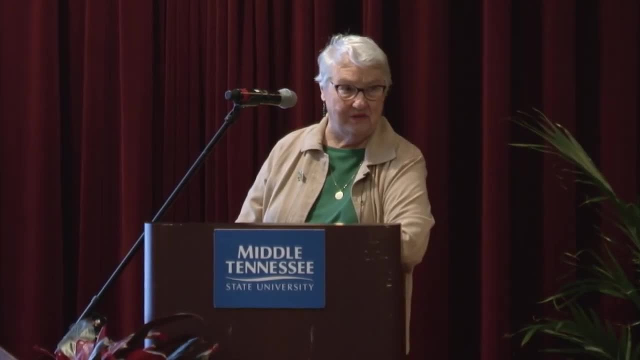 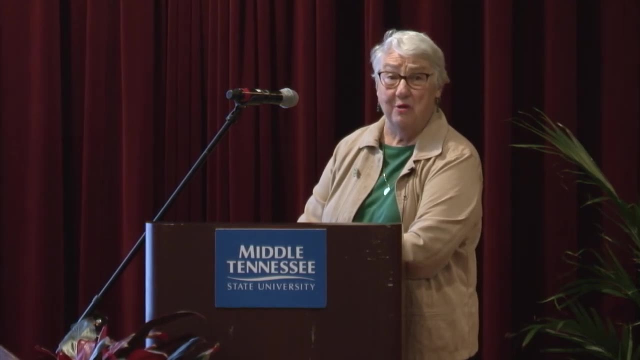 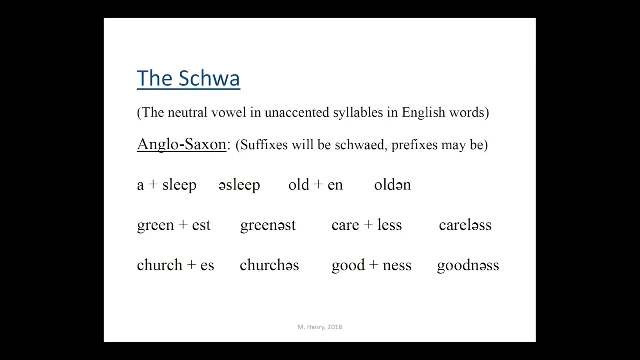 What do we call this? uh, sound The schwa. Good, A lovely word. Most vowels are schwaed And a schwa happens when you have a non-stressed syllable. It's the neutral vowel in the extended syllables. 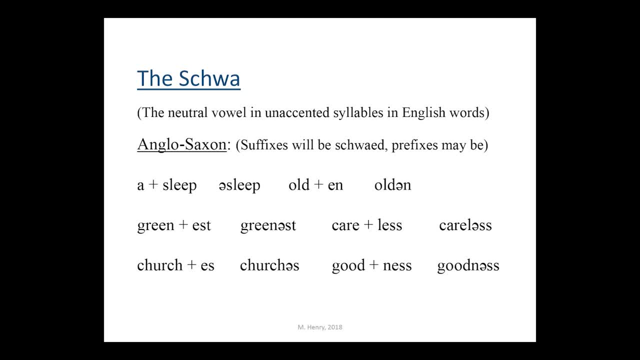 So usually prefixes will be. suffix will almost always be schwaed And prefixes sometimes Asleep Olden Greenest. I don't say est, The suffix isn't est, it's est Careless, It's not less. 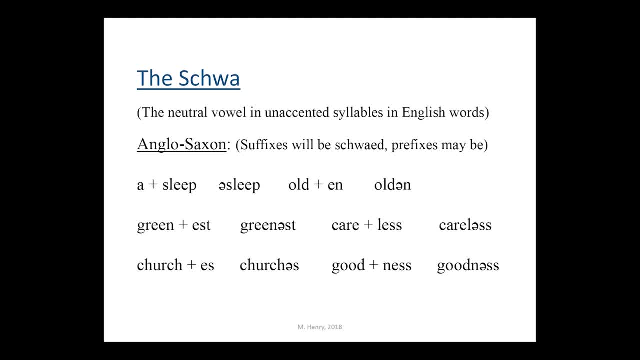 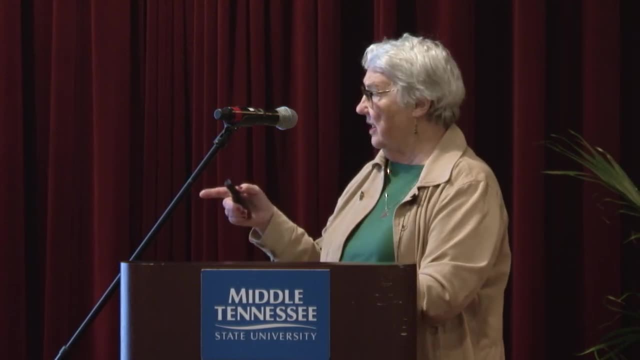 It's careless. The accent comes on the base. usually These are unaccented And the schwa's diacritical marking is that upside down e. So if you're looking up a word in a dictionary, you'll see that upside down e. 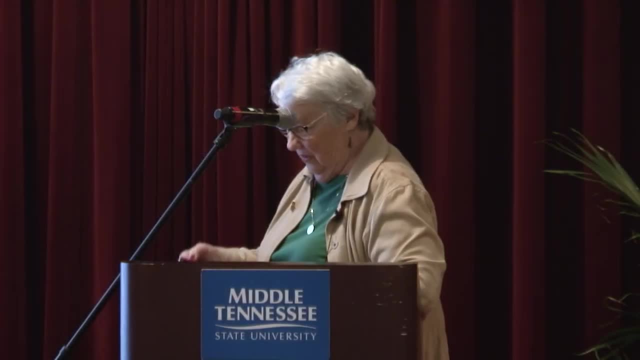 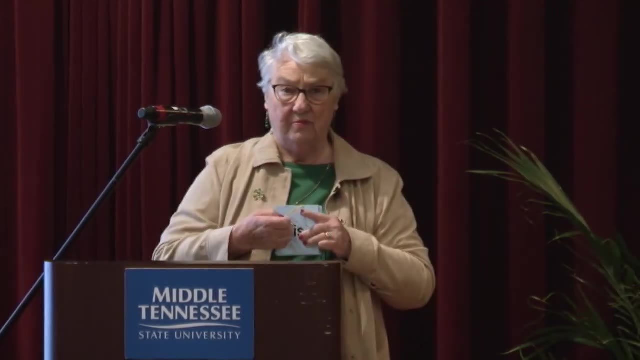 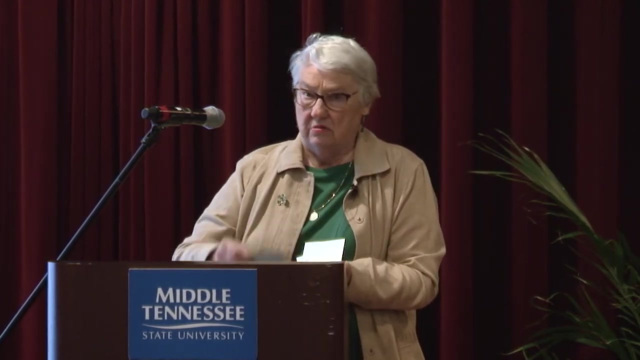 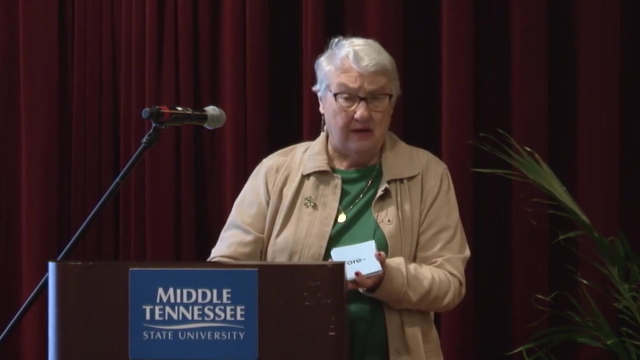 Church, churches and goodness. Now, what I do? I like to. I just make cards for my students because I want these prefixes to be absolutely automatic for them. What we find is, if the morphemes are automatic, this helps fluency. 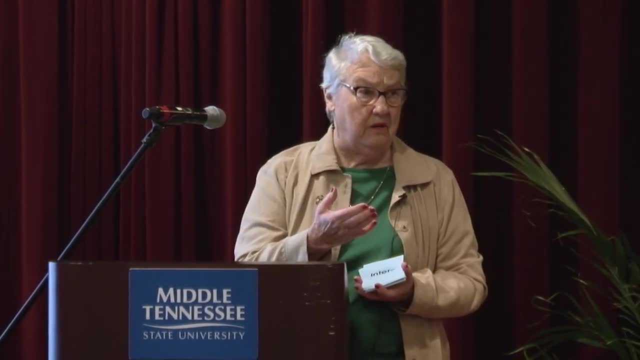 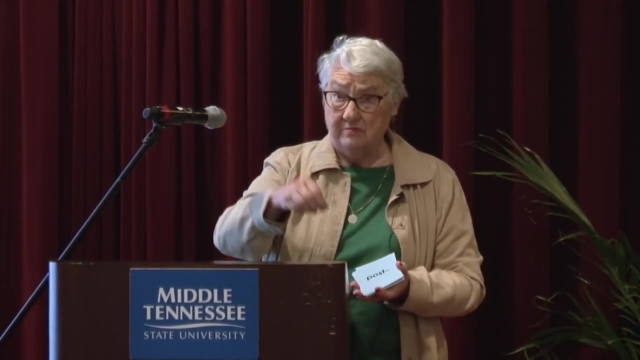 That automaticity adds to the fluency We know. fluency is one of our goals in reading, isn't it? In decoding And in spelling? We want them to be able to write it quickly. Well, if they recognize these immediately and know how to. 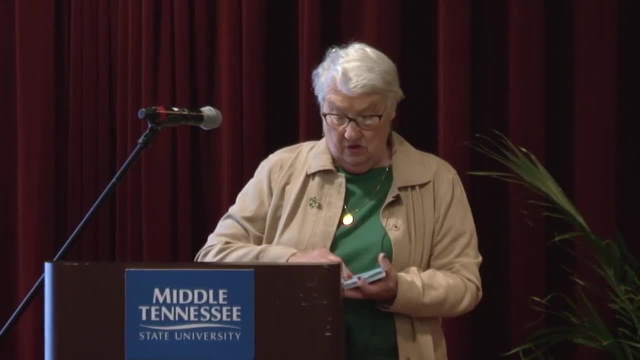 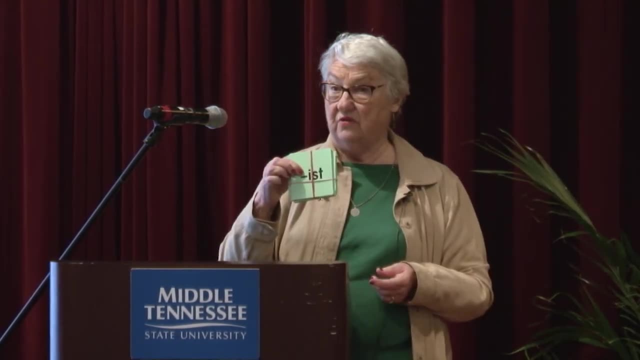 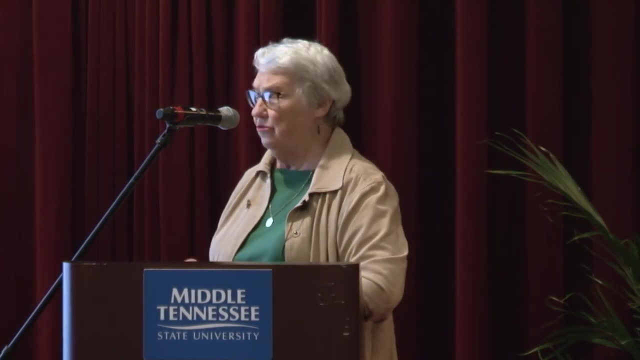 spell them. that'll be very useful. So I like to color code the different cards. I have the same kind of thing for suffixes, With the common suffixes. Now suffixes do something kind of interesting. We have our inflected endings. 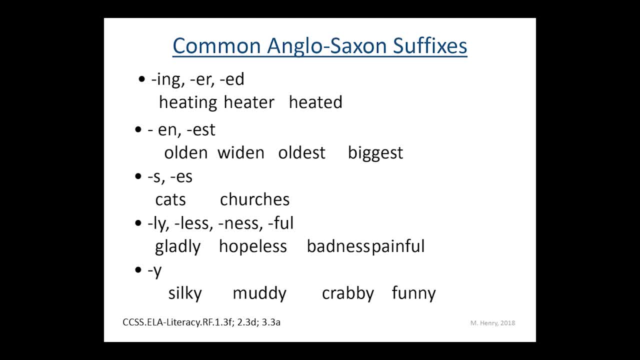 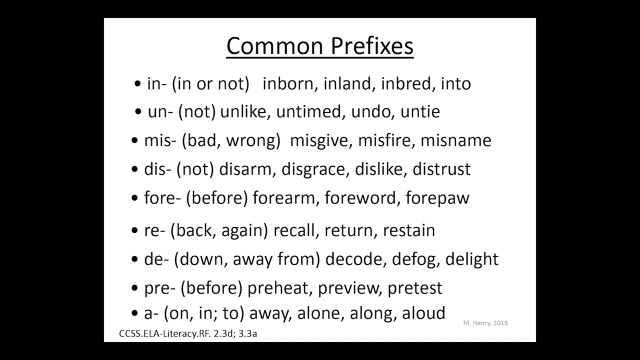 We have our plurals. Here are another four very useful suffixes. These are the most common suffixes, And suffixes have a different kind of meaning than prefixes. Prefixes and roots have a very specific semantic meaning Like not, or, in, or. 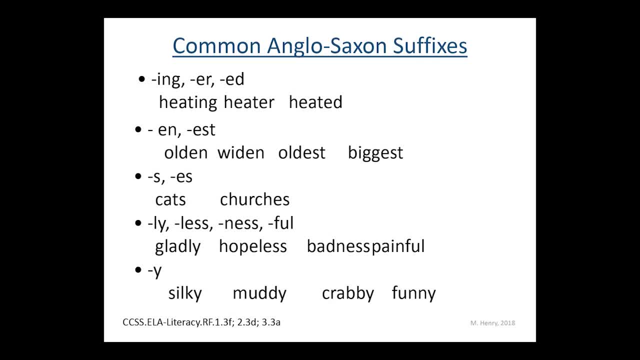 whatever, But suffixes tend to have a syntactic meaning. The suffix puts a word into a certain part of speech. We'll get into that as we go into some of the derivative suffixes. Here are some of these. Now, this is just kind of. 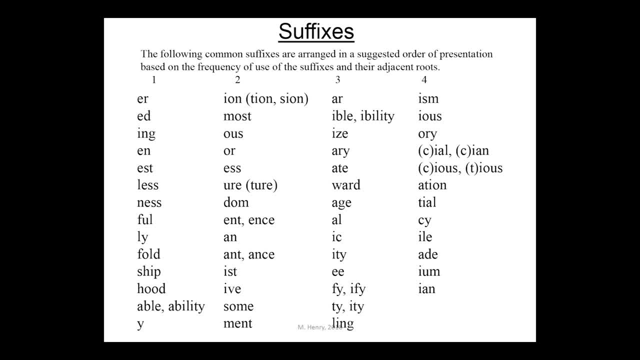 by column. The ones that I teach first are generally the ones we can add with Anglo-Saxon base words, So they're the ones we learn first. Then we have the I-O-N, We have most us, etc. Now one of the 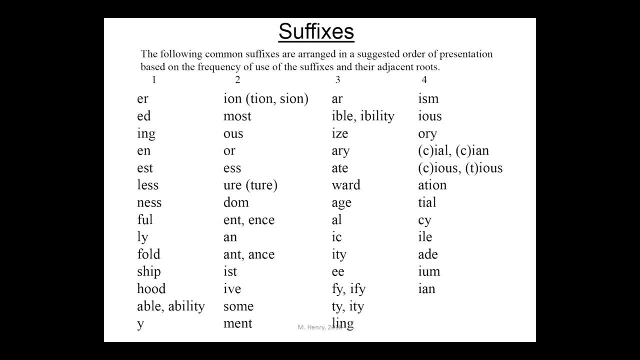 things that you have to be aware of. O-U-S and E-S-S both say what They're both schwaad and they say us, So how do I know which one to use? When do I use O-U-S? With what? 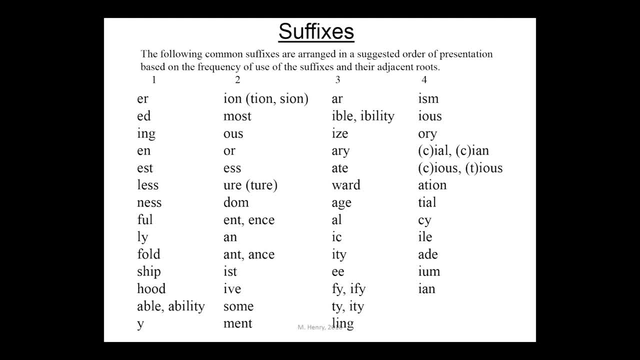 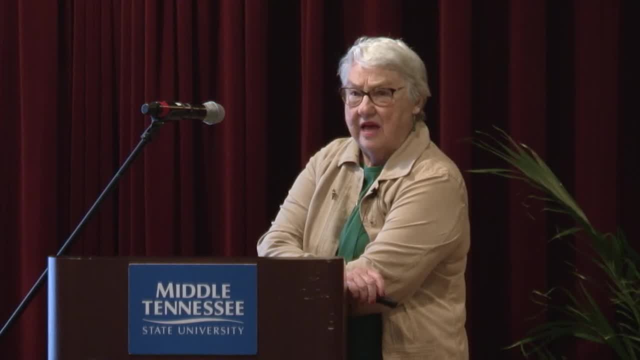 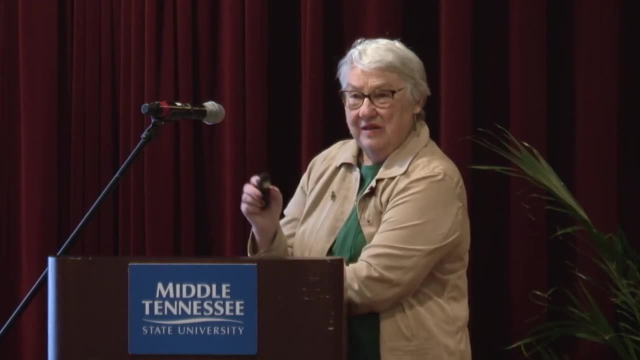 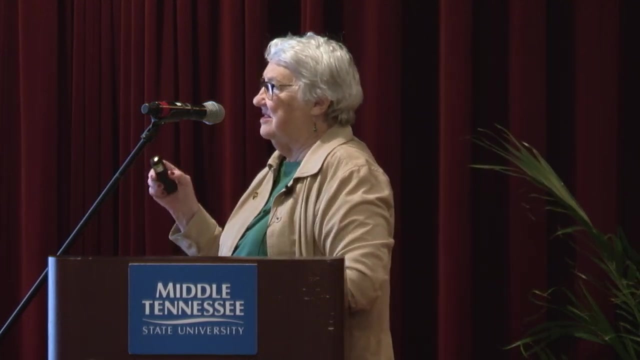 Which part of speech? Dangerous, adventurous, humorous adjective. How about E-S-S Actress governess princess, Feminine noun Right. These are things we can teach to children so that they can understand that this language is not all a language. 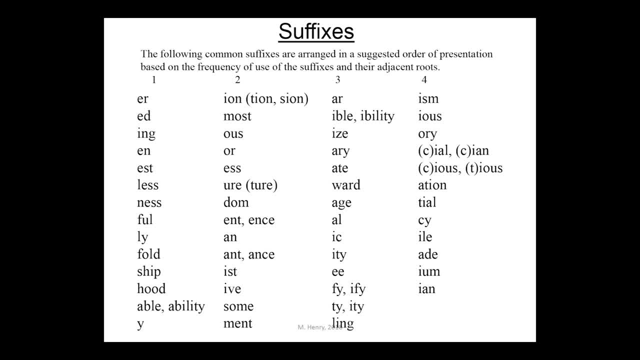 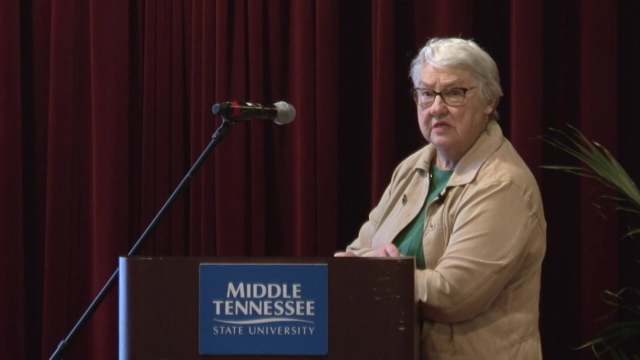 of exceptions. This is fairly regular. Look at the suffix: E-R versus O-R versus A-R. They all say er, but E-R is usually used with Anglo-Saxon base words for noun or adjective: Skater, baker, older, smaller. 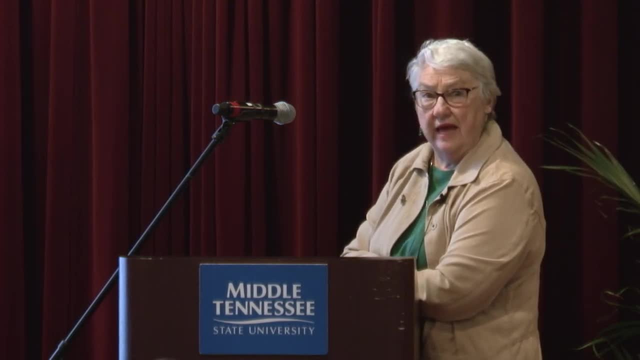 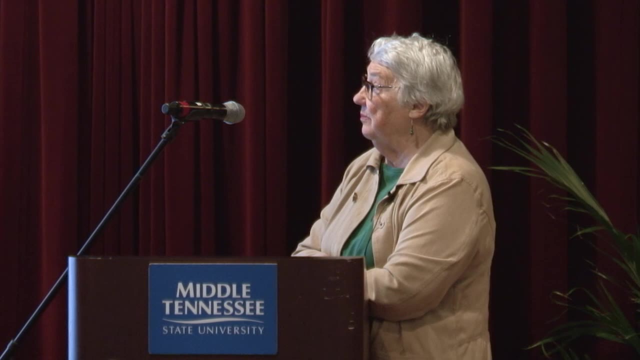 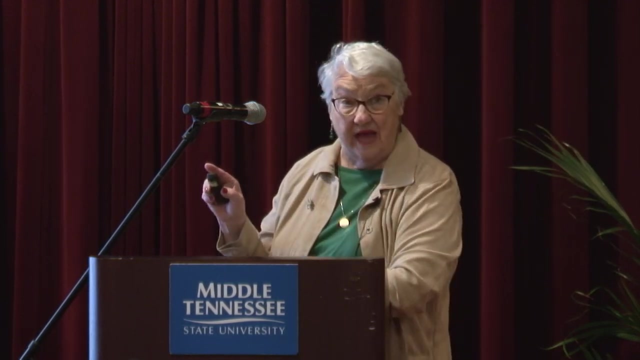 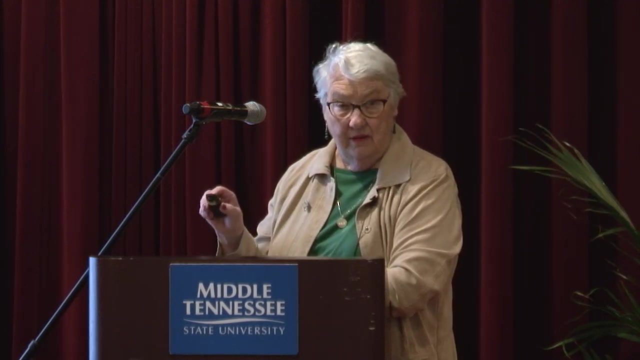 O-R is usually used with Latin roots: Conductor, inspector and so on. O-R is almost always used as a noun. A-R is used with Latin as an adjective: Spectacular, popular and so on. So these are. 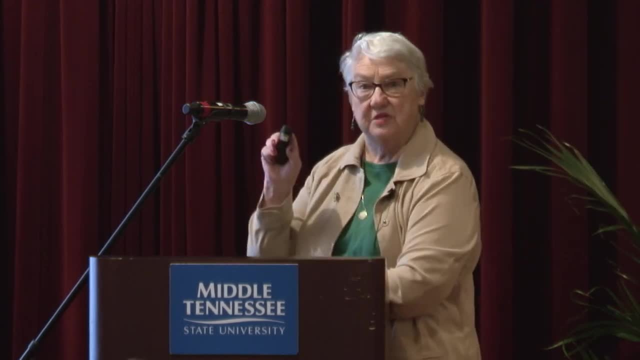 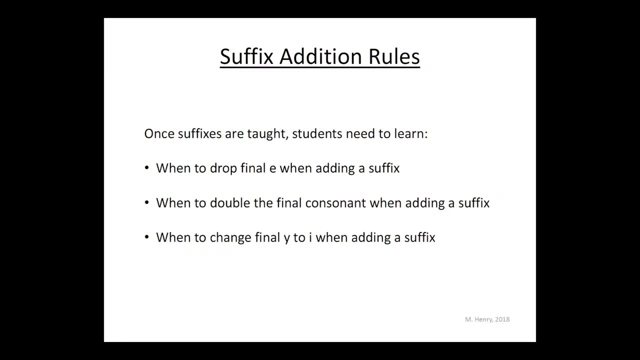 things that we can teach our kids that help them to spell these words. Now we do have to add the suffix addition rules. I'm not going to get into those specifically, but we have to know when to drop a final E when adding a suffix. 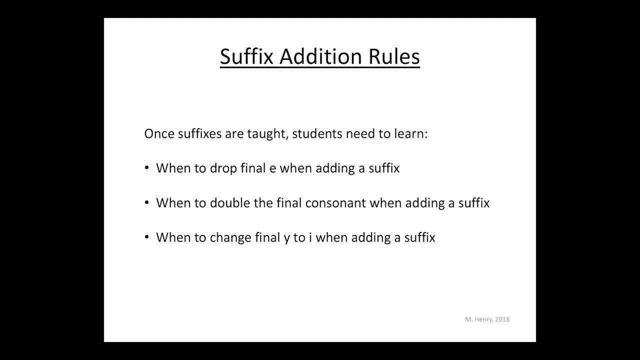 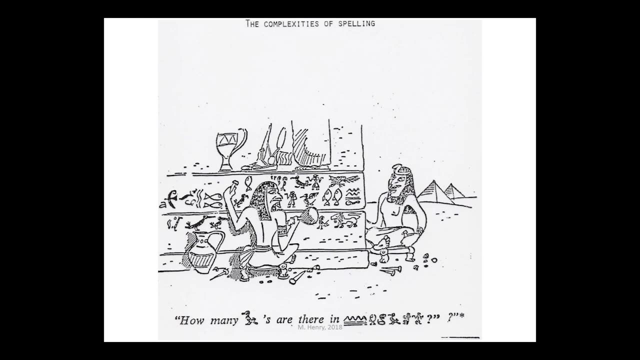 when to double the final consonant, when adding a suffix, or when to change a final Y to I. So all of you should know that and figure that out. Here's the Egyptians doing their hieroglyphic. How many are there in? 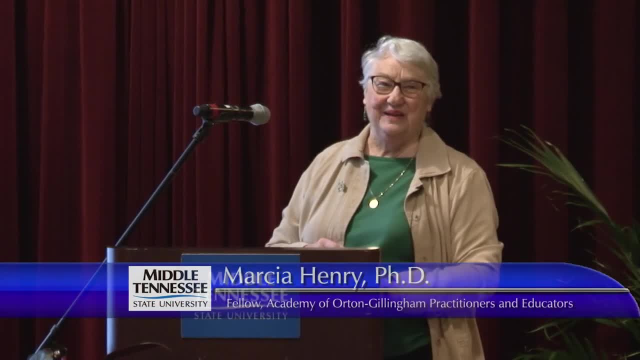 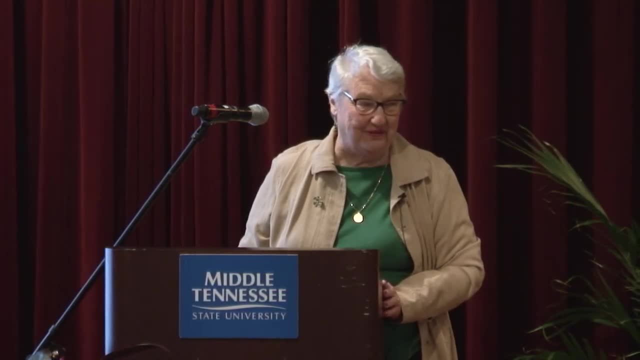 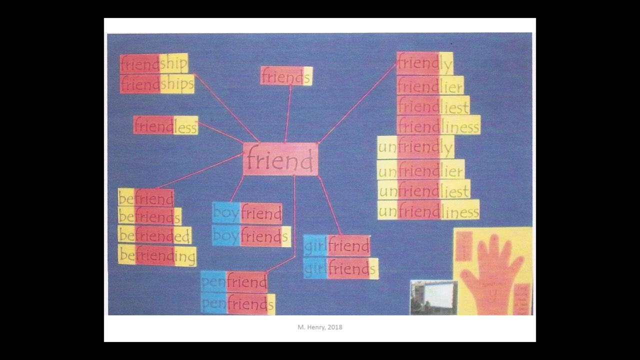 whatever It's like. does bigger have one or two G's? Does swimmer have one or two M's? Now, one of the things that I think is fun to do when you're working with M's is to have kids do activities like this. 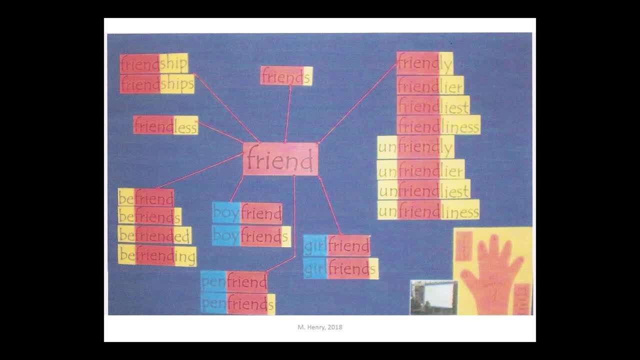 You can do this on the board, Have them. you could maybe choose the base word. So here we have friend, We have friendship and friendships. We have friendless, We have friends, Then, friendly, friendlier, friendliest friendliness. 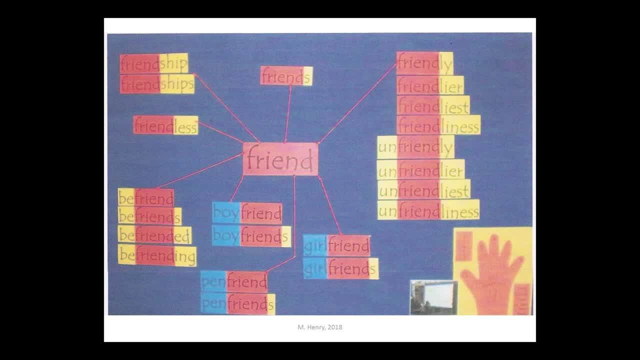 unfriendly, unfriendlier friendliness, girlfriend, girlfriends, pen friend. This was done at a school in China, in Beijing, an international school. So I guess a pen friend would be what we would call a pen pal, Boyfriend, boyfriends. 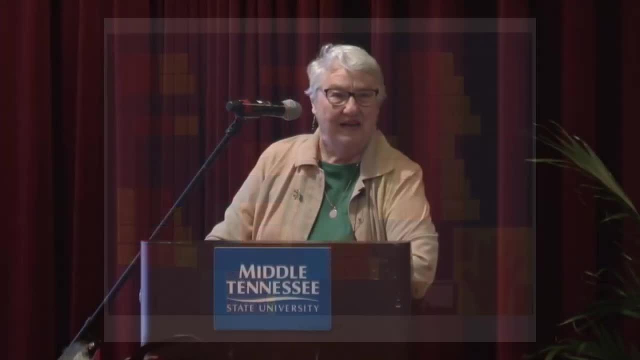 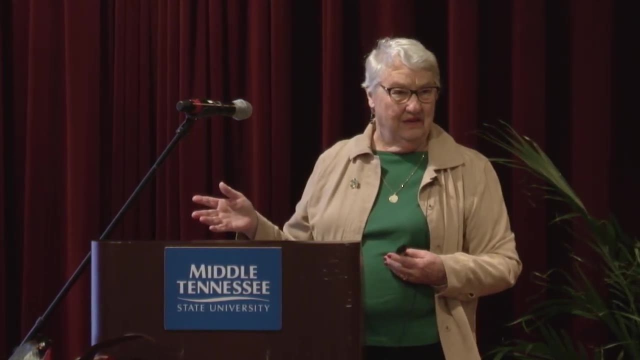 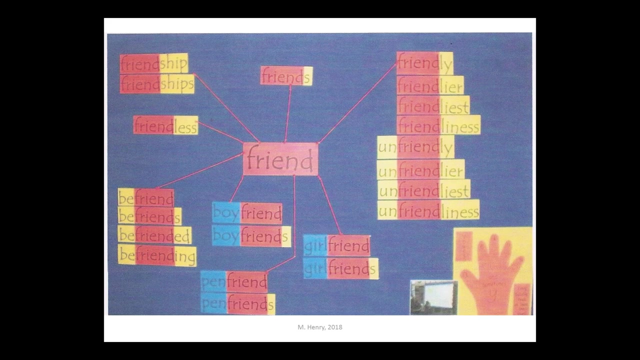 befriend, befriends, befriended, befriending. Showing kids how words expand- These are wonderful group activities. You can get two or three kids together to be making these kinds of word walls and word charts. This is from Pete Bauer's. 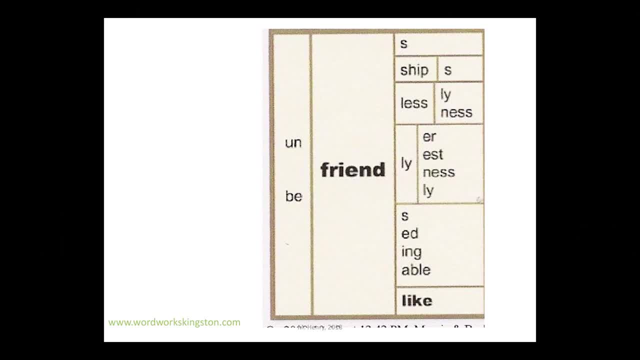 word works, What he calls a word matrix. So I have my base word here, friend. Then my prefixes with friend could be un or be. Then I can show all the different suffixes that I could use with that Notice. friend is in bold. 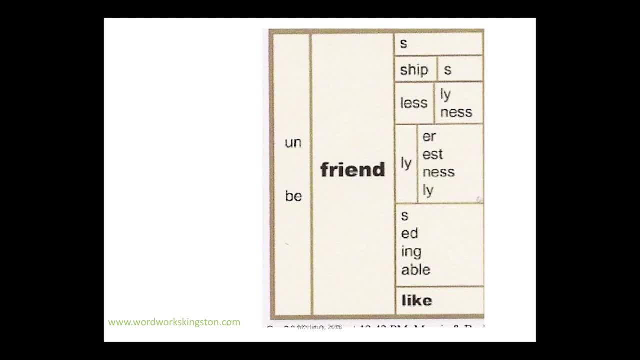 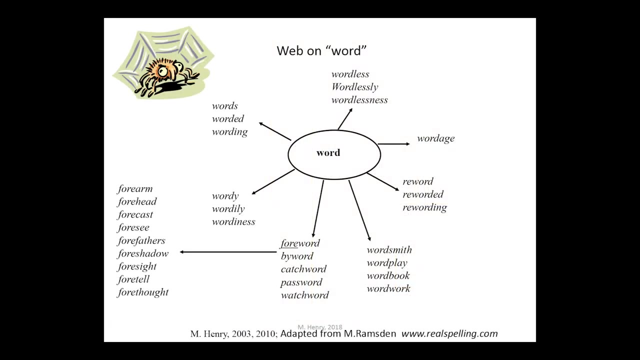 and like is in bold, because here I've got a compound don't I Friendlike, So I have to bold face the base words there. This is from Michel Rameau's work Real Spelling. He has a new website. 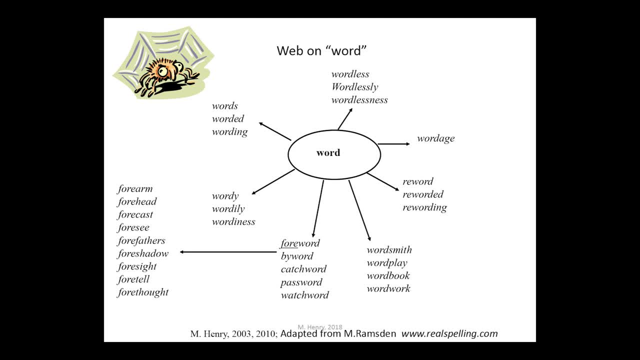 It's realspellingfr, which means France. It's worth looking at, But we have word, words, worded, wording, wordless, wordlessly, wordlessness, wordage, reword, reworded, and so on. 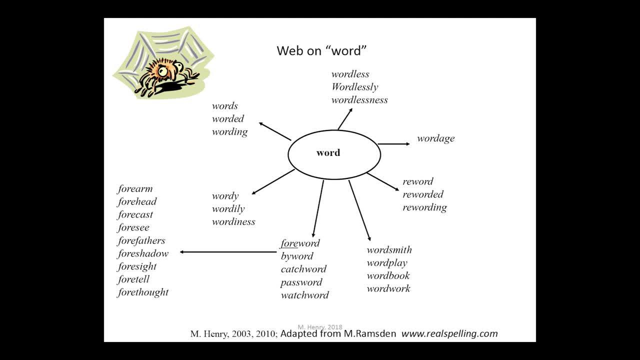 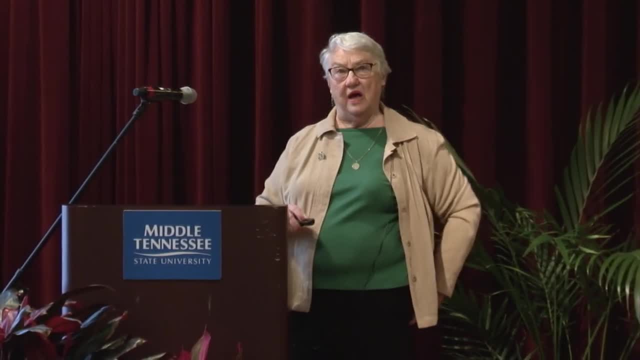 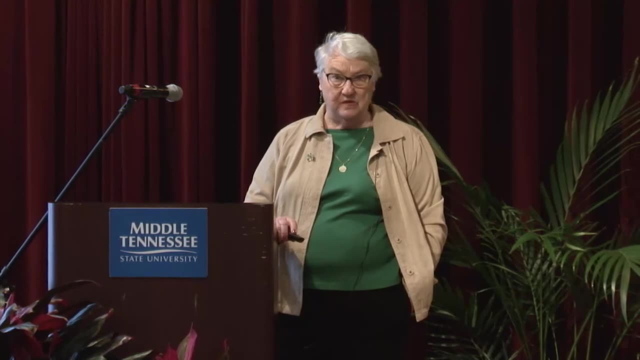 You know, giving kids the sense of how we can expand on these words. Now I want to move on for the rest of the morning to why we need to learn the Latin and Greek morphemes. How many of you are working with kids three and above grade three? 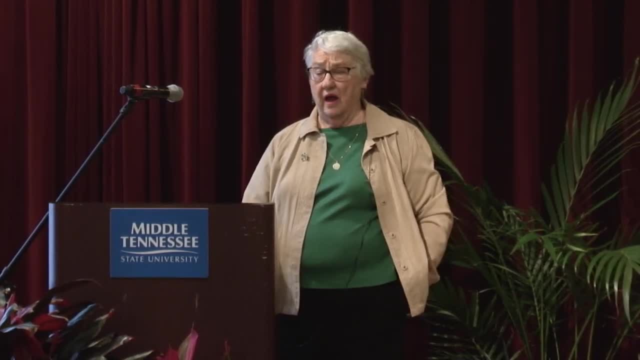 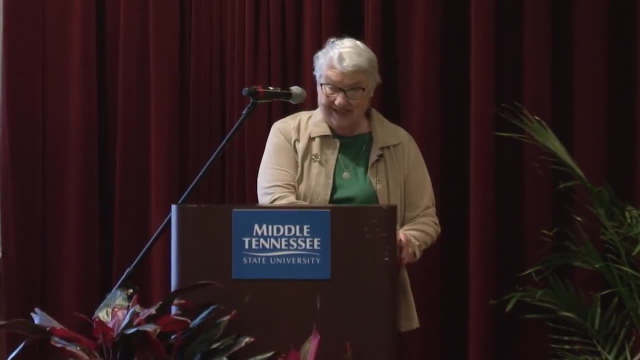 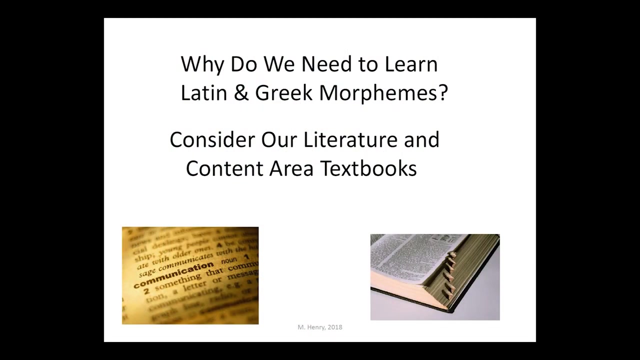 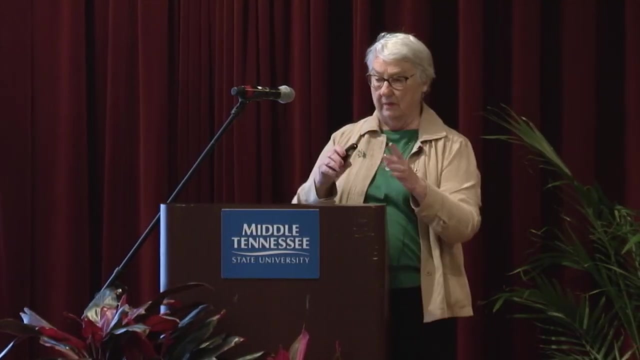 and above Most of you. it looks like Those are the kids that need the Latin and Greek morphemes, So hopefully you'll be able to get something from this. Now consider our literature and content area textbooks. I just opened the book Call of the Wild. 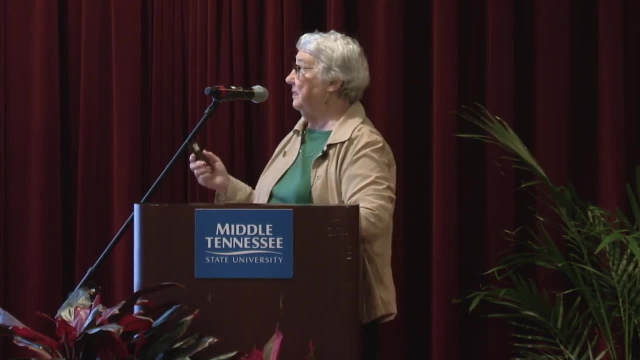 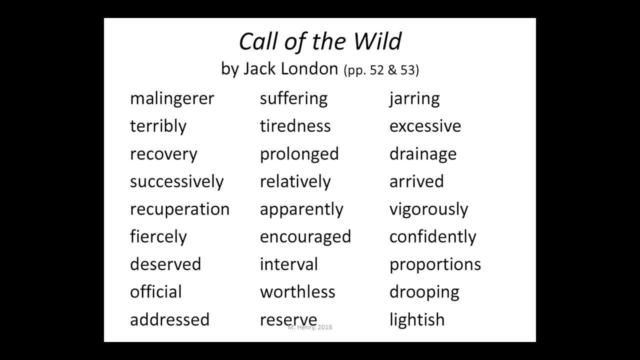 to. you know just any pages. And when you open it- page 52 and 53, here are words that the kids are reading. Now this is a sixth grade adoption. in California, All sixth graders have to read Call of the Wild. 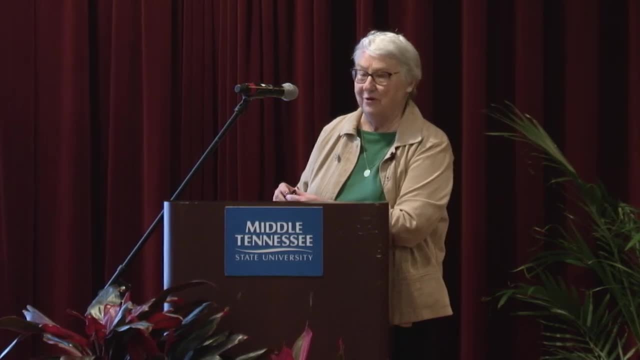 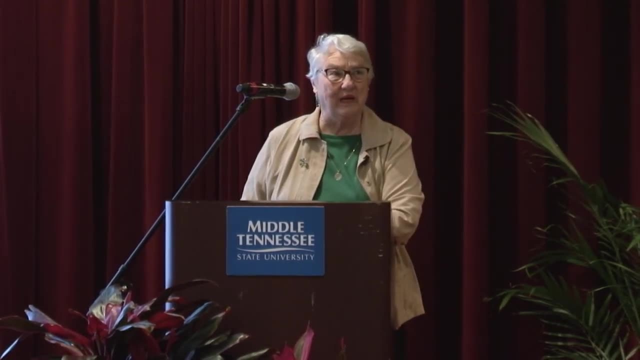 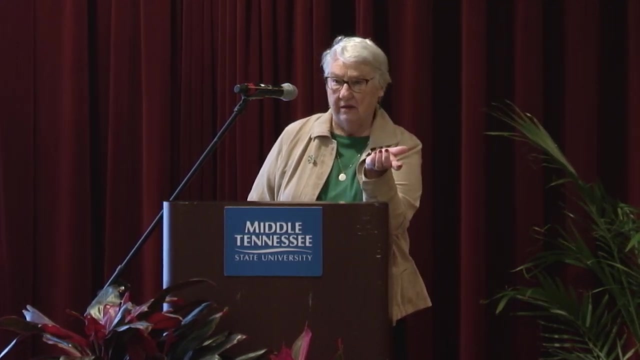 Jack London was from Oakland, California. Maybe that's why they have them read that. I don't know if you all remember the book, but it has a lot of French, Canadian dialect And they spell that out phonetically. So dis and dem and. 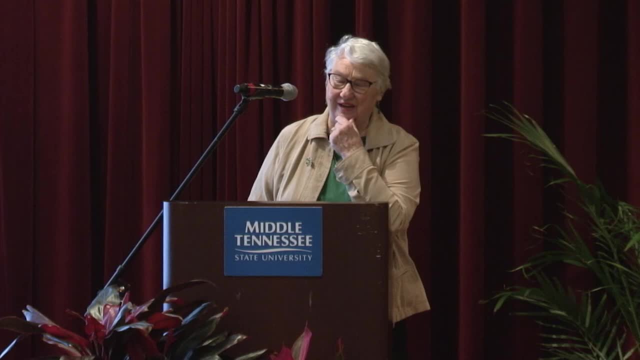 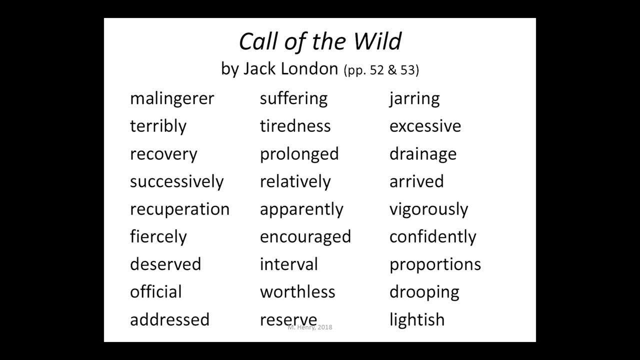 dose And it's very tricky for our kids who are struggling readers and writers. But look at these words: Malingerer, suffering, jarring, terribly tiredness, excessive recovery, prolonged. I just took some of the words that had prefixes and suffixes. 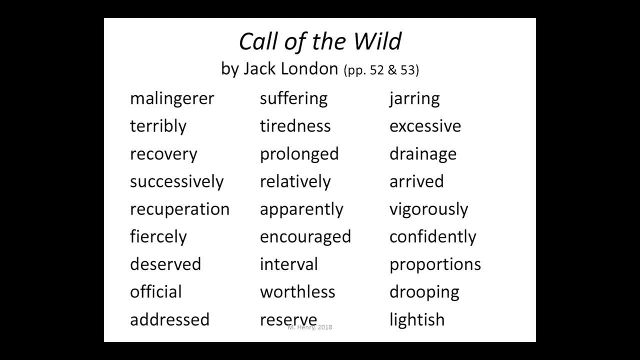 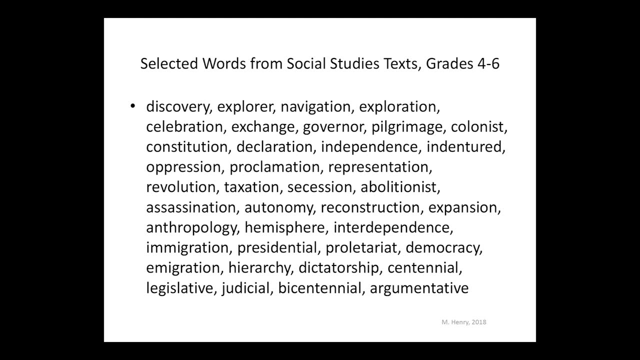 And I thought: wouldn't it be helpful for kids who could automatically recognize those prefixes and those suffixes? Here's some social studies, grades four through six. These are not high school textbooks. These are fourth through sixth grade. Discovery, explore, navigation, exploration. 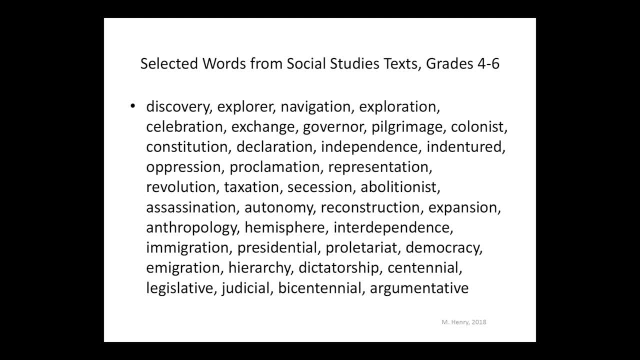 celebration, exchange, governor pilgrimage, colonists, constitution declaration, independence, indentured oppression, proclamation, representation, revelation, taxation. What if you'd never seen prefixes and suffixes, And some of these with the Latin word roots? 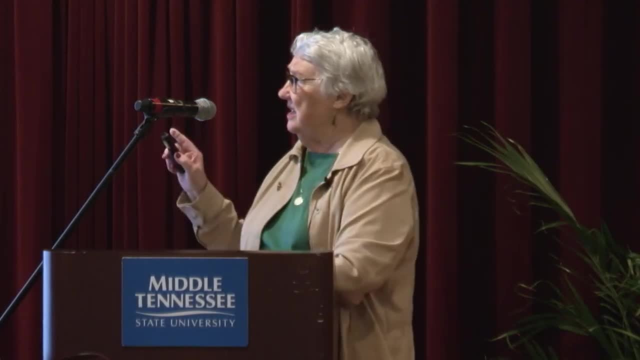 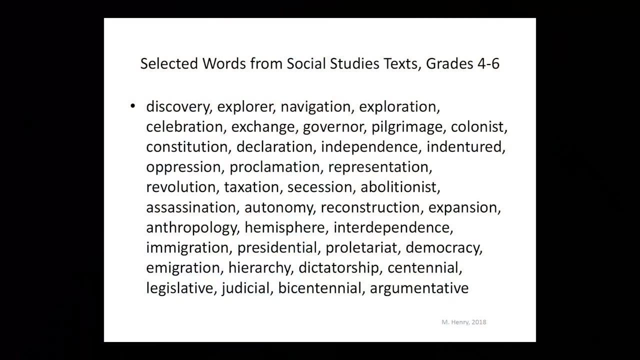 You'd have a terrible time because phonics isn't going to help you. If I try to sound out a long word like discovery, there's no way I can get discovery. I have to know. dis-cover- ee, Okay, Explorer Nav. 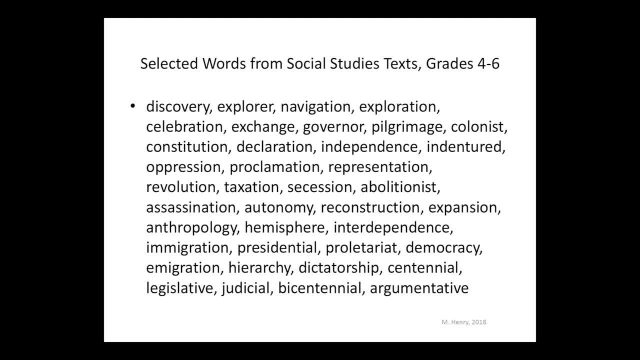 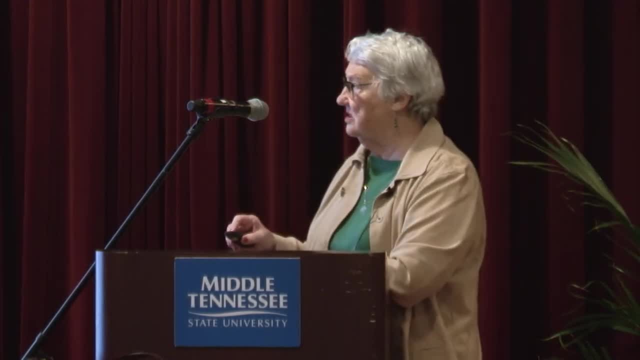 ee Gay Shun. I can sound it out by syllables if I can't recognize, but if I recognize shun right away, then I've got a lot of the word. So this is why we need to move kids ahead into this. Look at some of these. 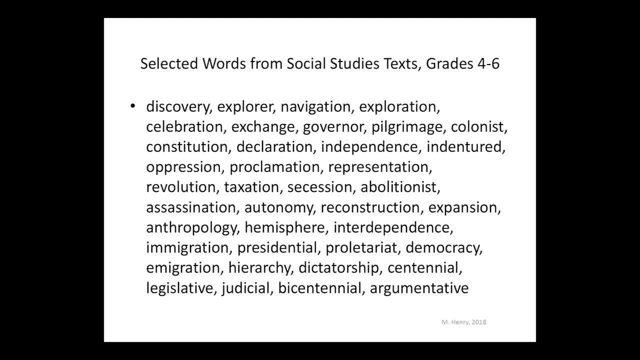 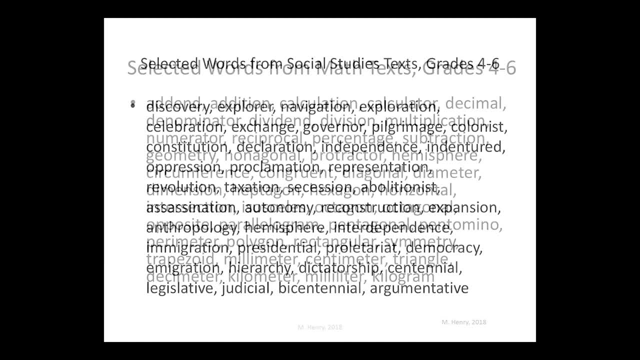 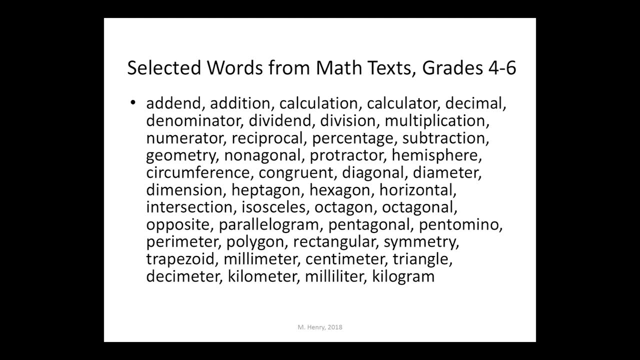 words towards the bottom: Assassination, anthropology, interdependence, proletariat, and so on. Look at math: Addend, Addition, Calculation, Calculator, Decimal denominator, and so on: Assosceles, Octagon, Octagonal, And so on. 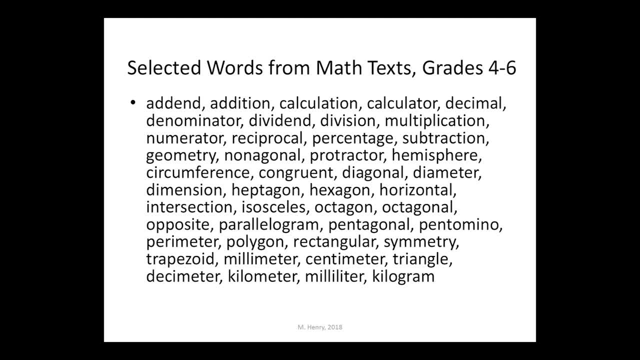 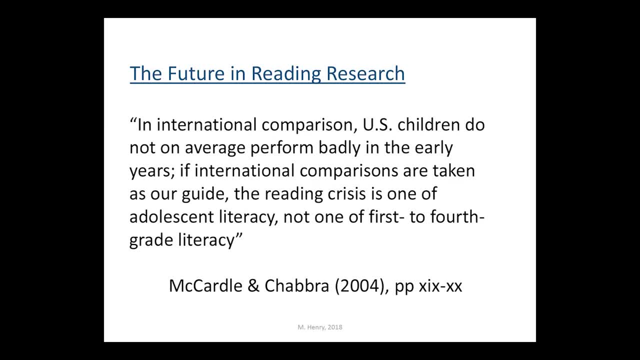 Pentagonal Pentomino: Perimeter, Centimeter, Millimeter And so on Milliliter. McArdle and Shabrai in a wonderful book say: in international comparison US children do not on average perform badly in the early years. 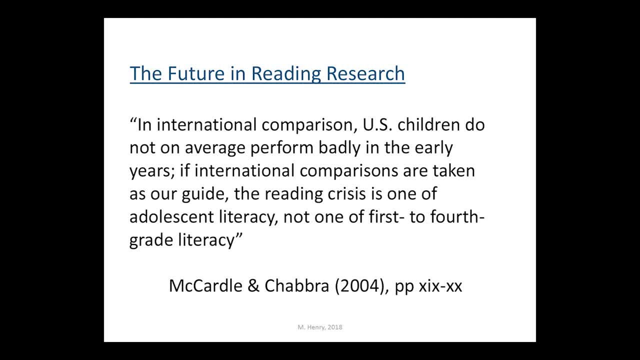 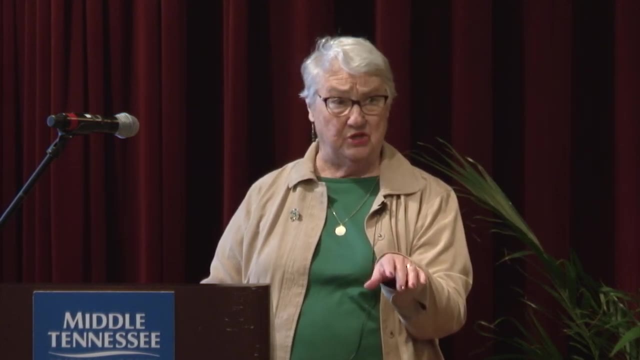 If international comparisons are taken as our guide, the reading crisis is one of adolescent literacy, not one of first to fourth grade literacy, And what we're finding is that, by eighth grade, the kids who scored on the NAEP- the National Assessment of Educational Progress- tests, who scored 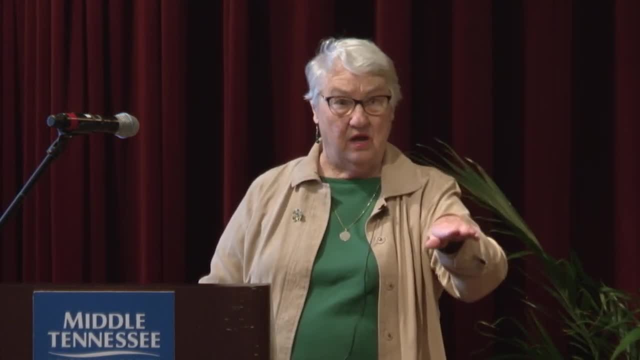 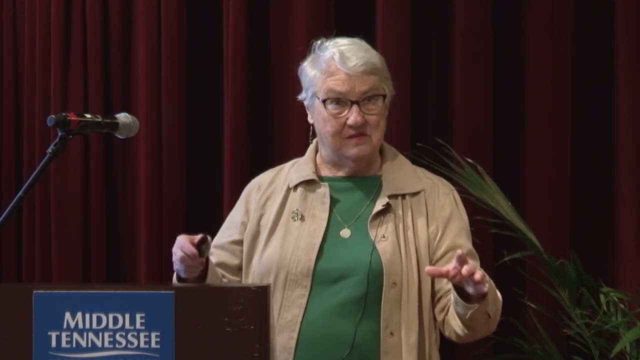 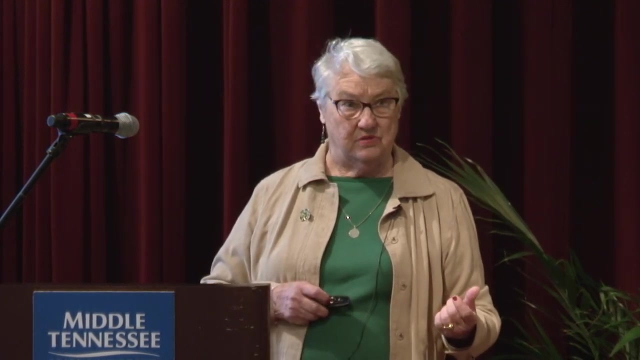 relatively okay in fourth grade, go down in eighth grade. I think a lot of it is that they don't get these words that are considered, you know, these longer words where they have to read beyond one and two syllables. Now I want to introduce you to Alan. 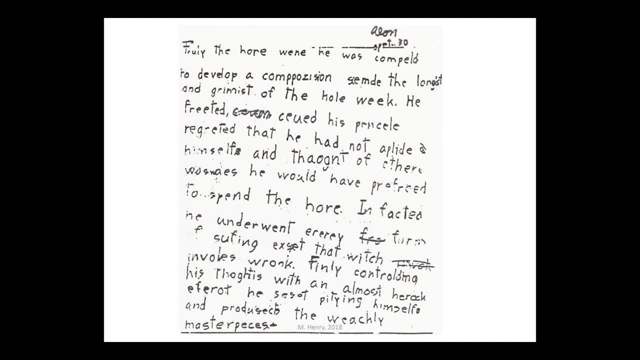 who is a 12 year old and he just finished. he finished sixth grade, he's going into seventh grade and he was asked. this is not his own paragraph, this is dictated to him by a clinical psychologist and she asked him to write in cursive: except going into seventh grade. 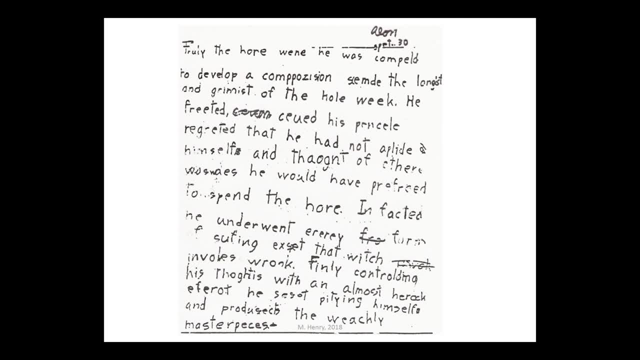 and he said: well, he tried his name Alan in cursive and he said I really can't write cursive, so she let him do the rest of his printing. He was asked to write the date, that's September 30th, and he immediately has that transposition. 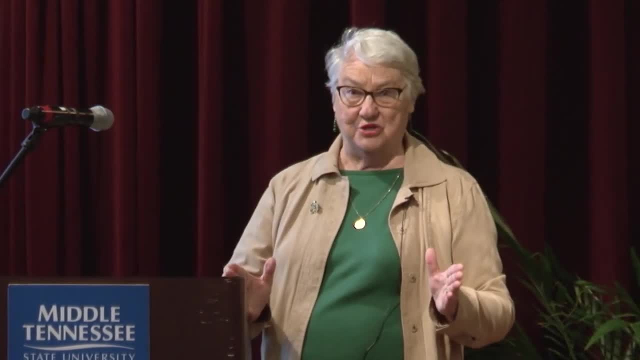 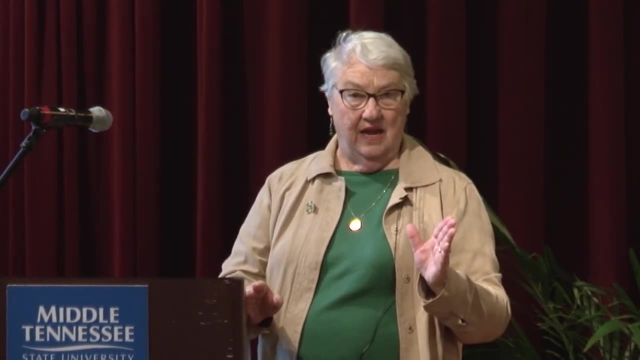 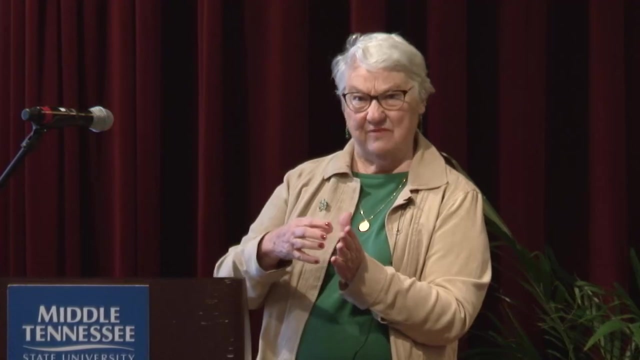 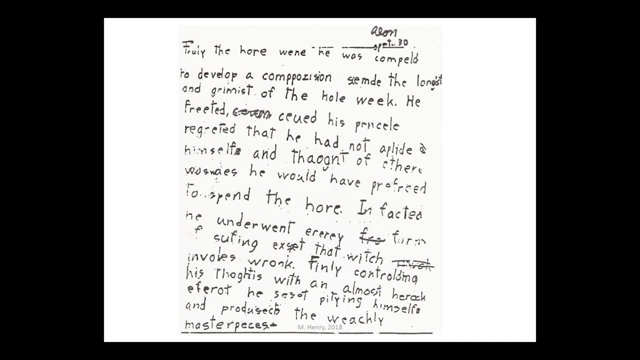 What I used to do was I would give this passage to my students at San Jose State and they had to find all the errors. what did those errors suggest for intervention? what did they have to teach the kids? now just try reading that by yourself for just a minute. 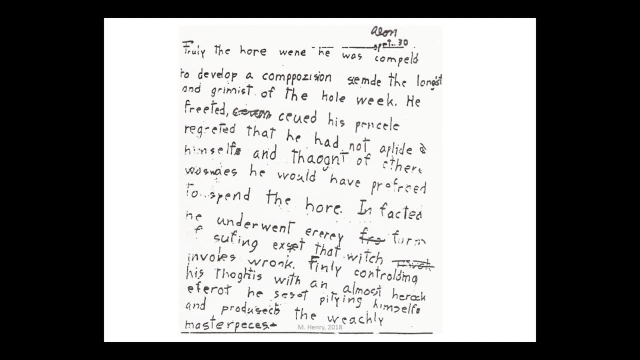 okay, so we have. let's try reading it together. I'll kind of conduct. okay, truly, the hour when he was compelled to develop a composition seemed the longest and grimmest of the whole week. he fretted, chewed his pencil, regretted that he had not. 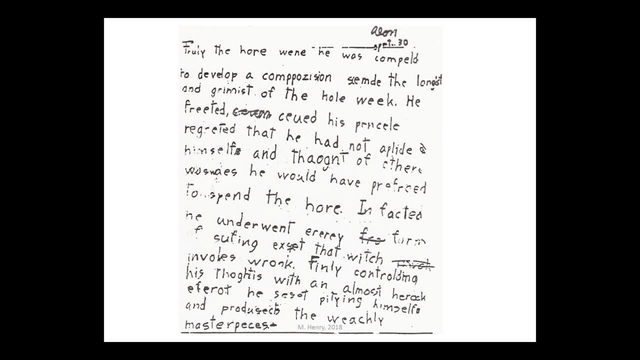 applied himself and thought of other ways he would have preferred to spend the hour. this is not about ladies of the evening. in fact, he underwent every form of suffering, except that which involves work, finally controlling his thoughts. with an almost heroic effort, he ceased pitying himself and produced. 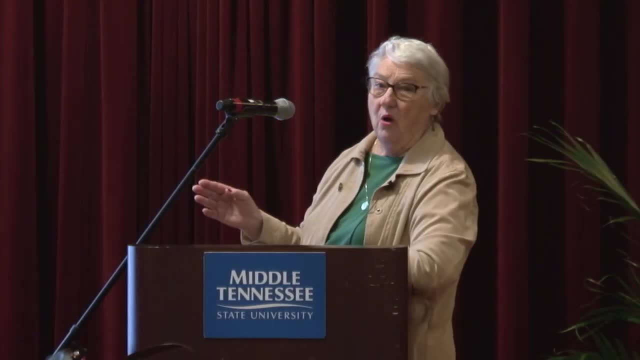 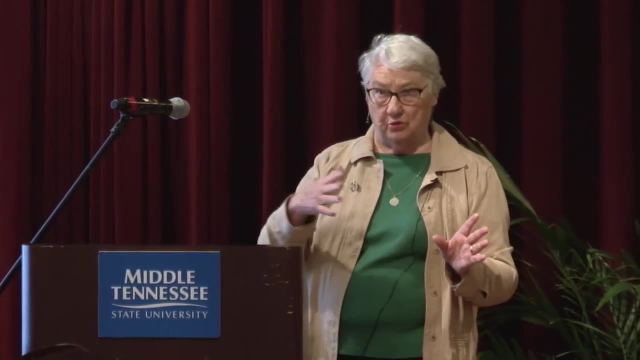 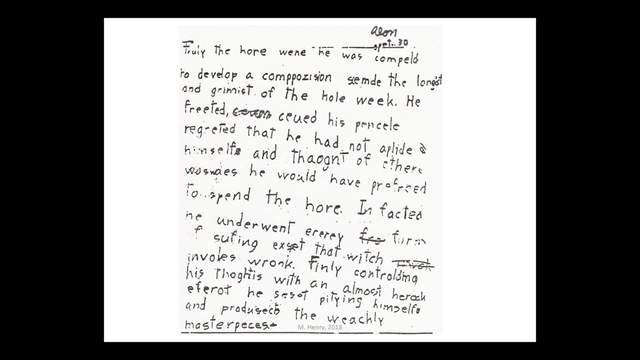 the weekly masterpiece. now, all of these words are within a seventh grade ability. if you're a good reader and dyslexic, notice the kinds of errors that he makes right away. take our and when um whole. many of these words are basic sight words that we're expecting. 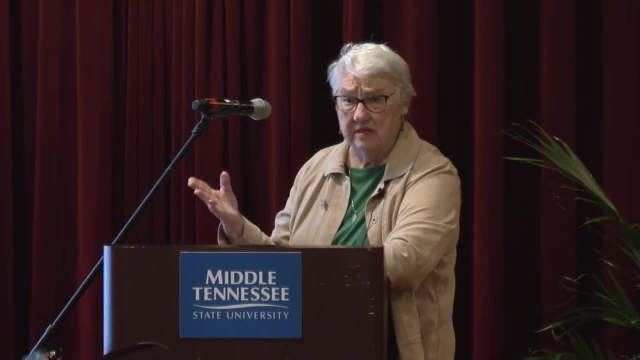 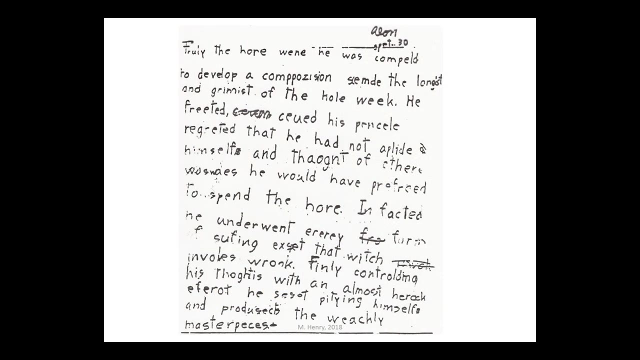 first and second graders to know, and Alan's now in seventh grade- um, what happens with composition? seemed longest grimmest. what is he missing? the suffix right he uses. um, look what he does for the past tense: ed in seemed. he writes d-e in fretted, he gets ed and he gets ed and chewed. 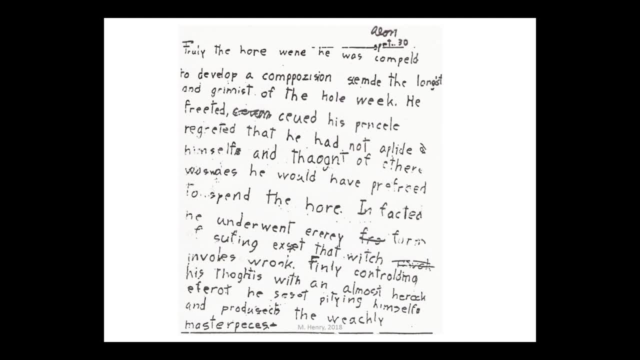 there's another one where he has the d oh compelled. he just has a plain d up there in the top line, so he doesn't know that that's consistent, that that ed is always the past tense. look what he does with longest and grimmest. uh, when do i use ist? think of a couple words that end in ist. 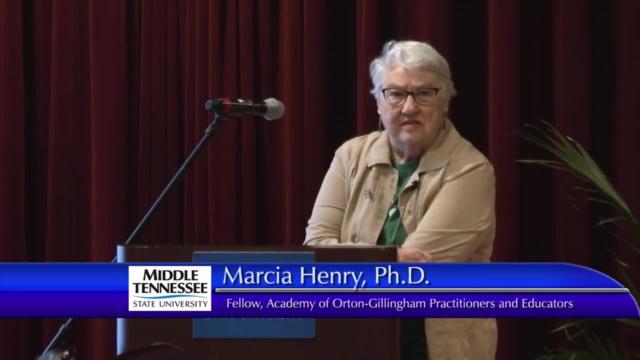 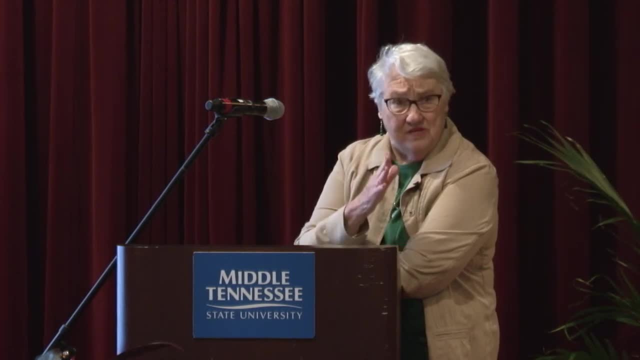 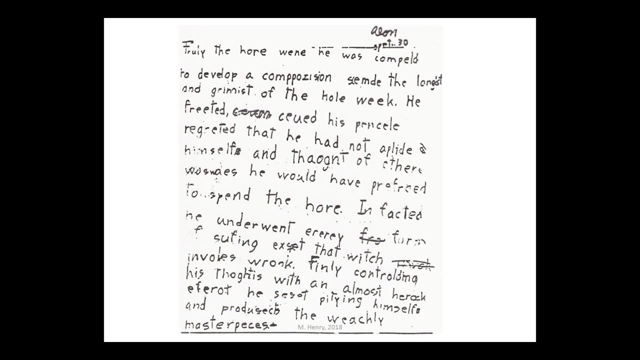 like dentist, scientist, chemist, pianist, all people, all noun people. IST is always a noun person. EST is the superlative degree of the adjective and so longest and grimmest have to use EST. he doesn't know to double the m in: uh, grimmest, uh, fretted. you can see he has. 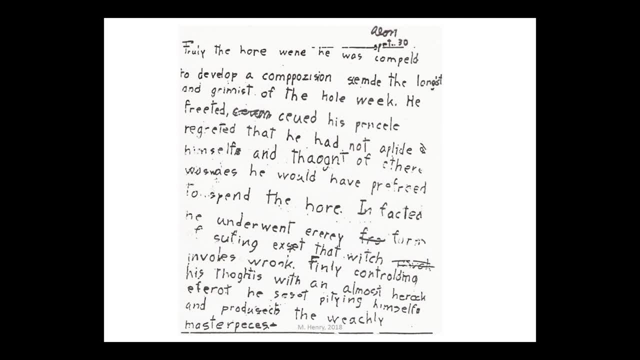 frenzied, Freeted, chewed, He doesn't get the ch. So some basic phonics kinds of errors, Thought, who knows where the A came from. Look at other ways. First he spells it was and then W-A-E-S. 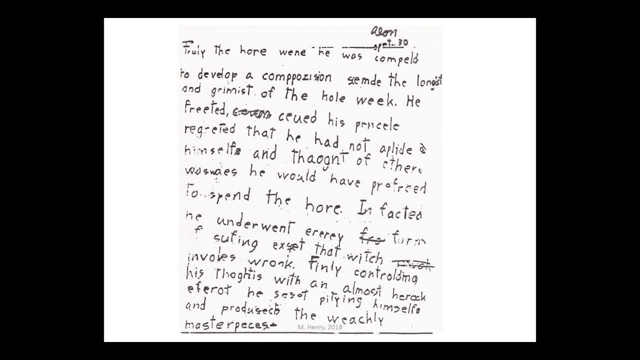 So again, one of those basic sight words that we would expect first and second graders to know Every suffing, instead of suffering. This is a fairly typical error with older dyslexic children. They tend to leave out that middle syllable. 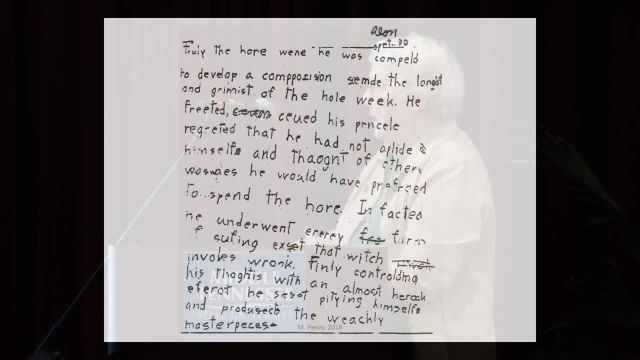 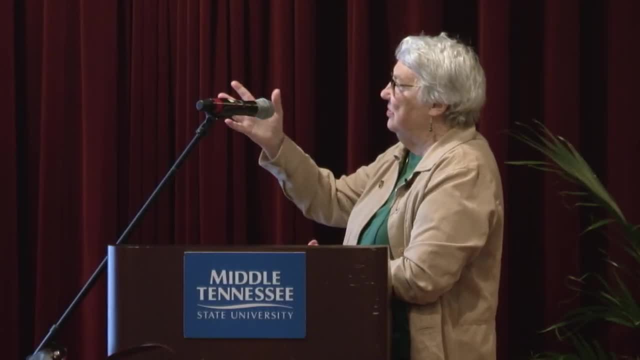 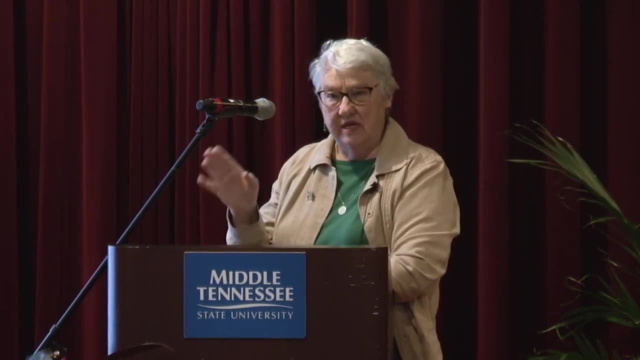 They're not really thinking in terms of syllables, except that which involves work, those basic sight words again. So you can see a lot of the errors. Now what's fascinating- and this is the interesting thing about Alan- is he is not your typical 7th grade kid. 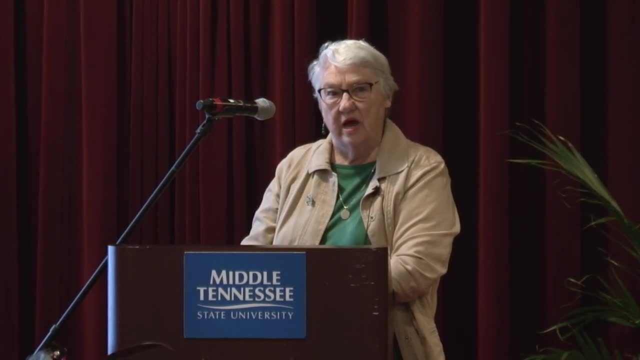 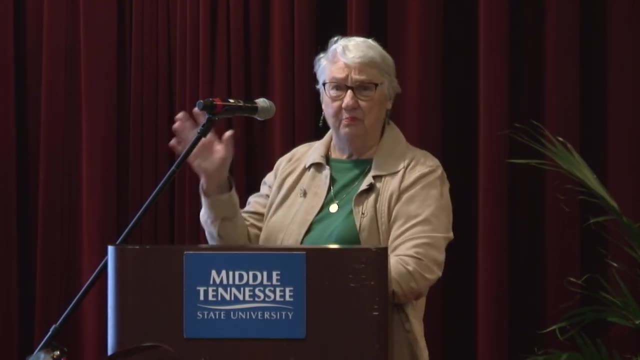 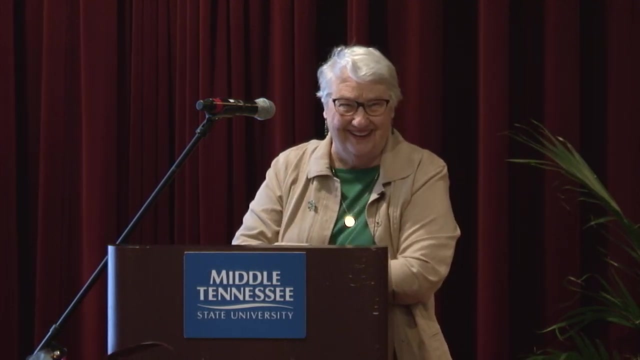 On a Stanford-Binet individual IQ test, he scored 172.. Now, that's genius level. So here's this brilliant kid. Now, at 11.29,, I'll tell you the end of his story. It has a really interesting ending about him. It has a really interesting ending about what Alan is doing today. But this was Alan and he got better because he was taught the structure of English words. He was taught all the common Latin and Greek roots and all of the corresponding prefixes and suffixes. 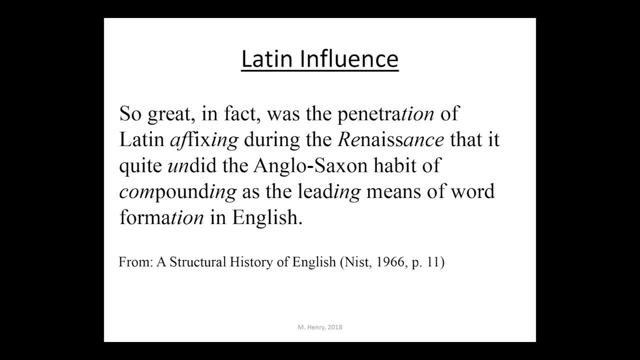 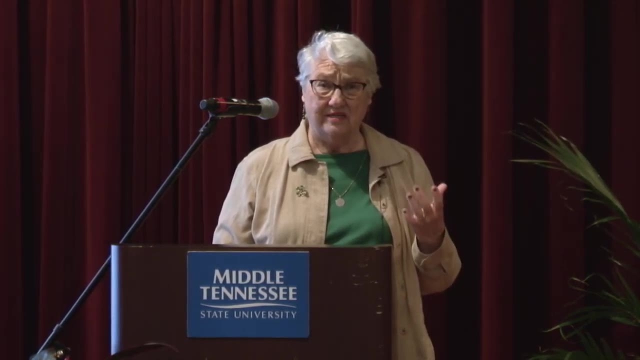 Now what happens with the Latin? remember that three-way matrix. the letter-sound correspondences are pretty much the same. Fortunately, in Latin there aren't very many roots with vowel digraphs. They're generally short vowels: spect, rupt, struct, dict and so on. 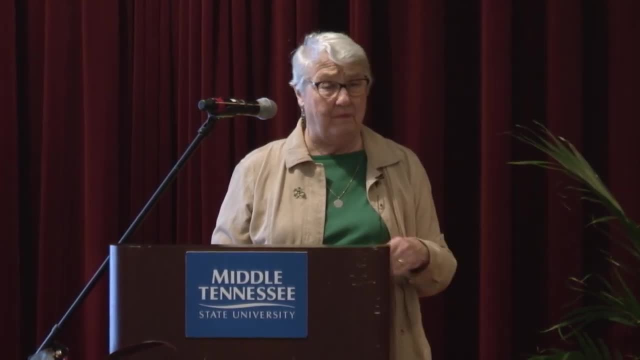 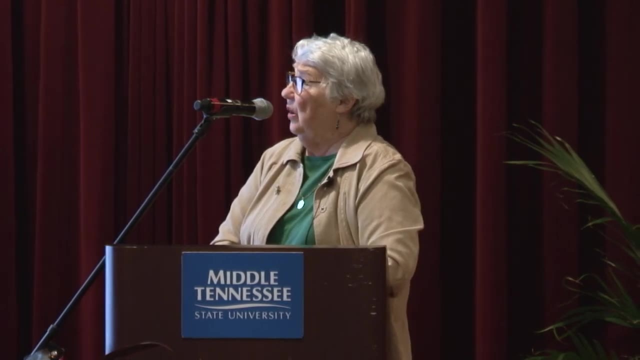 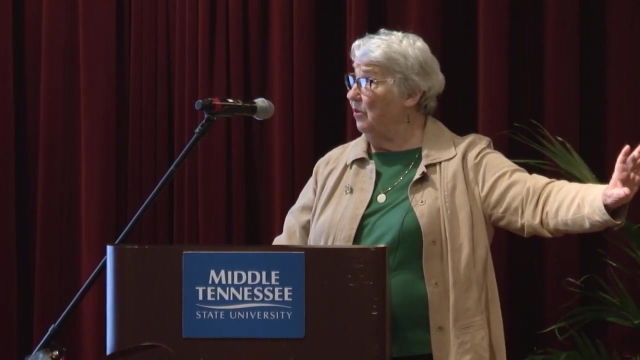 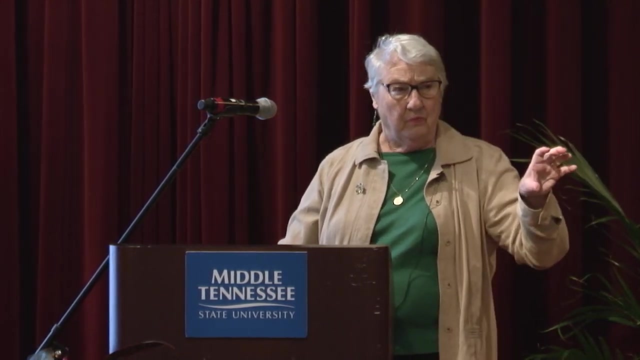 Some have vowel consonant E, like scribe, but most of them just have a short vowel. Fillable division is pretty much the same And with the morpheme patterns we don't compound very often. We occasionally do, But we tend to only affix. 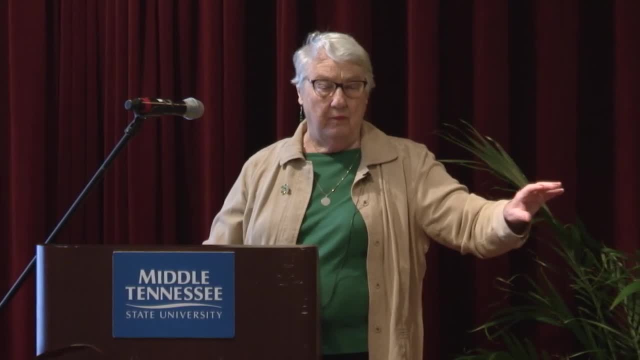 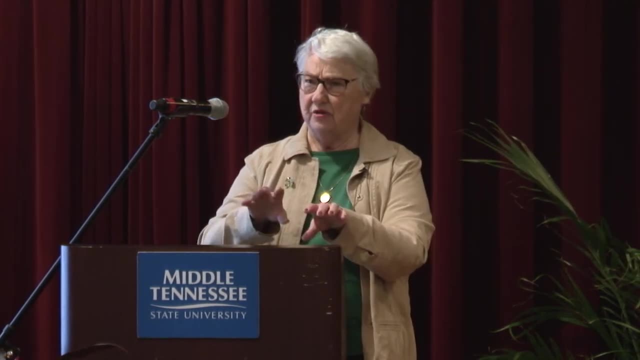 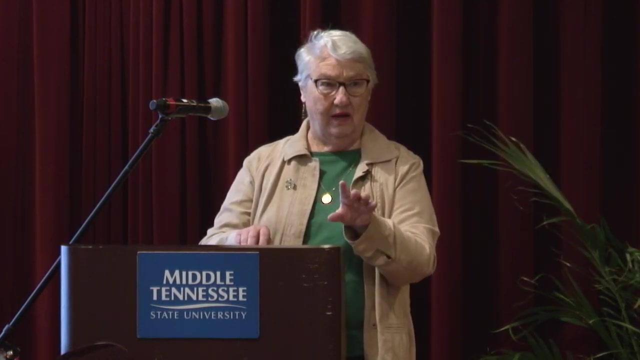 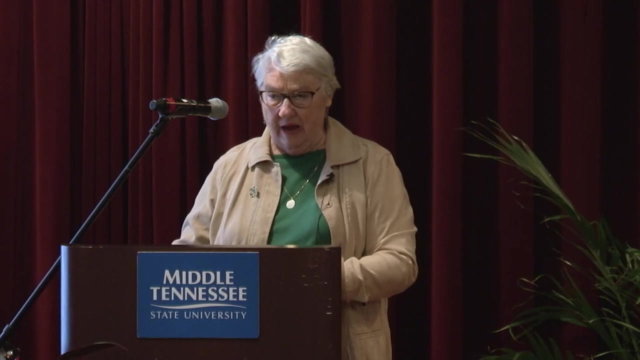 I should say usually affix. We don't compound like struct, dict, Spect, rupt no, But I have spect inspect inspector, respect, respectful, respectfully. I have to tell you kind of an interesting story I was asked by. this was years ago. 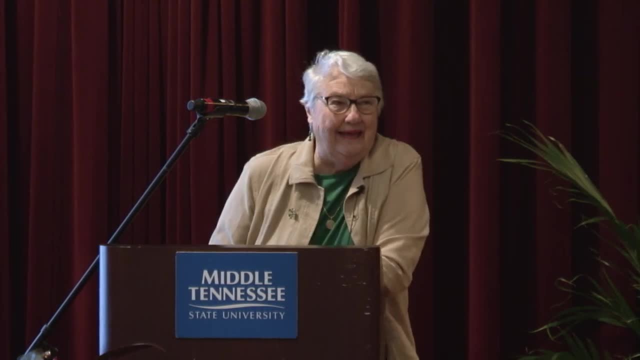 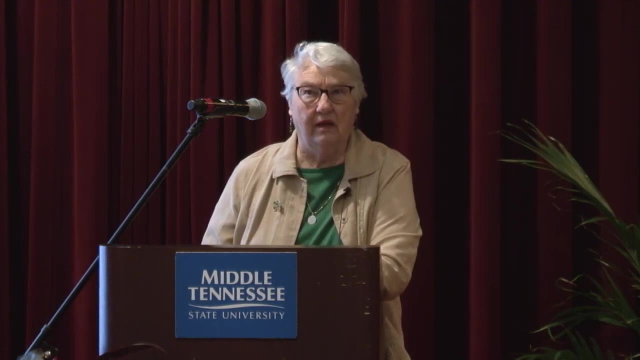 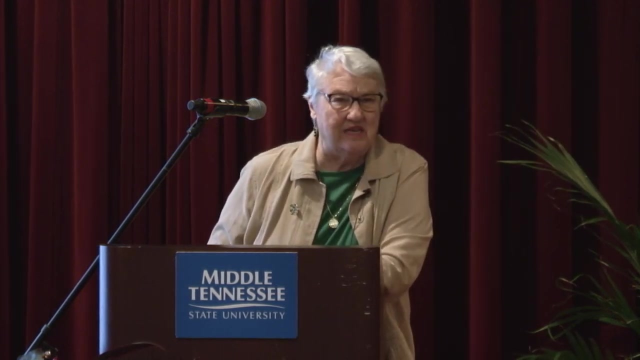 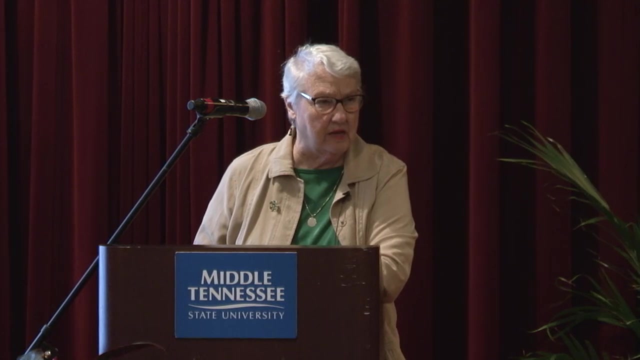 about 1985, I was asked to speak at the capital IDA capital capital branch, or I think it was called something like that. It was in Washington DC And they had an adult literacy group. Mostly these were young people in their 20s, I'd say. 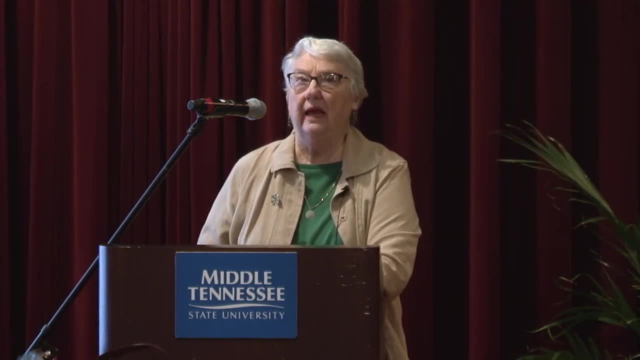 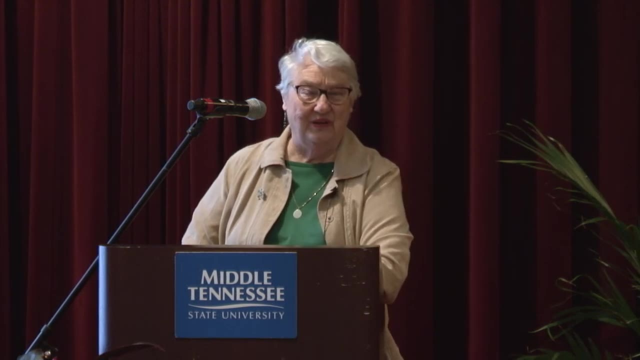 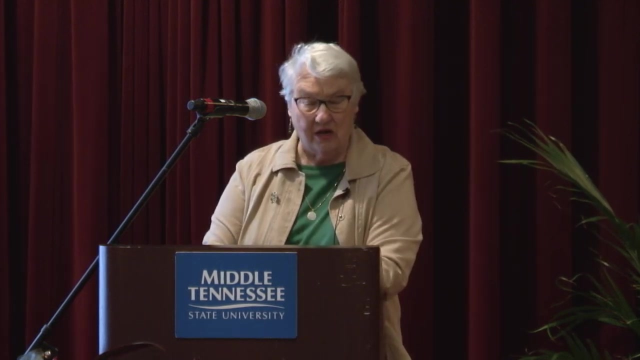 Most were men And I was asked to speak at their awards banquet. They had some banquet, So I can't remember the name of the branch president, but anyway she asked me if I would talk about Latin word roots. as you know, the dinner speaker. 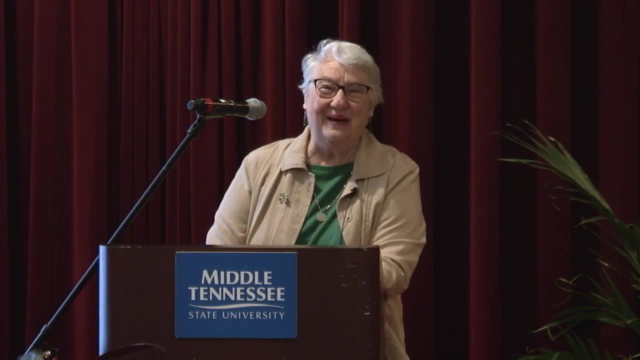 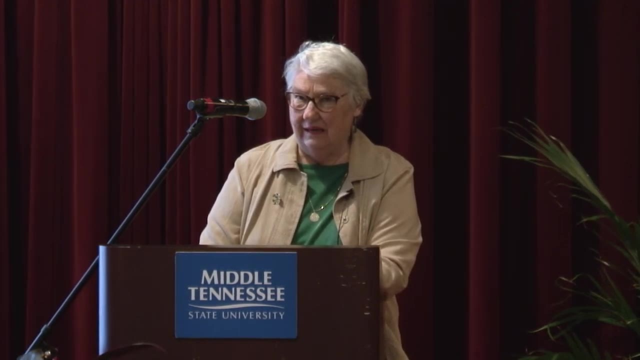 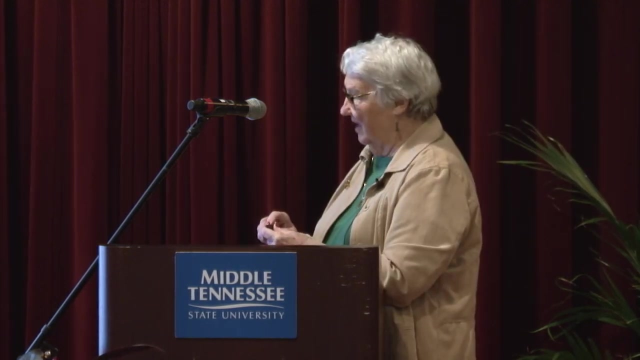 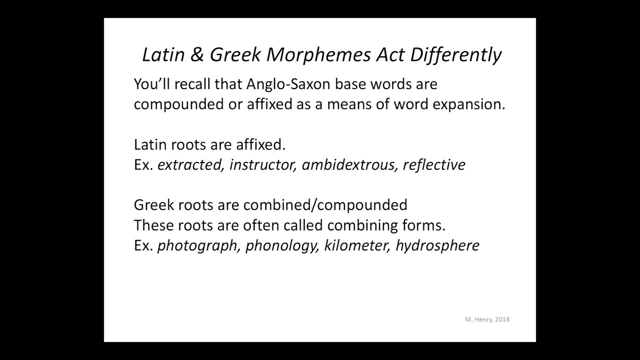 And I thought: oh how fascinating. But I did, And I had them do a web on struct And I think I have that in a minute. Well, let me hold that story a minute And we'll see Anglo-Saxon base words: compound or affix. 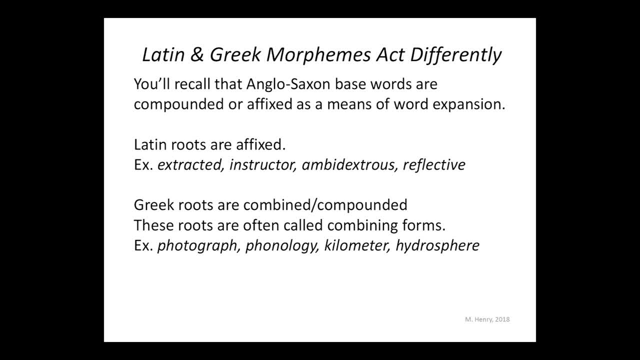 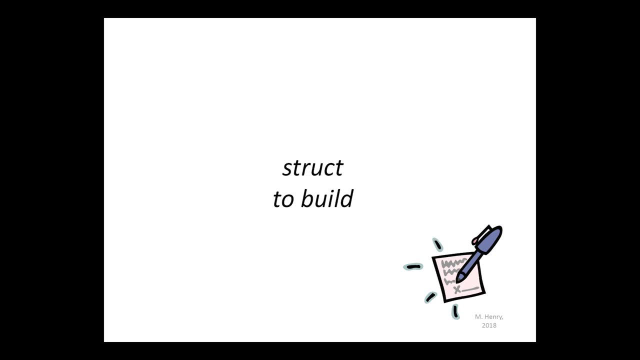 Latin affix, And you're going to find out that Greeks, the Greek roots, generally compound. again, They don't affix as much I wanted as long as I started that story, Okay. So I had them all. they all had a piece of paper. 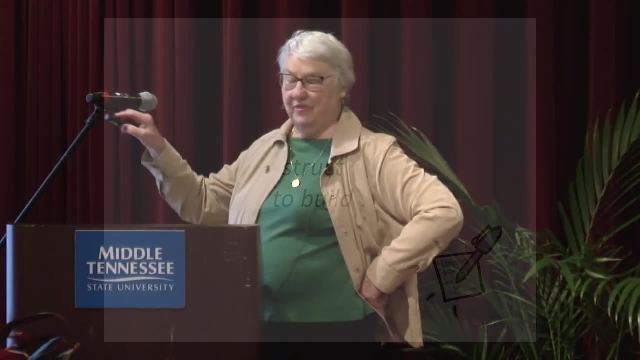 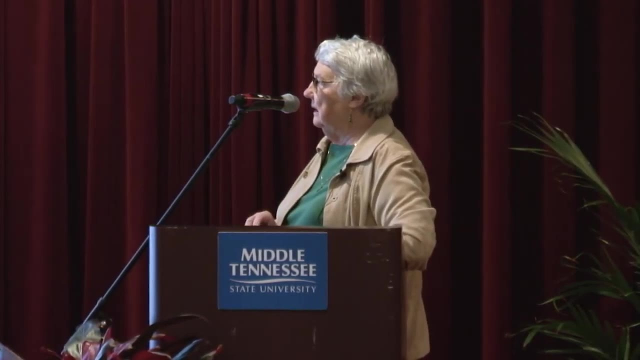 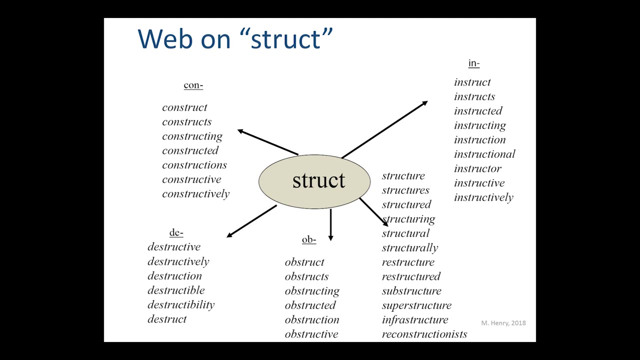 And they could just brainstorm at their table the various words that they came up with, And so they came up with something like this. So here were a bunch of words with the prefix con, with dee, with ob, with in, and then all of these other ones. 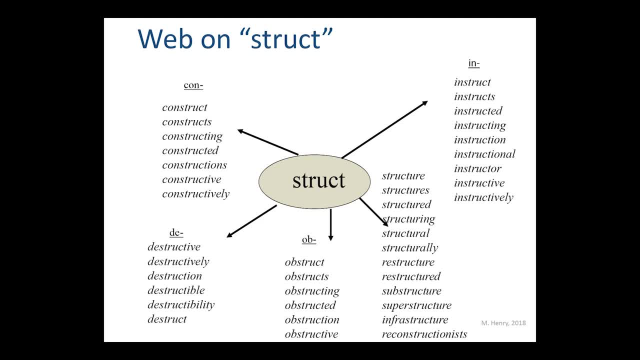 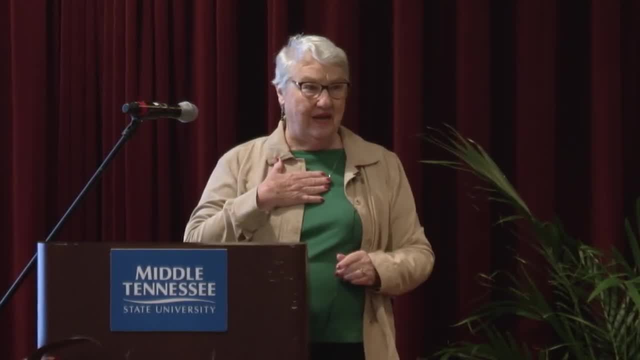 And after the meeting, this young man came up to me and he said: I'm so mad. Well, I thought, what did I do? How did I offend him? And he said: I said, well, can I help you? 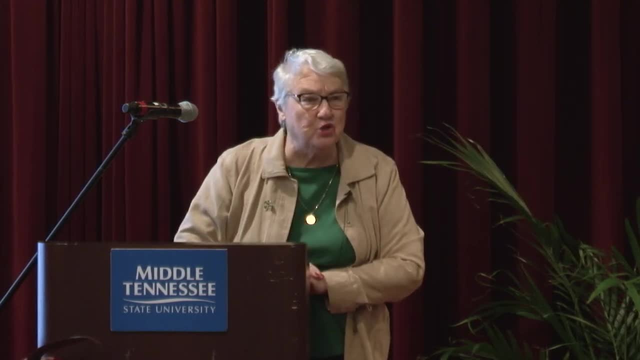 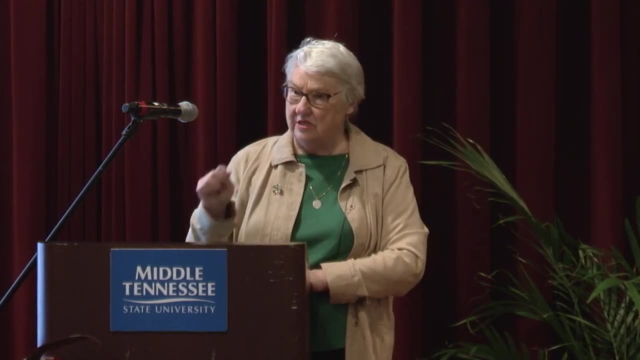 How can I help you? And he said: I'm so mad. They never told me. And I said: what didn't they tell you? Although I knew what he meant, They never told me that all I had to do was take this root. 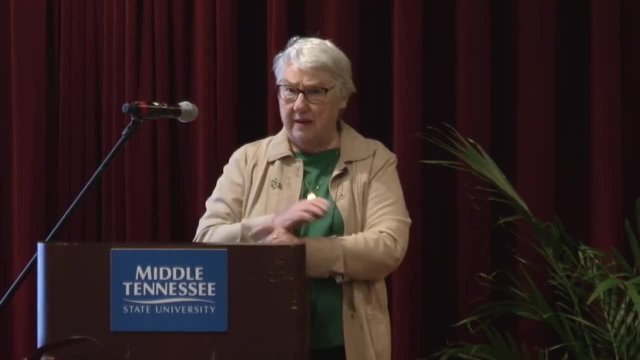 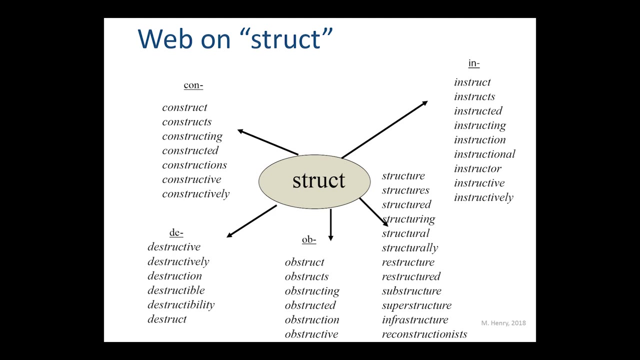 and add these prefixes and suffixes, And I could make long words. Now you and I know that all of these are related. We know that all of these have something to do with building. We can figure out the meaning. It's a beautiful structure. 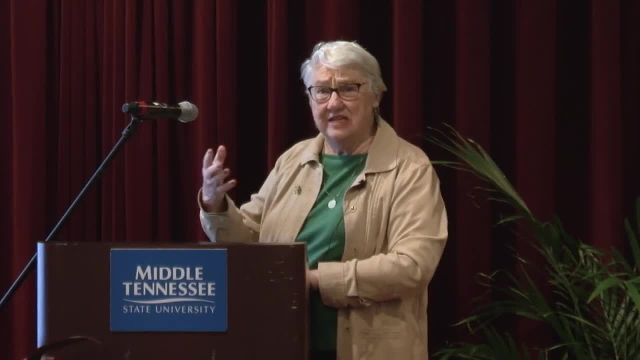 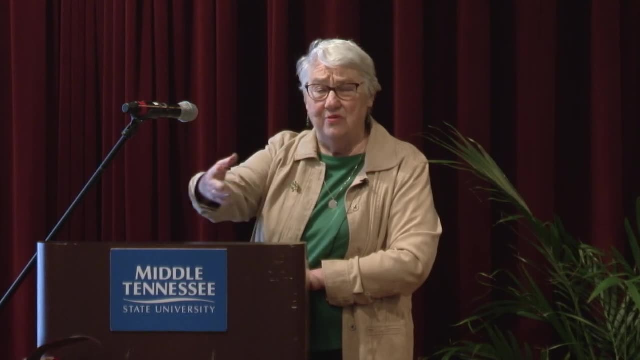 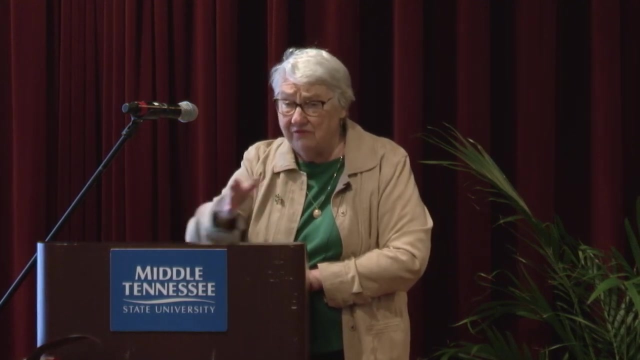 It's a beautiful building. If I reconstruct something, I build it again. After the Civil War, who came down this way? The Reconstructionists. Just by adding all those suffixes, I get that long, long word. Okay, I just wanted to talk a little bit more. 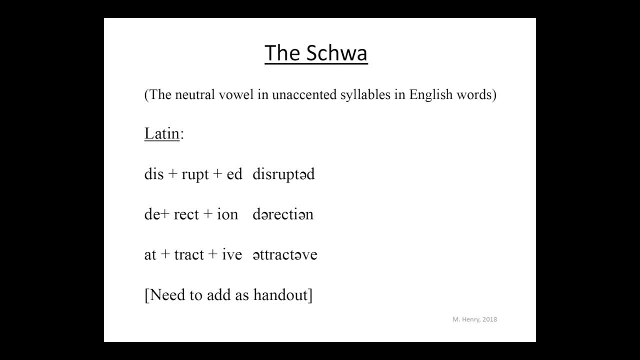 about that schwa Here in the Latin base word I have rupt. That's generally going to get the accent, So I have disrupted Direction D, Direction Ut At Tra Trac Iv. So I need to know. 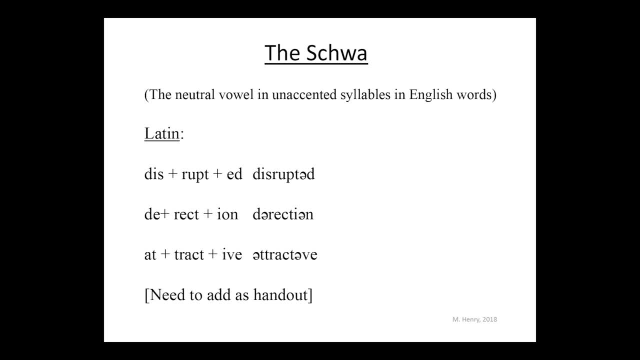 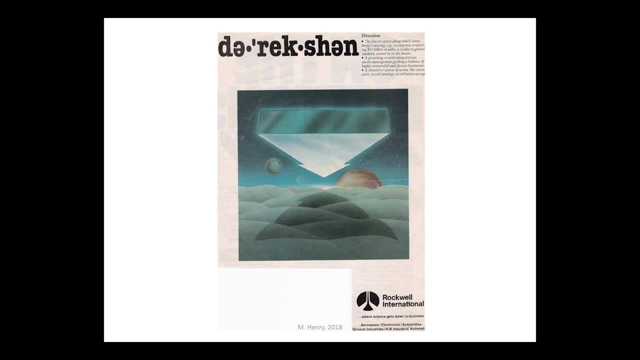 that I-V-E doesn't say Ive, It says Iv, Attractive Elective And so on. This was an old Rockwell International. I don't even know that. I don't think that company exists anymore. Direction is how they show the dictionary. 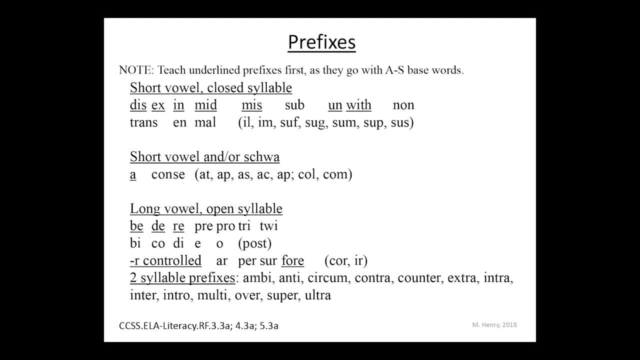 Here are the prefixes, The ones that are underlined we teach first because those are the ones that go with the Anglo-Saxon base words: The long vowel, open syllable prefixes, the R-controlled prefixes, and then we have some two syllable prefixes. 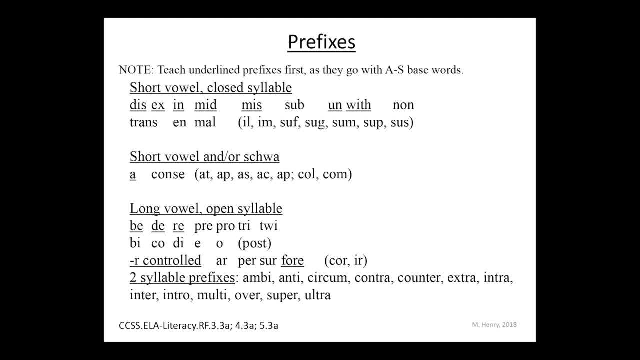 Ambit, Anti Circum, Contra Counter, Extra Intra, And so on. Most of these that are not underlined are usually found with the Latin word roots And, again, they all have specific meaning. Now, one of the things that we have to: 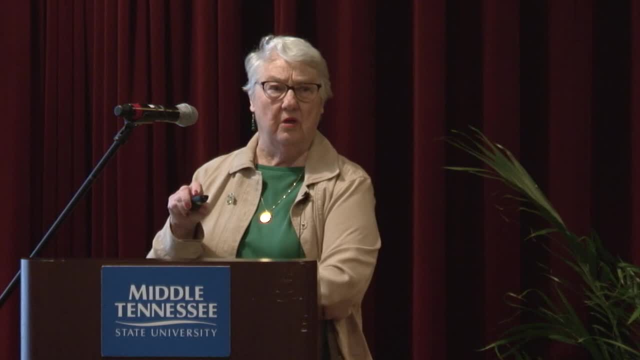 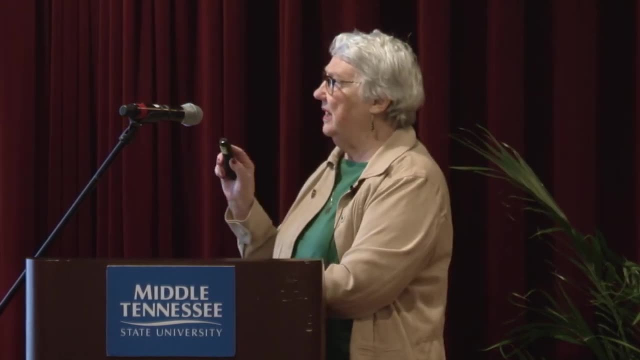 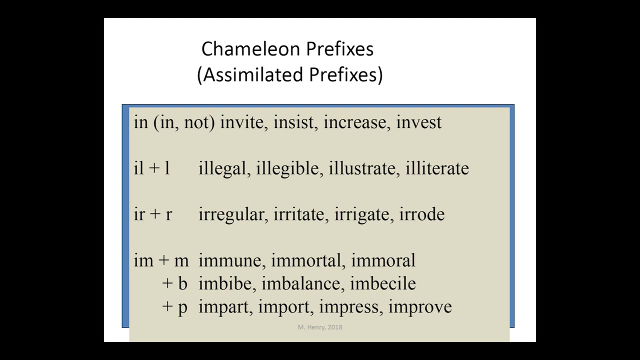 especially with older students. are any of you working with middle school, high school, Good, With those older students? we want to get into what my mentor, Paula Rome, called chameleon prefixes And linguists would call those assimilated prefixes. 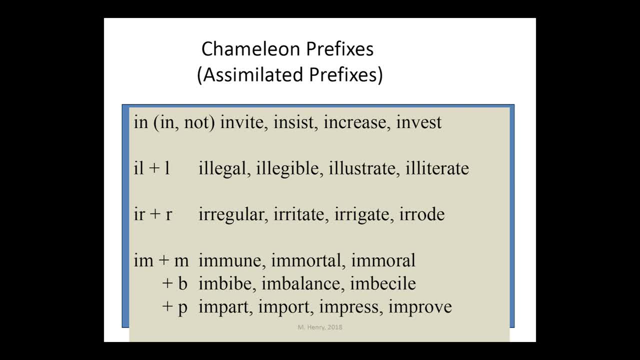 Take in meaning in or not. We change the N to an L if the root begins with an L. I don't say something is in-legal or in-legible, I say ill. We change the N to an R if the root begins with an R. 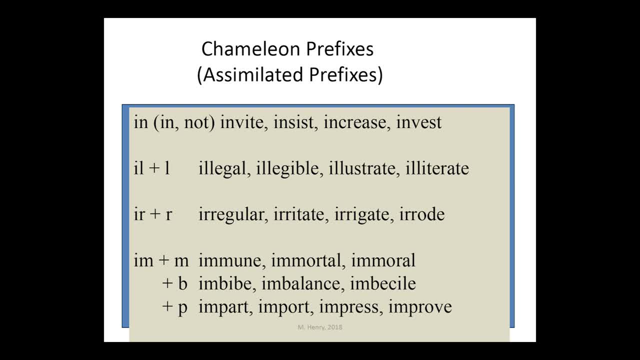 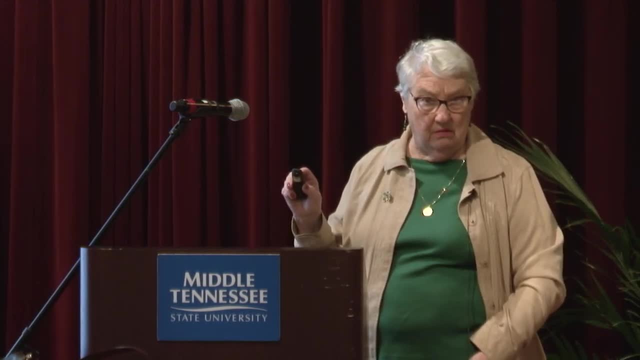 Irregular, Irritate, Irrigate, Erode, And we change the N to an M, with the root begins with M, B or P. Now, this is not so hard for decoding, but it is harder for spelling. That's why you have to point these out. 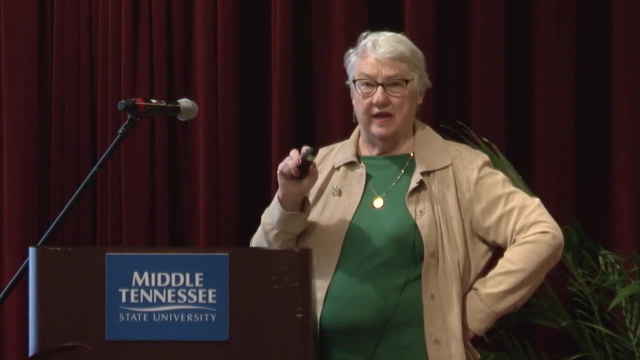 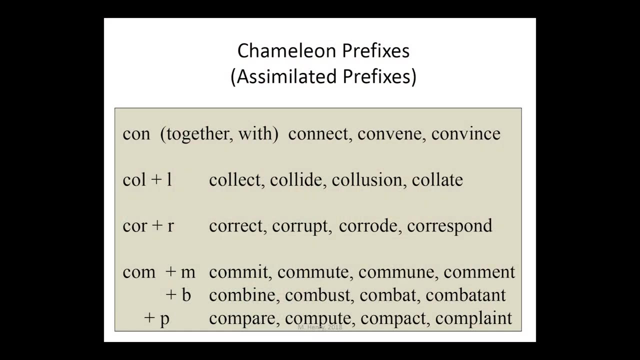 because chances are they'll end up with just one L in illegal. They may not hear both those Ls. Same thing happens with C-O-N, Con, Connect, Convene, Convince, Meaning together, or with We change the N to an L. 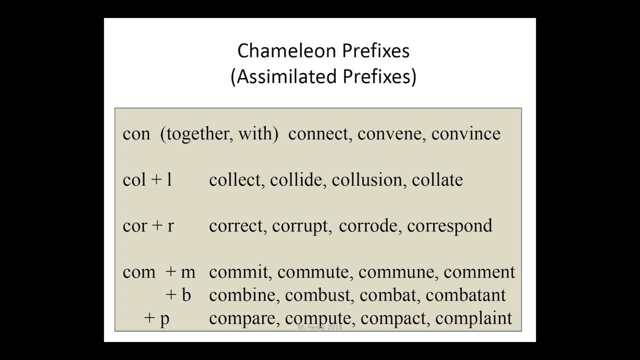 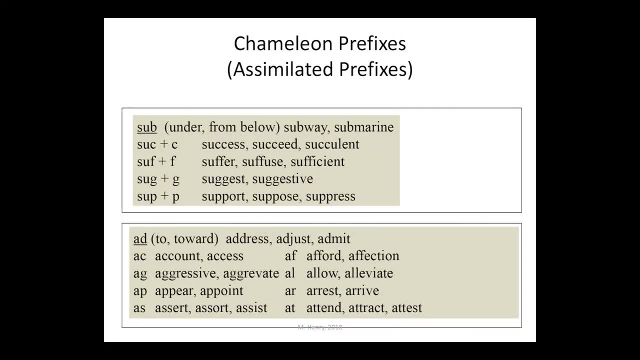 if the root begins with an L, To an R before an R And to an M before M, B and P. Same thing happens- Not exactly the same, but we have chameleon prefixes for sub if the root begins with a C. 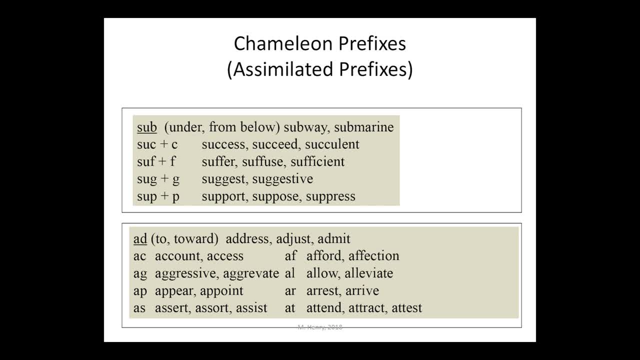 that B becomes a C. Success Before an F, it's an F, and a G and a P, And then add meaning to or toward. has eight different variants, what we call variants Account Aggressive Apparent. 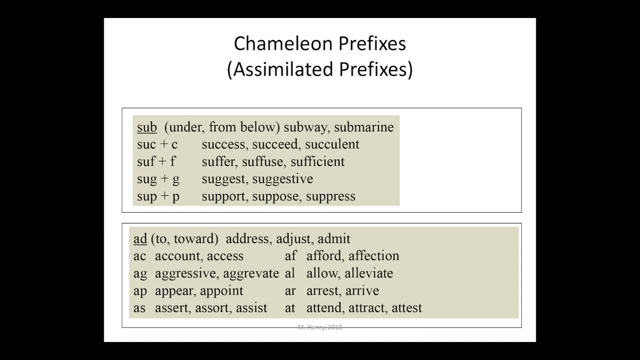 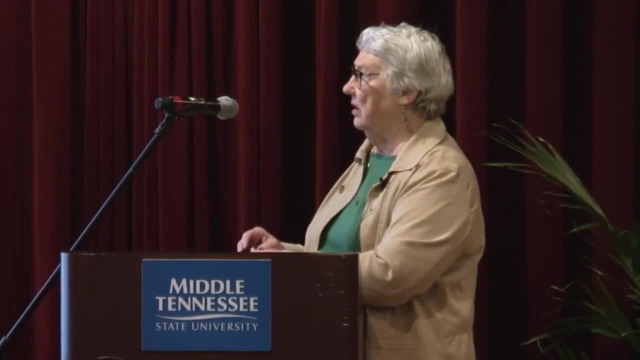 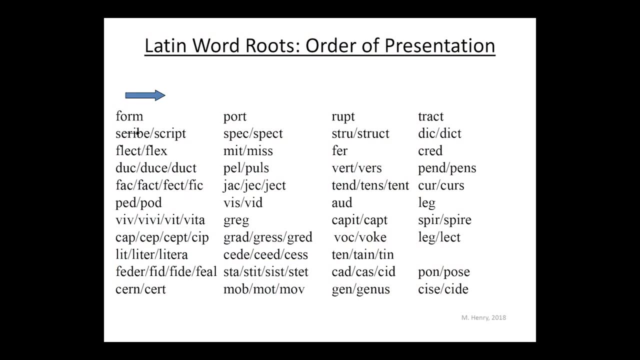 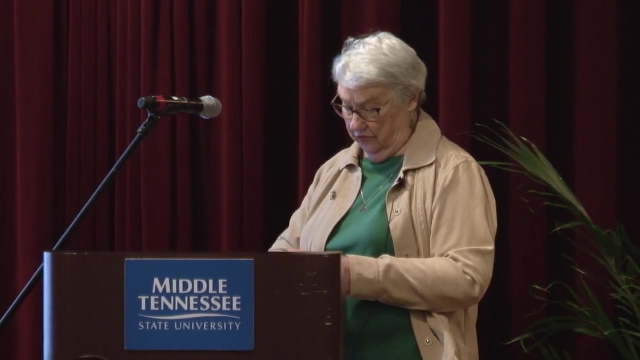 Assert, Afford, Allow, Arrest, Attend. So these are just some of the things that you need to know about because it may come up Now. here's the order that I give the Latin word roots in And I make cards for the Latin word roots as well. 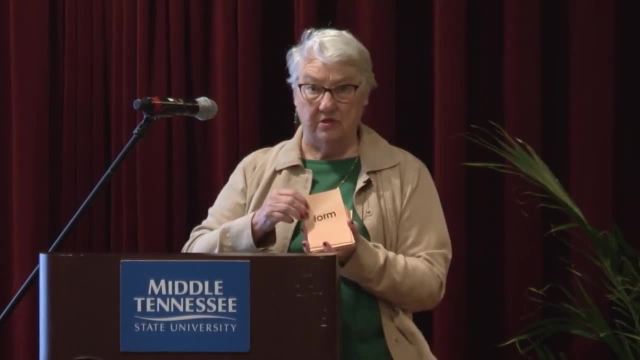 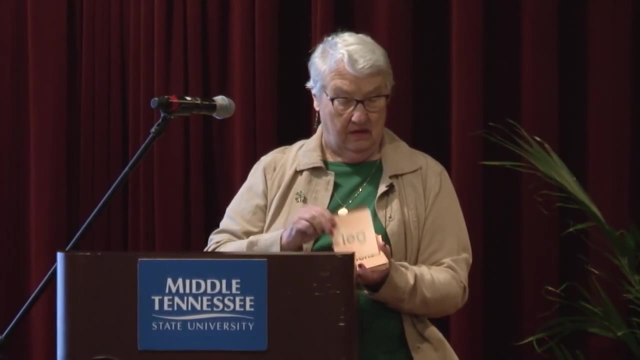 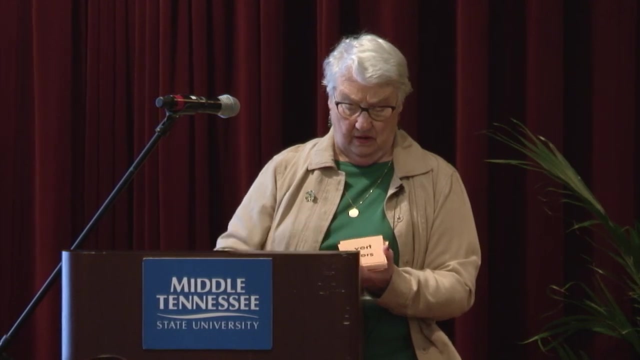 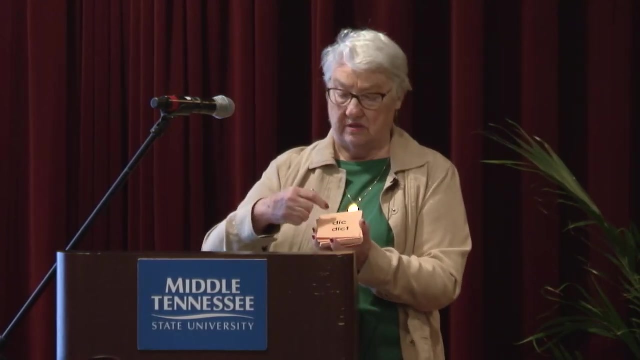 So I want them all to be able to just automatically know what these say and what the meaning is, Because all of these have very specific meaning, But, notice, most of them have. well, this has are controlled, but most will just have a short vowel. 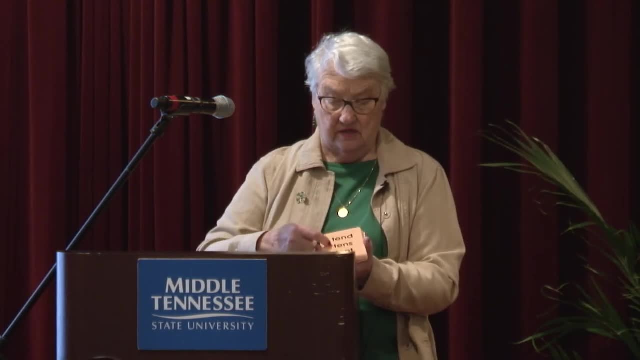 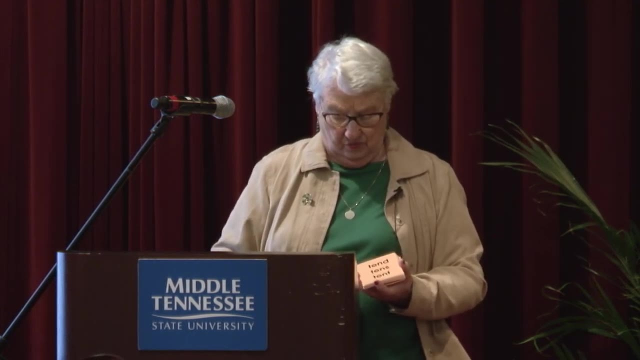 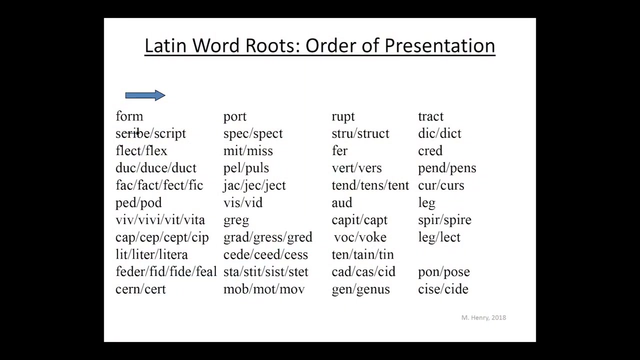 Dic and dict, Vis and vid, Tend, tense tent. So we don't have. we have very few that have vowel digraphs, which are more problematic, So we'll just leave that for our students. I give form port rupt and tract first. 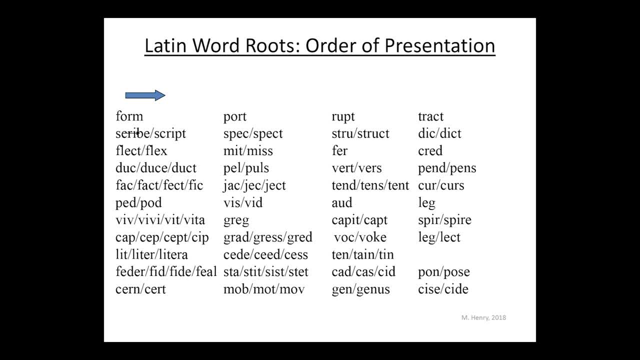 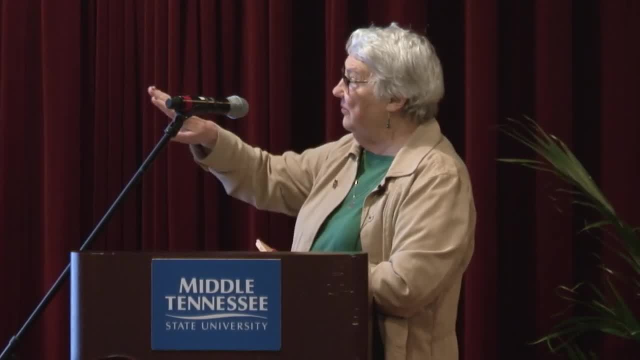 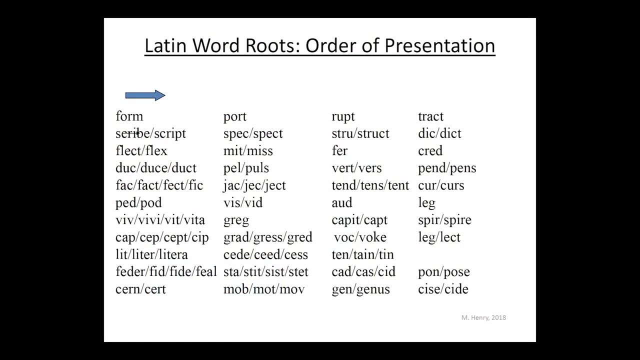 mainly because they're among the most frequently used and they have only one form. Now we have quite a few that we. we have what we call twin bases. We have scribe, script, spec, spect, strew, struct, dic, dict. 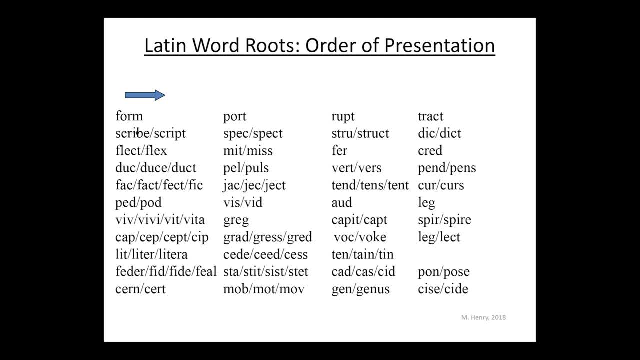 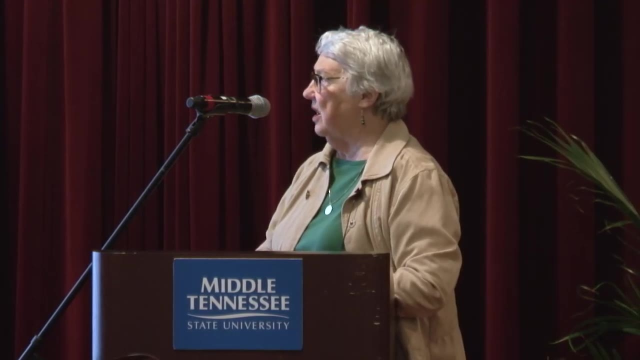 flect, flex and so on. Some have even three forms or four forms, Those I generally present later In the Unlocking Literacy book. these are among the first ones taught and then in the last chapter, I think, the more advanced chapter. 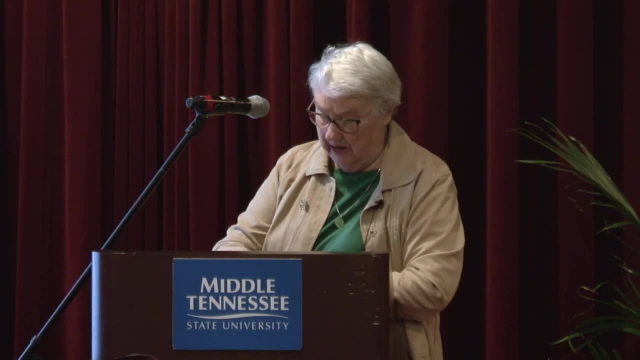 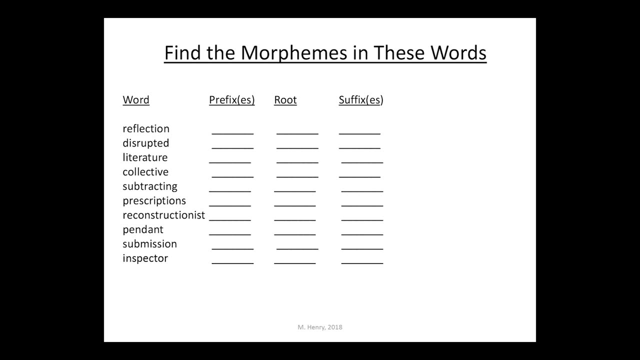 I have less common Latin word roots. I don't have that on this chart. Now let's see if we can do some of these together. Find the morphemes in these words. What's the prefix in reflection? How about the root? 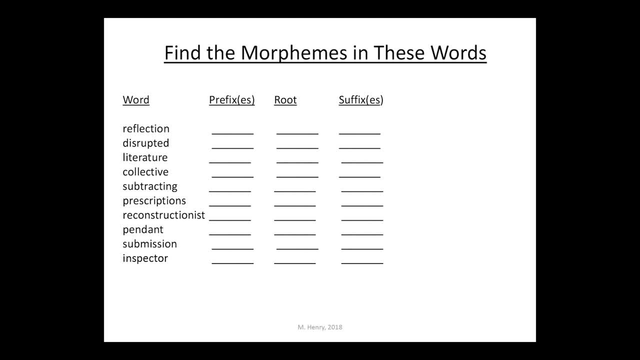 How about the suffix? Now let me talk about shun, T-I-O-N, S-I-O-N and C-I-A-N. When do we use C-I-A-N? Can you think of any words with C-I-A-N? 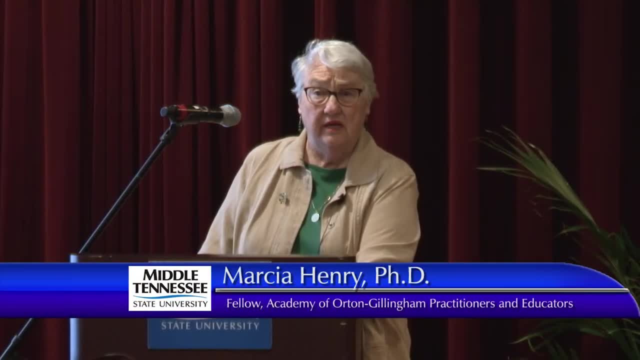 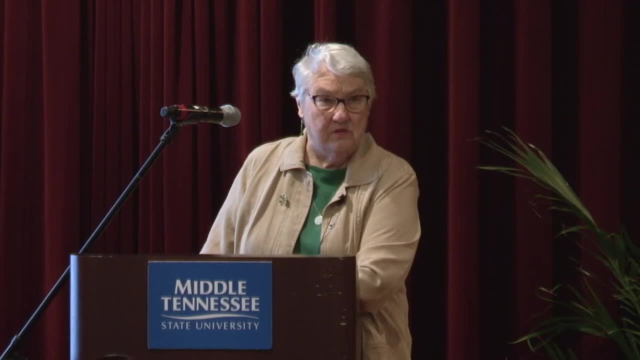 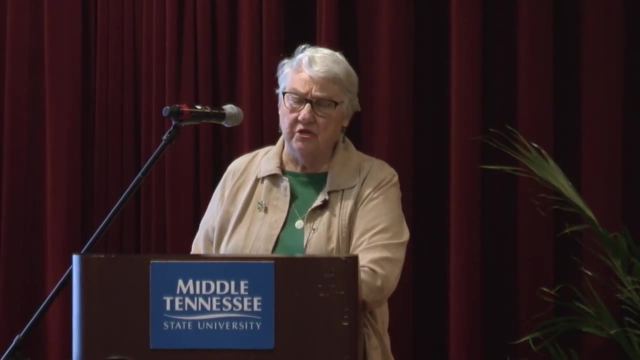 Mathematician, electrician, statistician, physician- They're all people. They're all noun people. So when we have a noun person- musician, magician- then we use C-I-A-N. Otherwise we tend to use T-I-O-N. 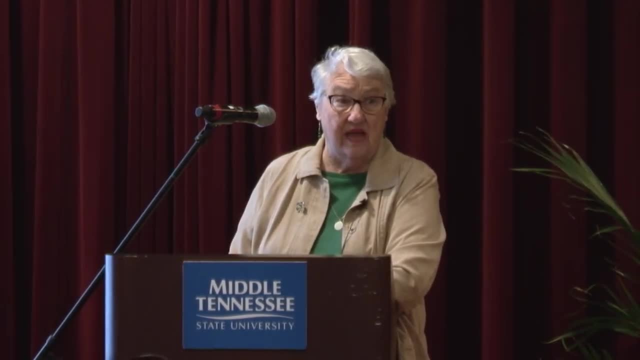 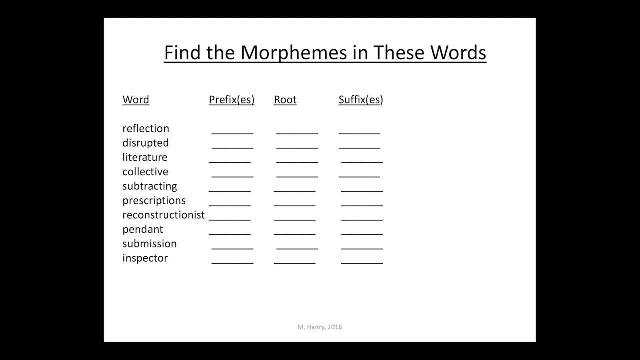 sometimes S-I-O-N, especially if the root ends in a S like accession. Technically, the root is only I-O-N, It's not shun, It's not T-I-O-N, But two different things happen If I'm asking a child to divide this into syllables. 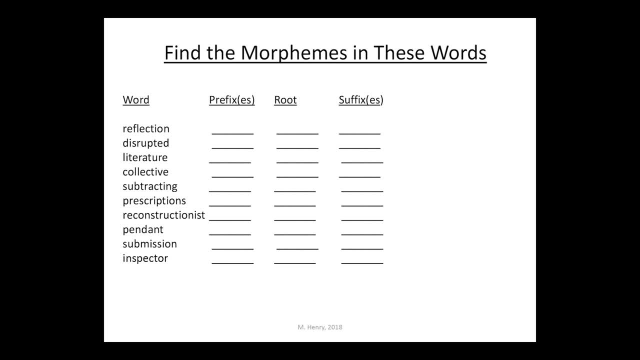 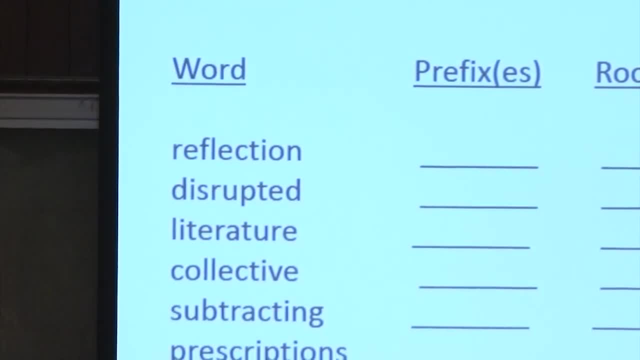 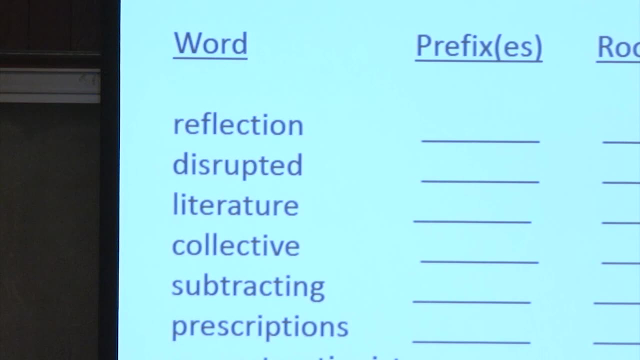 where am I going to divide? first, Re-flec-tion, right Between the C and the T. But if I'm asking them to identify morphemes, I have re-flec-t and I-O-N. I would give credit for suffixes. 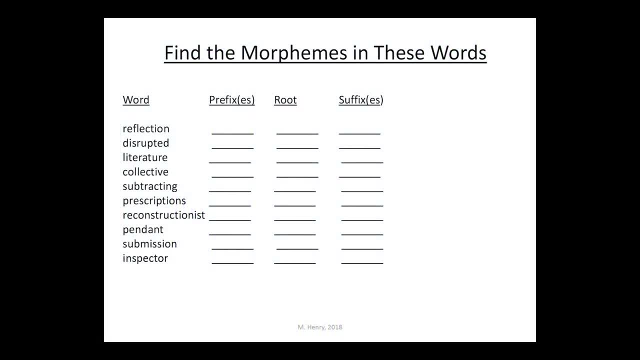 if they put T-I-O-N, but I want you all to know that it's I-O-N is the suffix. How about the prefix in disrupted Yes Root Suffix? How about the prefix in literature? There isn't one, is there? 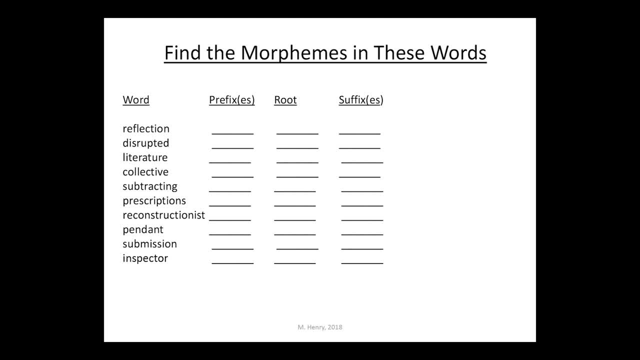 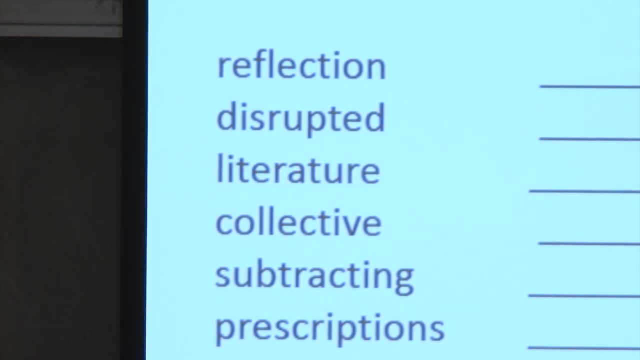 Good, And the root is litter or littera. It's really littera, And then we've added eight. She's literate. Then we drop an E and we add U-R-E literature. So it would be Technically. I actually have two suffixes there. 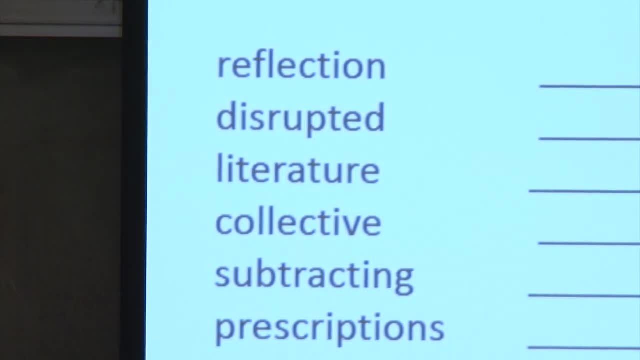 I have the root litter, I have a suffix eight and then I cross off the E and I have a suffix U-R-E. How about collective? What's the prefix? Col C-O-L, The root Lect And the suffix. 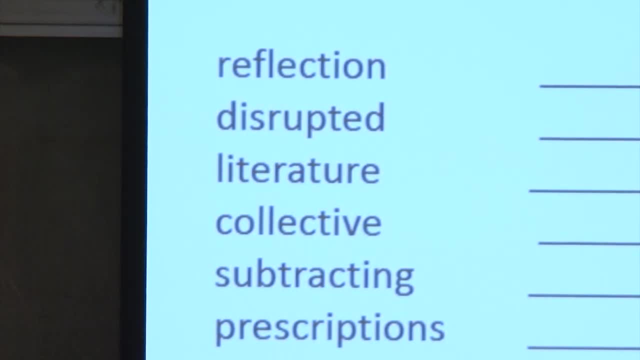 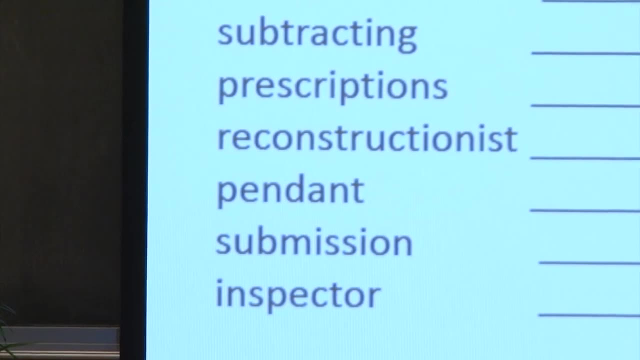 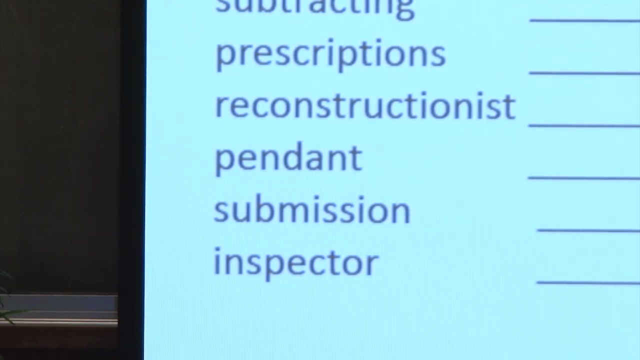 Subtract: Okay, Subtracting Subtract Prescriptions, Prescriptions I-O-N and S right. How about reconstructionist Prefixes, Prefixes Root, Subtract Suffixes, Suffixes Good, I-O-N and I-S-T? 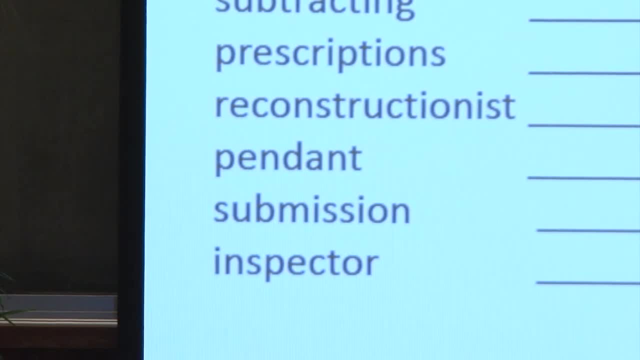 How about pendant? What's the root Pend? I mean there's no prefix. Pend is the root meaning to hang A pendant hangs, And the suffix The N-T, A-N-T. Submission Subtract I-O-N. 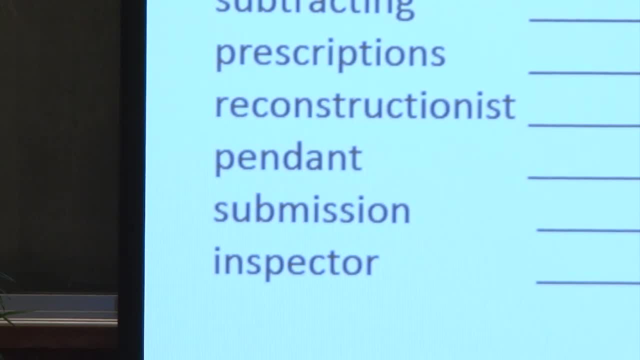 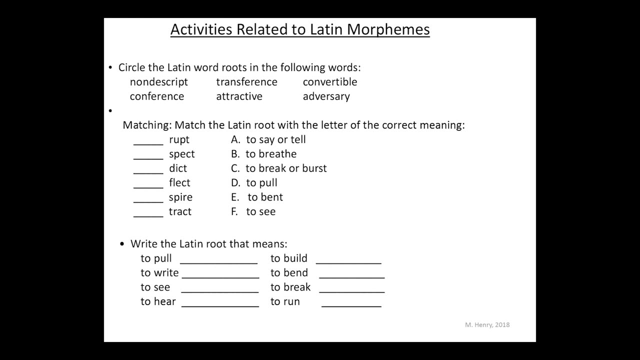 I-O-N good Inspector, Inspector, Okay, What are kinds of exercises that you can do with your kids? You can have them circle. Latin root in the following words: I know you've just had a glance at those roots, but what's the root in the first word? 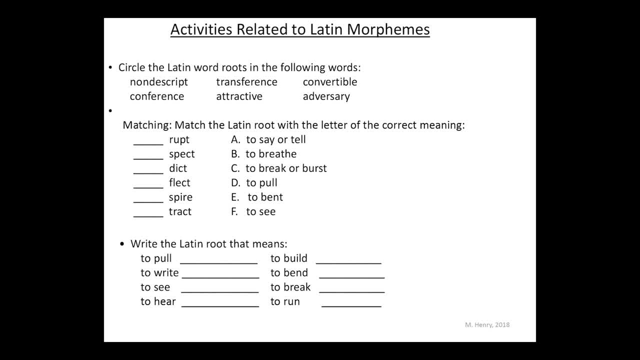 Script, Script. How about the root? in the second one? It's fur, Fur, Fur. How about in convertible Vert, Vert to turn: Conference, Conference, Conference, Attractive, Attractive, Adversary, Adversary. 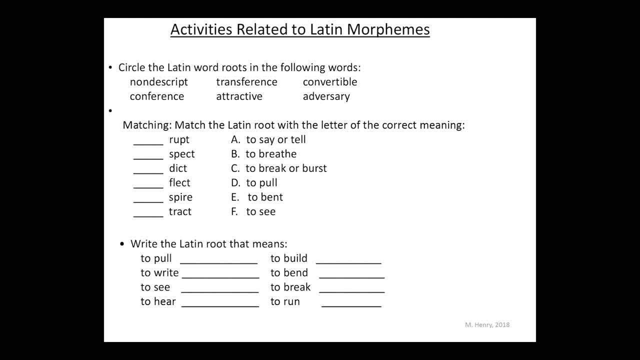 Adversary, Adversary, Adversary, Adversary, Adversary, Good. Okay, what does rupt mean? To break, To break or to burst? Do you rupture your appendix? It bursts. How about spect? 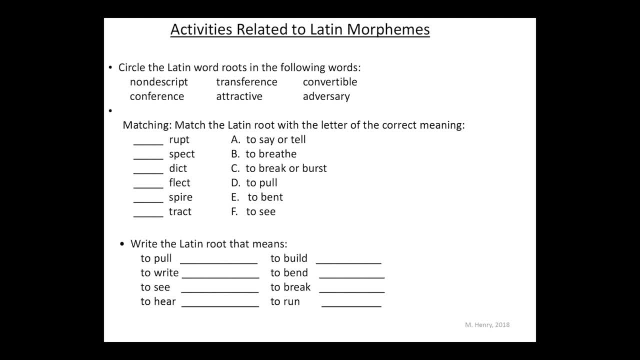 Okay, How about dict, Dict, noises, Flect, Flex, Flex, bend be bent Flex. How about spire To breathe like respiration Tract To pull Tractor: Attractive, you're pulled toward something. 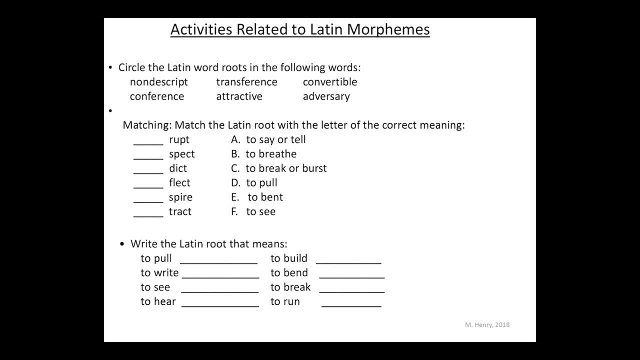 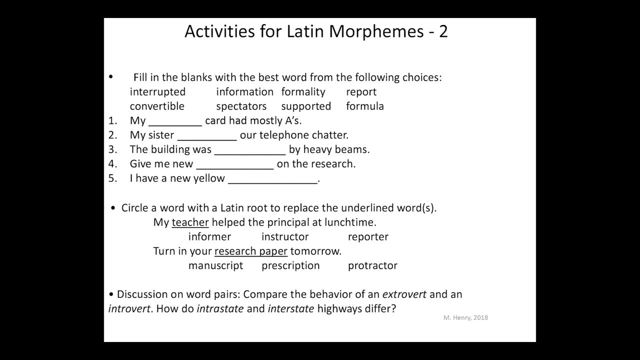 Write the Latin words that mean to pull. That would be tract. You can just see the type of exercise I won't test you on that. Fill in the blanks with the best word from the following choices: So it would be what My report card had, mostly A's. 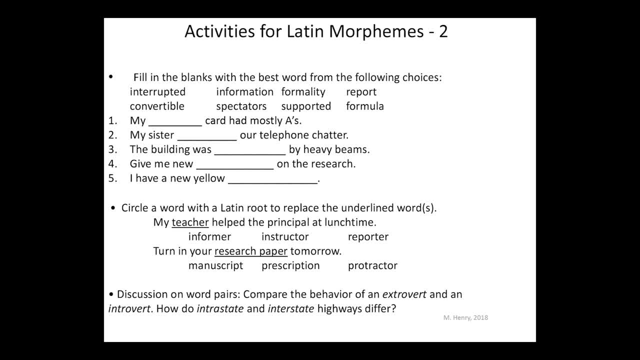 My sister interrupted our telephone chatter, The building was supported, and so on. Circle a word with a Latin root to replace the underlying word or words. My teacher helped the principal at lunchtime. What word means the same as teacher? Okay, how about turn in your research paper? 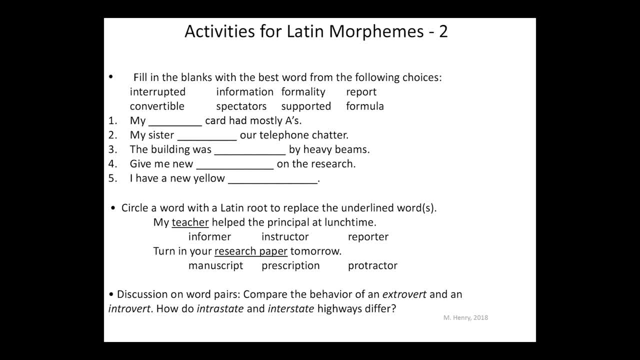 your manuscript. Discuss word pairs, Compare the behavior of an extrovert and an introvert. Vert means to turn, An introvert turns where Inward an extrovert outward. The payoff for teaching morphemes is that not only are these patterns for decoding, 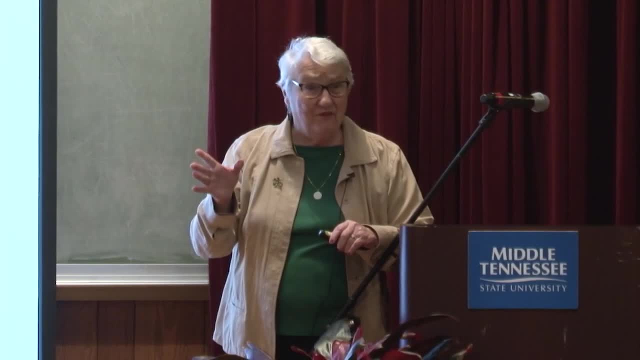 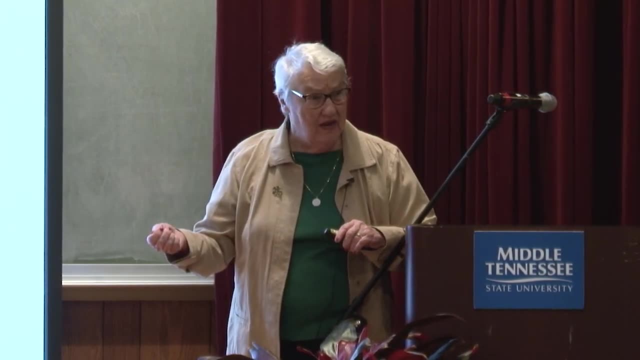 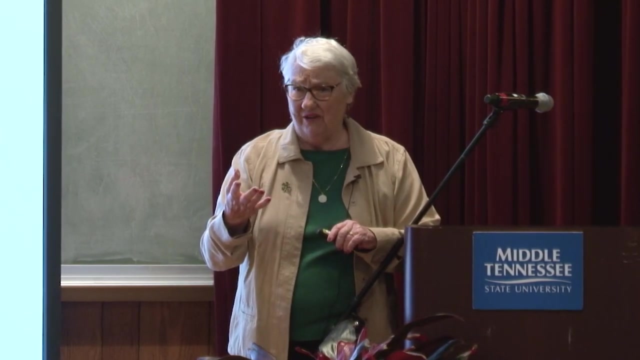 and for spelling. but for what? For vocabulary, And what has the highest correlation with comprehension: Vocabulary. So you get triple at least payoff teaching these morphemes. And yet teachers many times are hesitant to do it. I've had teachers say 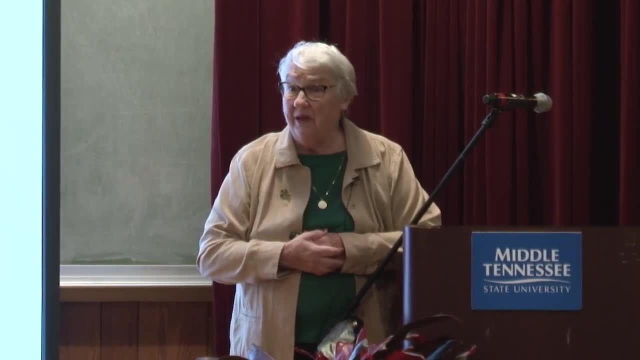 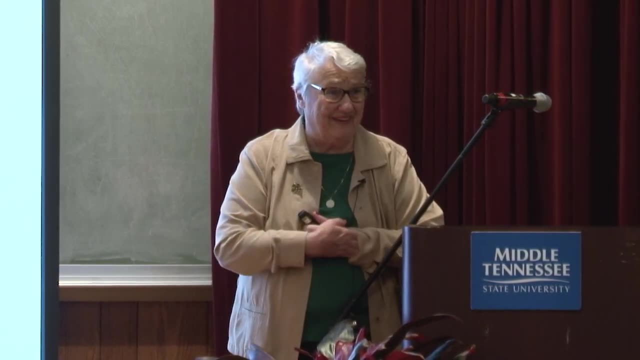 but I never had Latin in high school- Well, most people haven't- Or Greek. I don't know of anybody. I don't know of anybody who had Greek, but maybe somebody did. But these are the kinds of things that you can do. 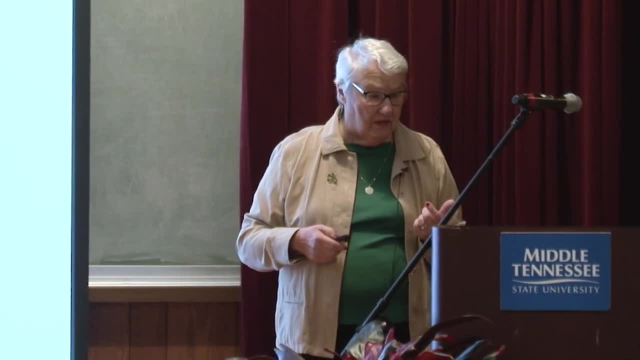 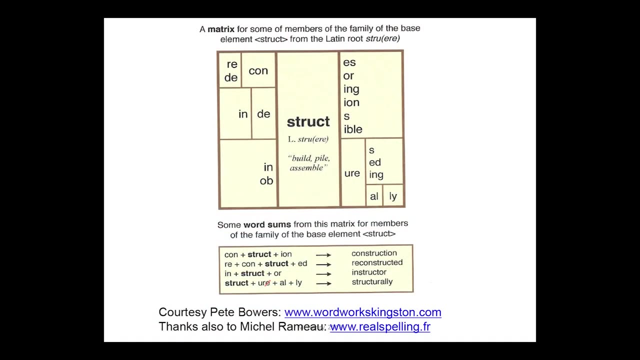 that enhance vocabulary, decoding, spelling, fluency and then therefore comprehension. Now here's from Pete Bowers and Michelle Ramoux. This is his, this real spelling. that's the right website. Here he's done. 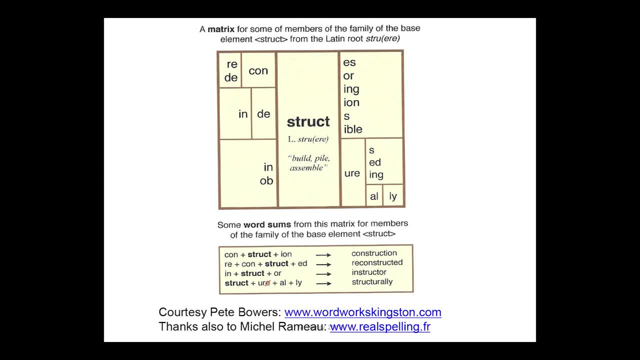 he's done one of those word matrices. with struct I can do re or deconstruct and so on. The es shouldn't be there, That es. if you've got handouts, cross that out. He also does what's called word subs. 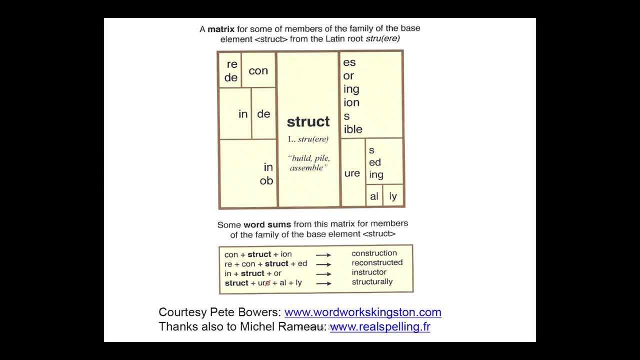 showing how you add those parts together: Con plus struct plus IOB Plus ION, Re plus con plus struct plus ed, In plus struct plus er, and so on. These are just fun activities that the kids kind of like doing in groups. 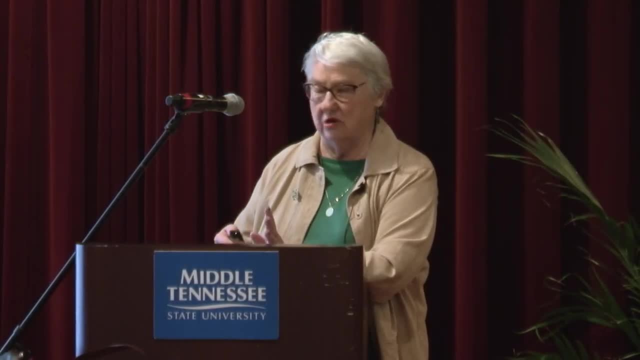 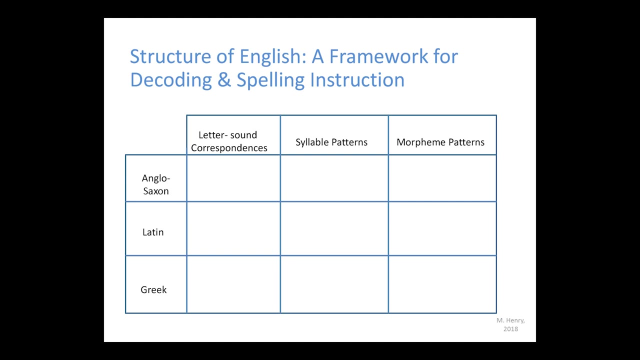 and it helps them to then be aware of the structure of the language. Okay, so here's our three by three matrix. again, We've gone through the Anglo-Saxon letter-sound correspondence. There's the syllable patterns, the morpheme patterns. 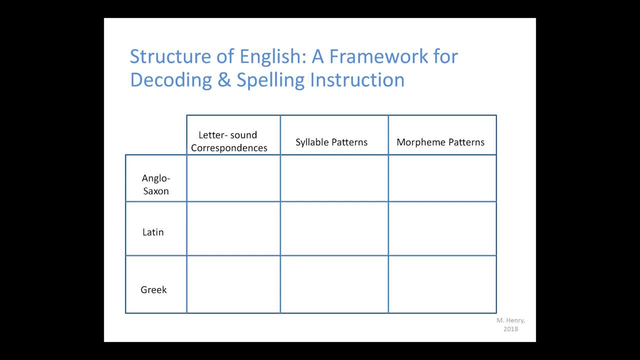 With the morphemes we learned that we both compound and affix. With the Latin we know that the letter-sound correspondences are the same as Anglo-Saxon. There are fewer digraphs. The syllable patterns are similar. The morpheme patterns we generally affix. 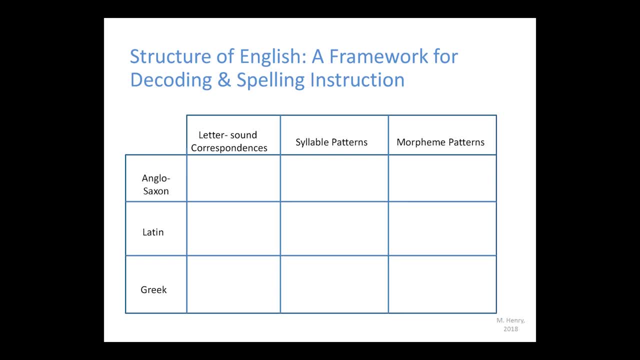 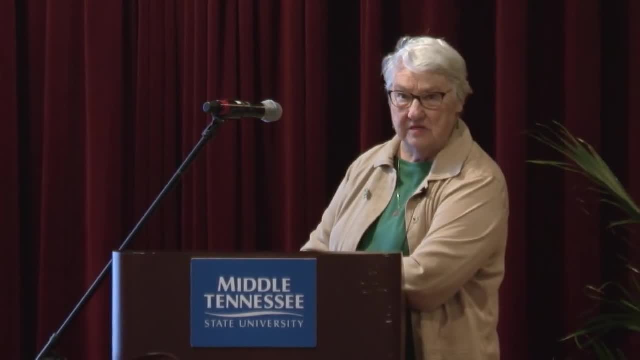 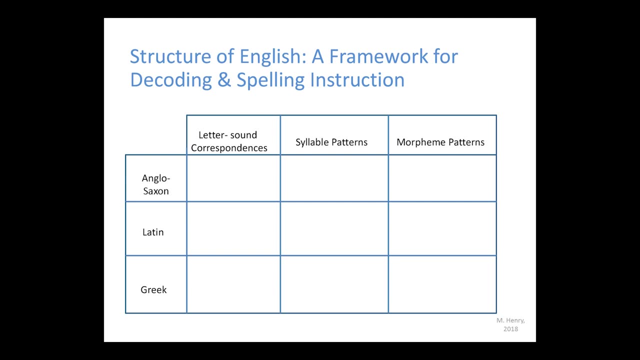 rather than compound. Now we're gonna move on to Greek Greece And we do have to learn some new letter-sound correspondences with the Greek, And syllable patterns will remain pretty much the same And the morpheme patterns will compound generally. 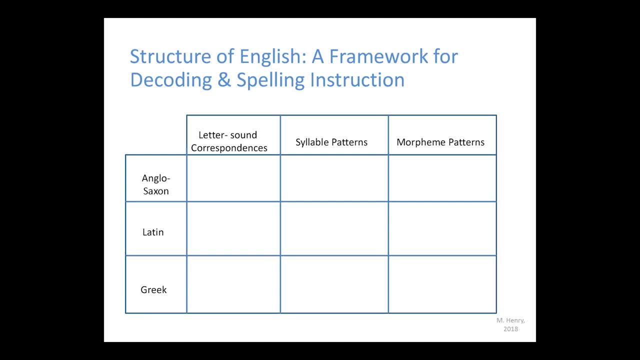 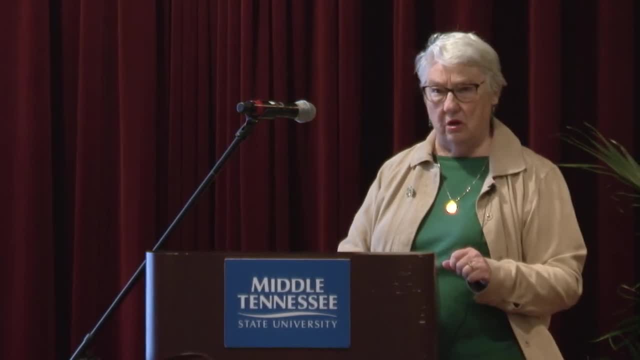 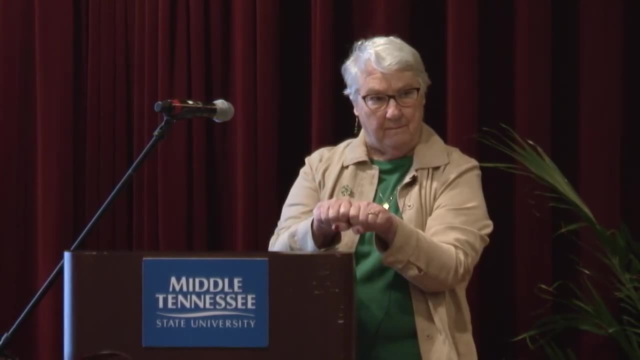 We can also add suffixes. but generally what happens- and these are linguists call the Greek roots combining forms, because we combine them And the Greek roots, the Greek roots, we combine them, we compound them. Now this is a fifth grade paragraph. 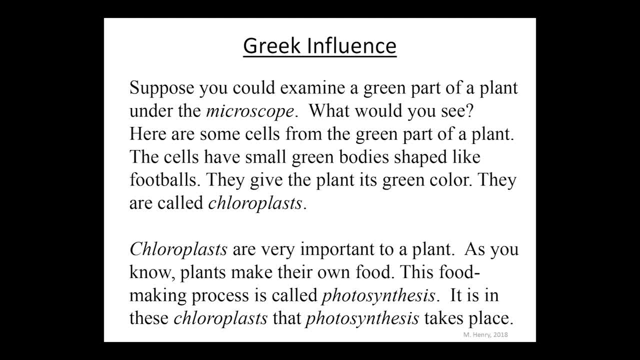 Suppose you could examine a green part of a plant under the microscope. What would you see? Here are some cells, and then there's a picture of cells From the green part of a plant. the cells have small green bodies shaped like footballs. 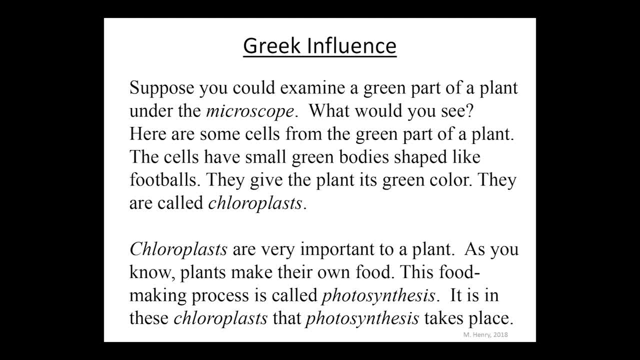 They give the plant its green color. They are called chloroplasts. Chloroplasts are very important to a plant. As you know, plants make their own food. This food-making process is called photosynthesis. It is in these chloroplasts that photosynthesis takes place. 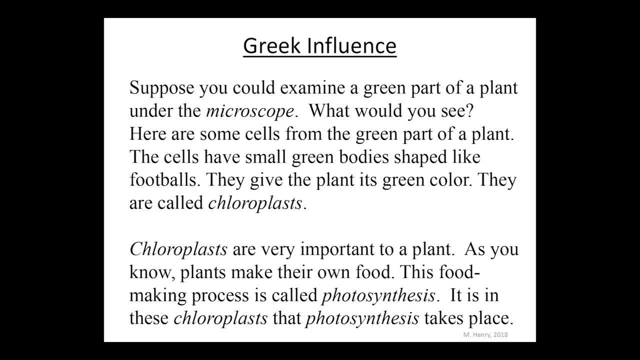 Now, if you analyze these two paragraphs, how would you characterize most of the words in terms of the language of origin? They're Anglo-Saxon, aren't most of them? Little words, You could a green part of a plant under the 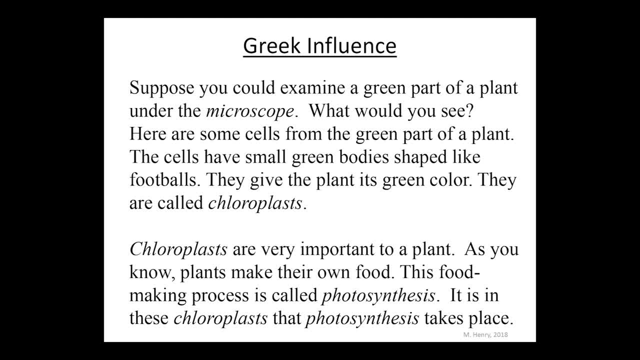 what would you see? Here are some from the green part of a plant. The have small green bodies shaped like footballs. They give the plant its green color. They are called: What are the scientific words? What are the words that in the context? 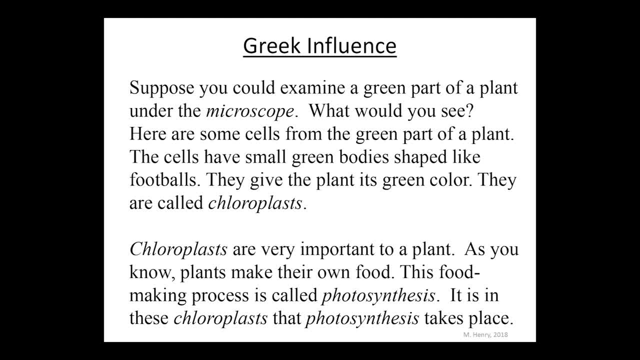 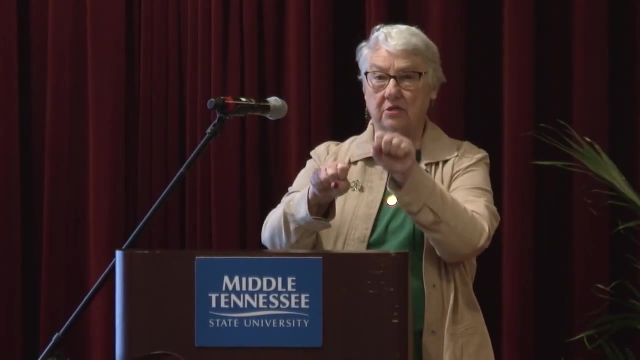 are so content-specific to science. Those are the Greek words And, like chloroplasts, chloroplasts, microscope and photosynthesis. Now notice microscope. I'm combining two, combining forms, two roots: Microscope. Micro meaning very small. 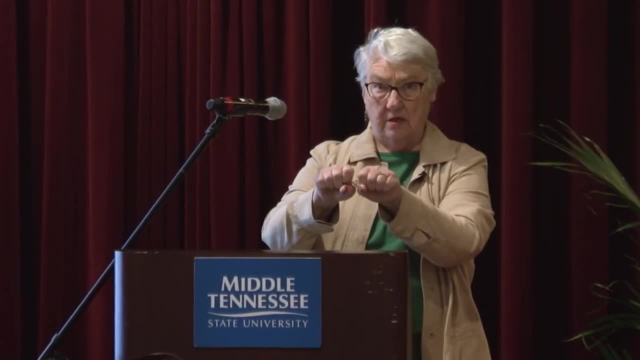 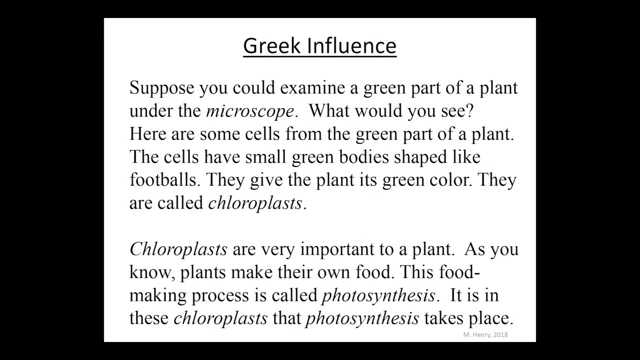 Scope, meaning to see or look. So I'm combining those And there are no different unique Greek letter. sound correspondence in that. But look at chloroplasts. I'm combining again Chloro, chlor plus what we call a connective o plast. 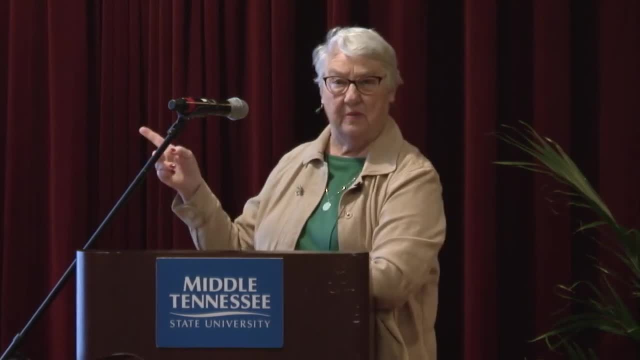 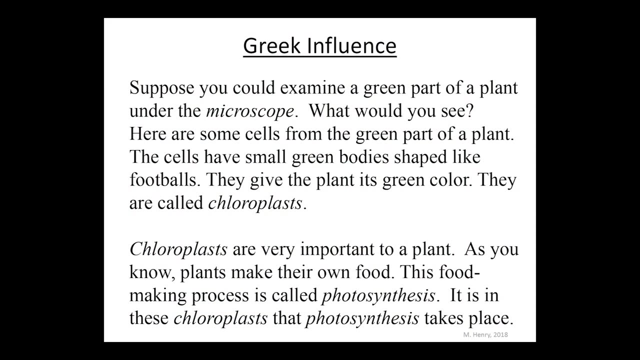 What's uniquely Greek in terms of letter sound correspondence with chloroplasts, The C-H saying k. In Anglo-Saxon the C-H says what Chesh? If it's a French Latinate word, what does the C-H say? 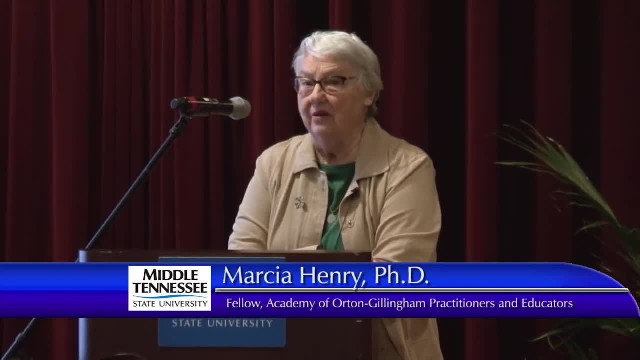 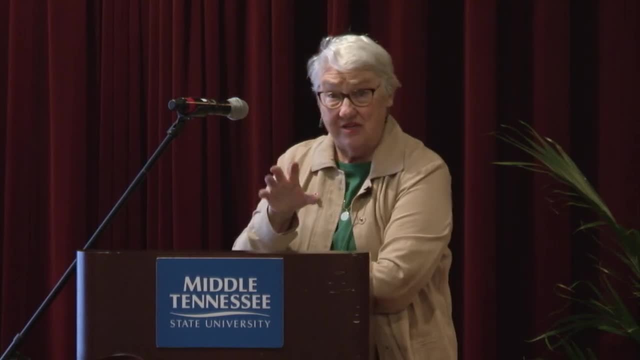 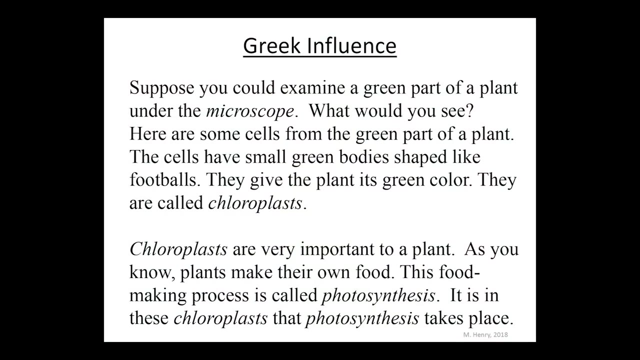 Sh like champagne or chef or mustache. okay, So the C-H can end up being one of three different sounds. How about photosynthesis? What's uniquely Greek letter sound correspondence in that word, Ph, The P-H saying ph and the Y as a short? I is very similar. 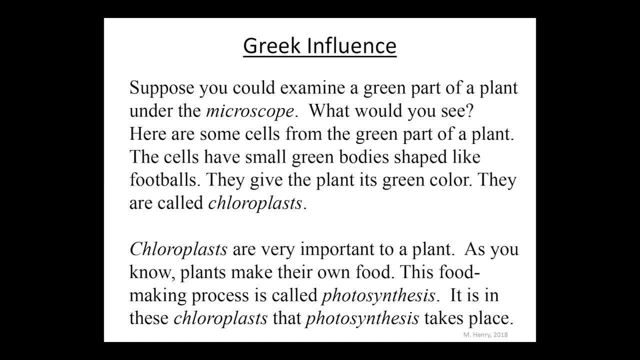 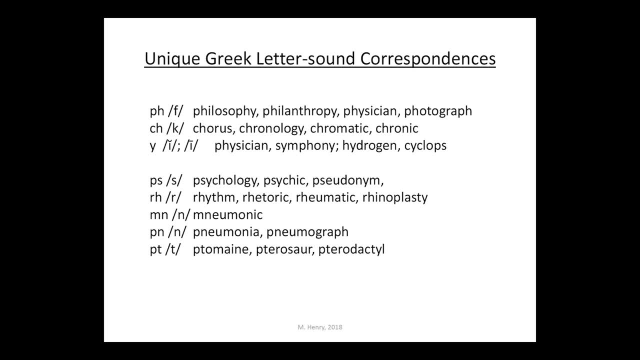 Very common. So those are the main changes. We have some very rare letter sound correspondences like M-N in mnemonics, P-N in pneumonia, and so on, R-H as in rhinoceros. those are all Greek. 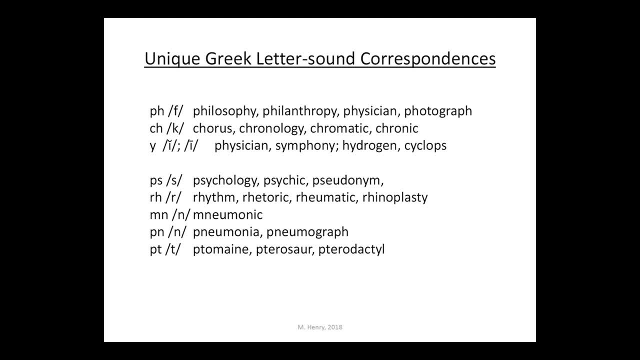 Yeah, I've got a list of those here for you. The three main ones, the P-H, C-H and the Y, is either an I, short I or ph I, or a long I, as in hydrogen cyclops, as an open syllable. 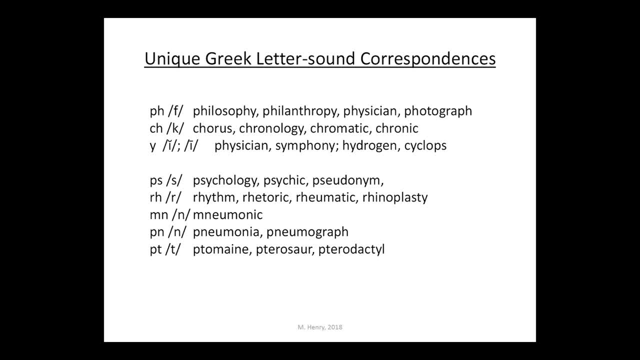 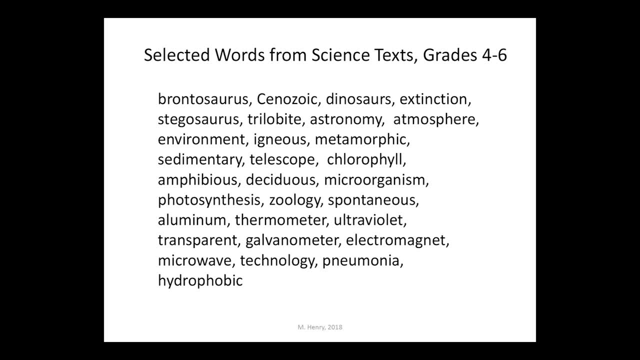 And then the less common, the P-S, the R-H, M-N, P-N and P-T. Look at the science text here: Brontosaurus, Cenozoic Dinosaurs, Extinctions, Stegosaurus, Trilobite, Astronomy. 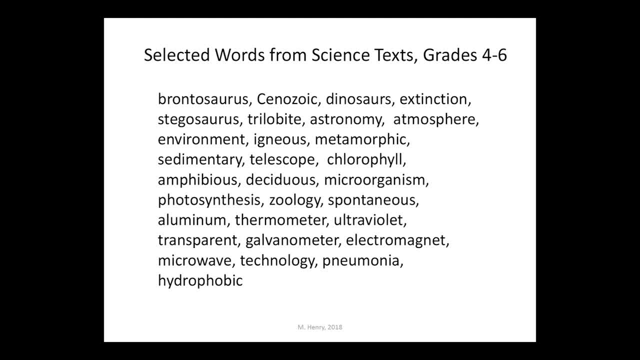 and Atmosphere, Environment, Ignis- Again, grades four through six. So it would be helpful. It would be helpful to have some opportunity to think about some of these roots, learn some of them. Here's the roots that I teach. 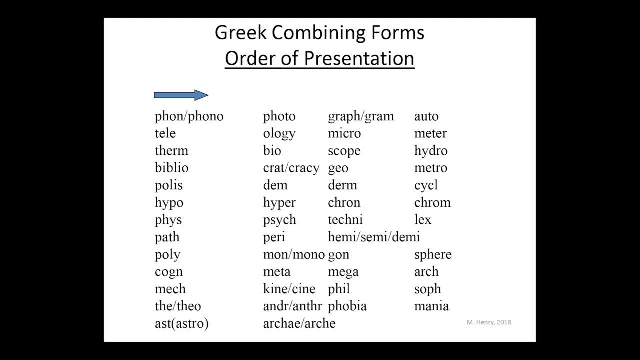 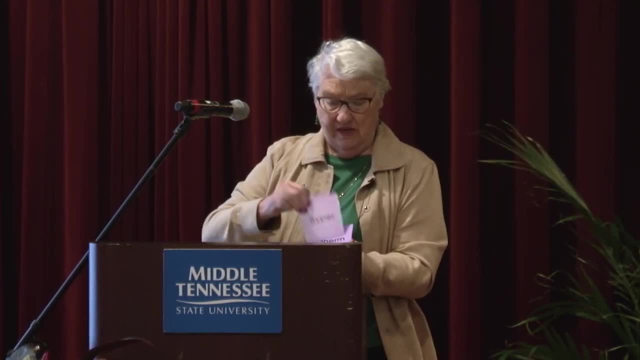 going left to right in the order And of course, you have to connect it with its meaning. So make some cards and you'll want the kids, your students, to know the meanings of all of these and you'll want these to just be. oh, they're so beautiful. 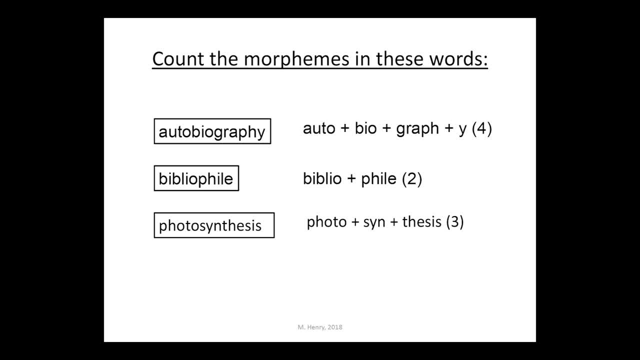 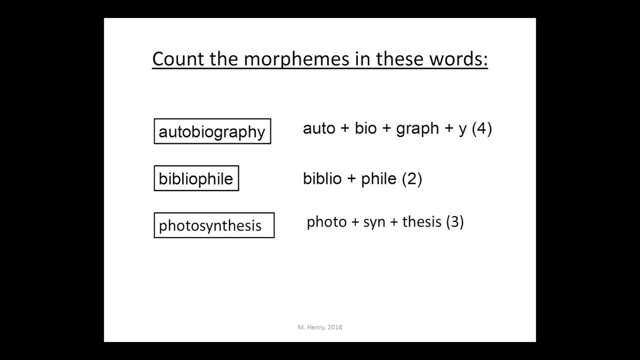 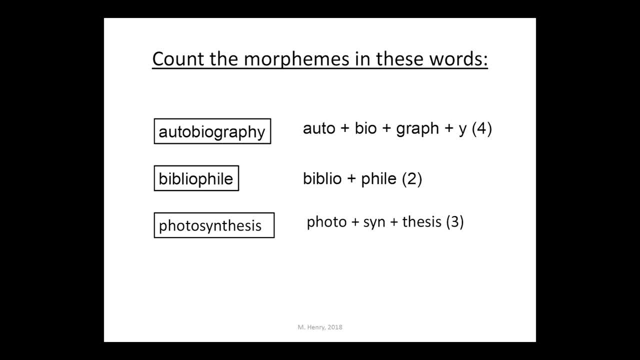 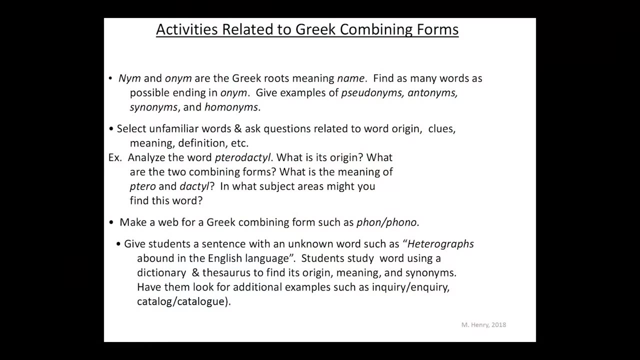 What is phile? A love of books. Phile is love, like in Philadelphia, the city of brotherly love. Okay, And a lot of snow a little bit ago. Activities that are related, like in and onium, are the Greek roots. 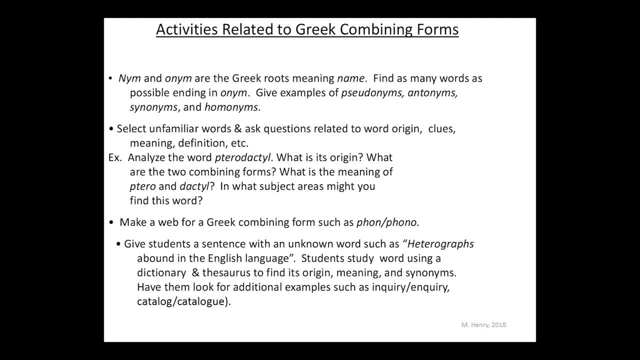 meaning name. find as many words as possible, So you have pseudonyms, antonyms, synonyms, homonyms, select unfamiliar words and ask questions related to word origin clues, meaning and definition. Analyze the word pterodactyl. 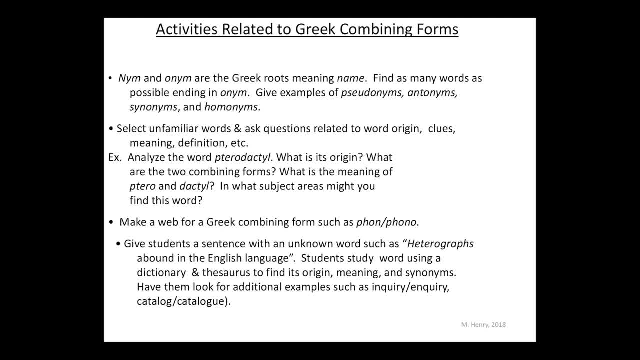 We kind of did that. What is its origin? What are the two combining forms? What's the meaning of pterodactyl? In what subject areas might you find this word? Make a web phone and phono? Give students a sentence with an unknown word? 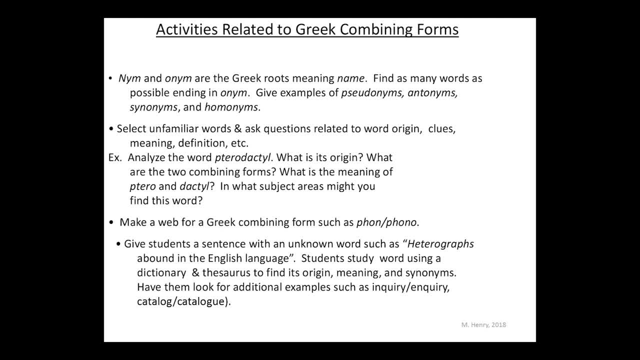 such as heterographs abound in the English language. Students study word using a dictionary, a thesaurus. find its origin, meaning synonyms. Have them look for additional examples such as inquiry, enquiry, catalog and catalog. So a heterograph can be spelled more than one way right. 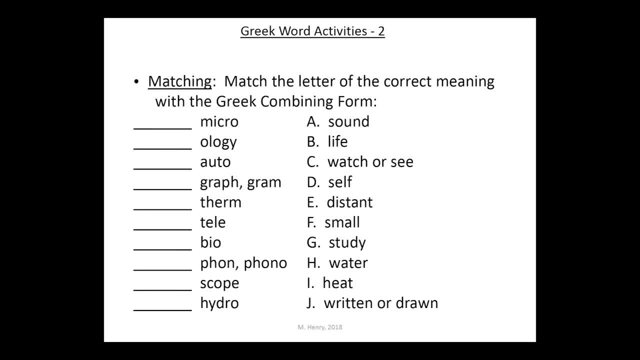 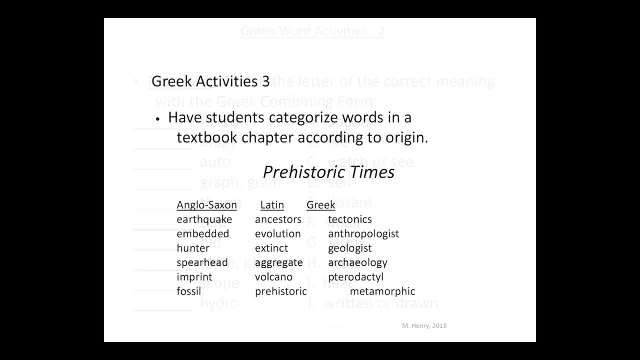 It's okay to spell inquiry with an I or an E. Again, we have our math. They have seen English and they can figure that out. viu-e-nive-ous-couch-ing type of thing, You can figure that out. 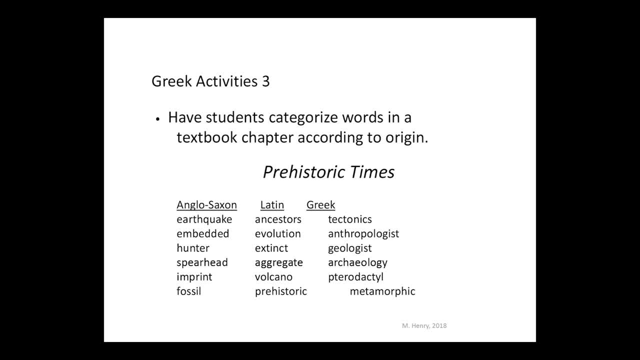 Have a student categorize words in a textbook chapter, so that one of my students did this one on prehistoric times. Some of the Anglo-Saxon words, some of the Latin-based words and some of the Greek-based words Count the morphemes and syllables. 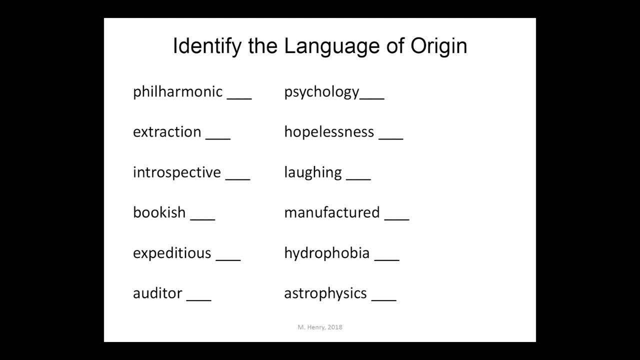 Well, we've done that a lot. ��릴게요 couple minutes. what's the language of origin in philharmonic? how do you know that you've got that clue right there, don't you? uh the ph? how about psychology greek? why the ps? yep, uh, extraction. 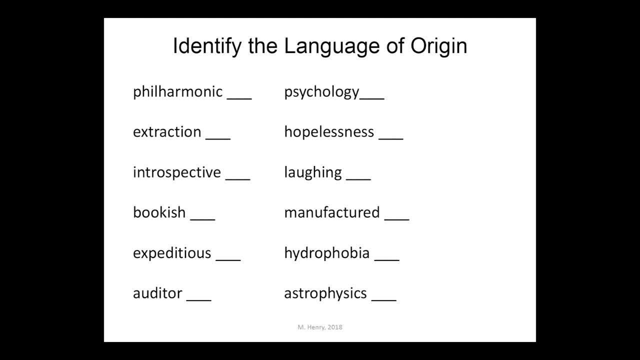 latin. right, i've got a nice strong uh root tract and i'm adding my prefixes and suffixes: hopelessness, anglo-saxon, i have hope. and then less and less introspective. good laughing, bookish, manufactured latin. good, expeditious latin, hydrophobia, um, what does it mean? 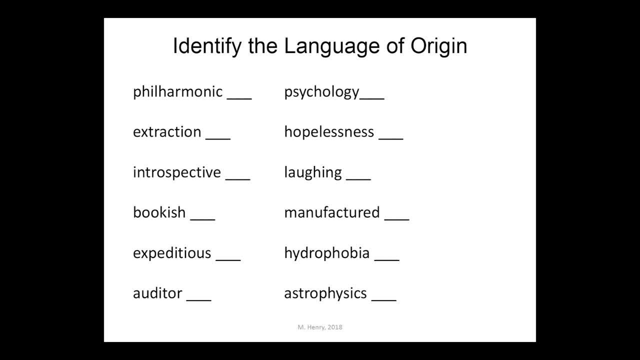 a fear of water. right, hydro is water, phobia is fear, a fear of water. how about, uh, auditor, latin, odd- and astrophysics- greek good, it's a nice come combined formed astro and physics, okay, uh, how many of you have seen akila and the bee, did you love it? 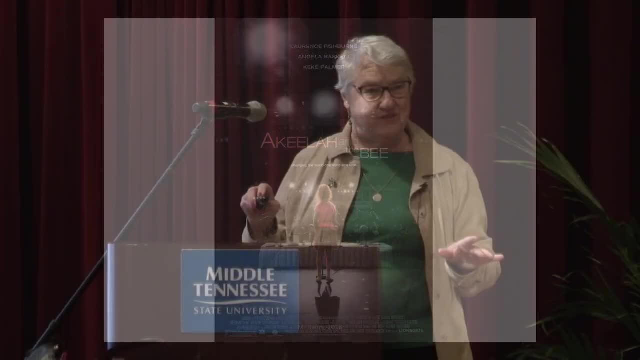 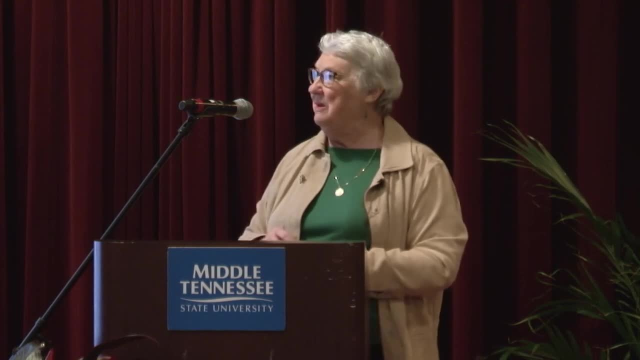 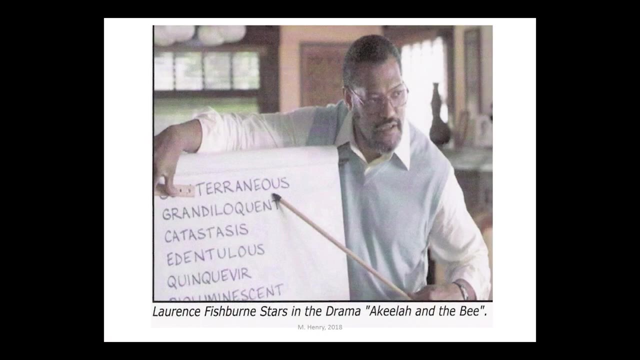 and just to add, i just wanted to see a little thing. i encountered another. you know one of the uh wonderful stories. i guess you'd want to go into the national spelling bee once for a little bit. you need to see a நviet pchenileri. 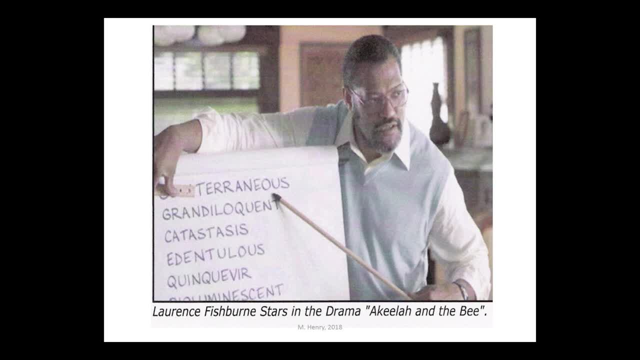 if you haven't seen it is that a wonderful story about a young woman, eighth grader, who wants to be in the national spelling bee, and Laurence Fishburne, who i adore, is her professor and he's from UCLA, and he shows her this word He said: well, what does solar mean? 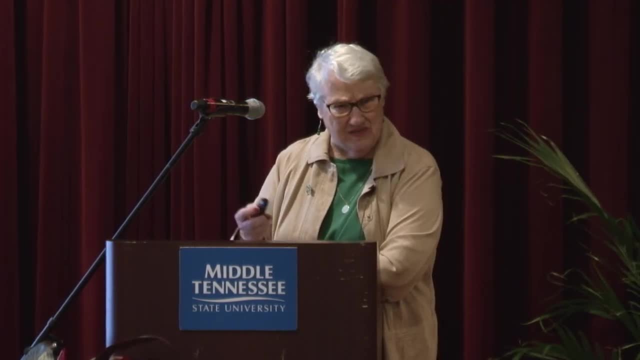 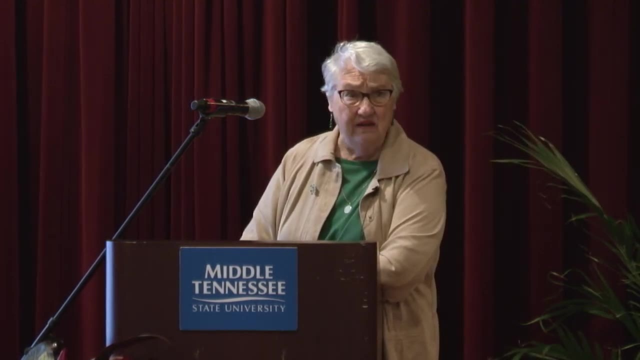 What does it make you think of? Well, she said solar, And he said well, what does that mean? Well, the sun. Do you recognize any other word part? Well, terrain, Yes, of course. What do you think terrain is? 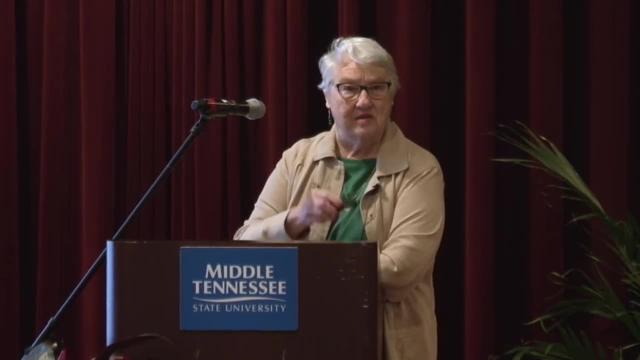 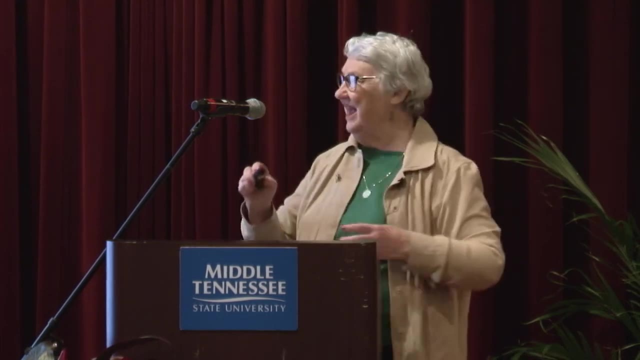 Well, it's the earth. Well, yes, that's right, It's the sun and the earth working together to provide energy. And so he takes her through all these words, And here's what he says. He says: where do you think big words come from? 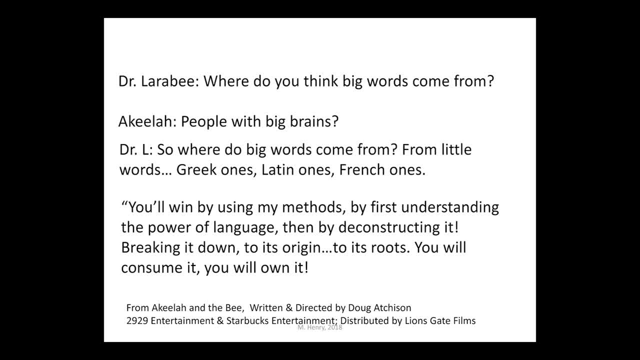 And Akilah says people with big brains. So where do big words come from? From little words, Greek ones, Latin ones, French ones. You'll win by using my methods, by first understanding the power of language, then by deconstructing it, breaking it down to its origin, to its roots. 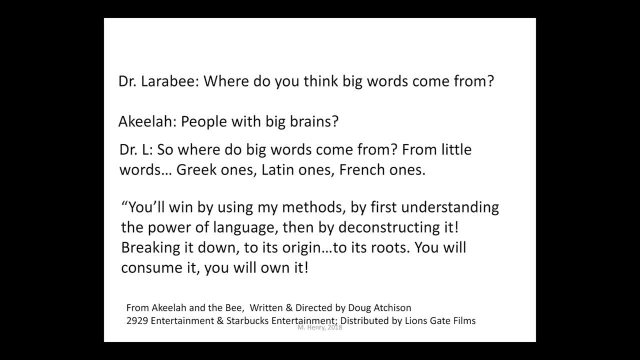 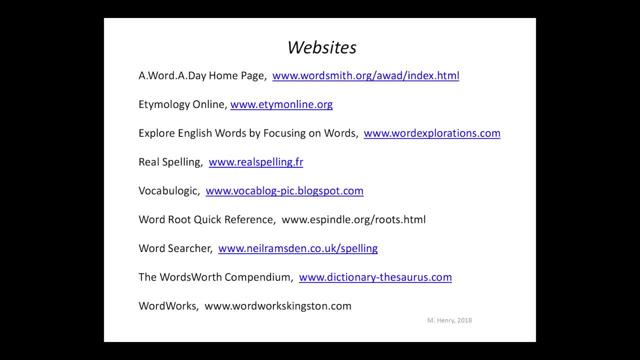 You will consume it. You will own it. I got goosebumps when I saw this. I said yay. Anyway, here are a bunch of websites for you. Etymology Online is a wonderful resource for the origin of words. All of these are really wonderful websites for you. 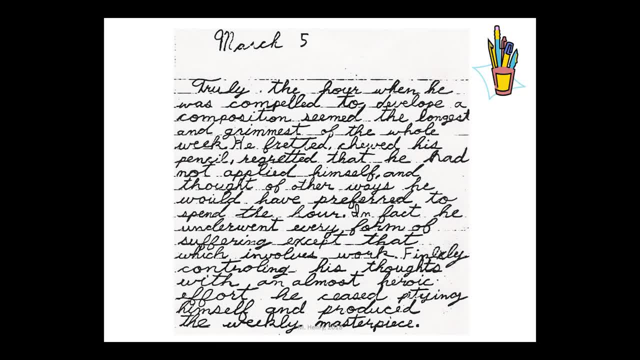 Here's Alan. at the end He's using cursive writing. I tutored him for six months And he just soaked this stuff up Because he was so bright And very atypical. But notice, he's not quite perfect. I mean, he didn't memorize these words that were. 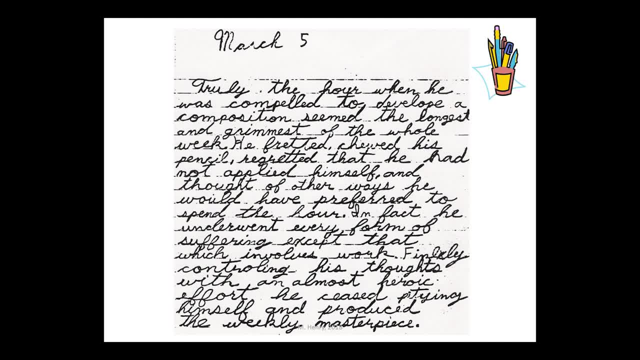 He learned about EST versus IST. He learned the rules of adding suffixes, Why he had to have two Ts in front of it, et cetera. But he's not perfect. He finally is wrong Develop. he has an E in the end.